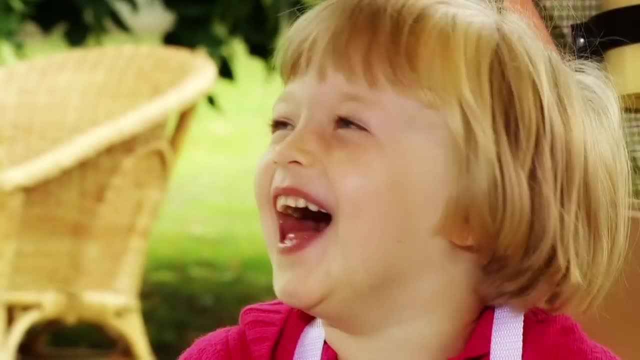 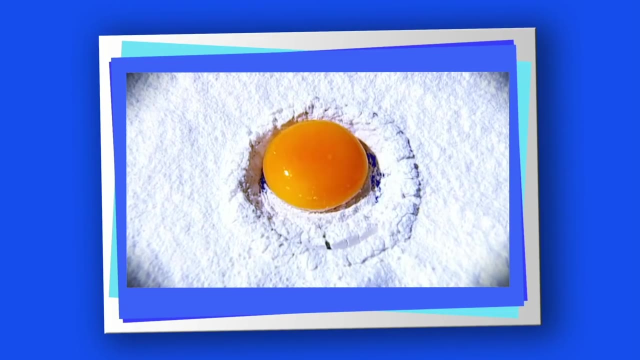 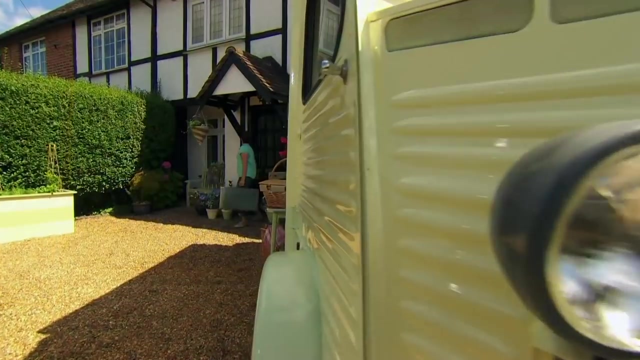 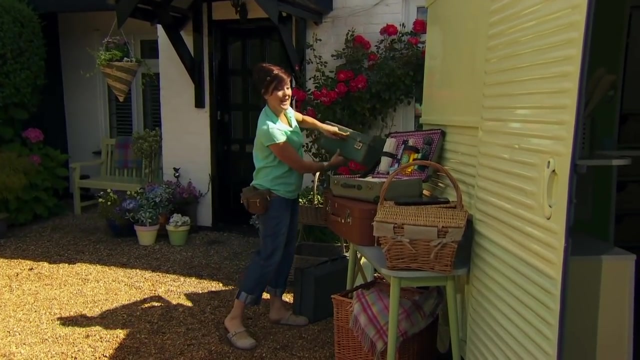 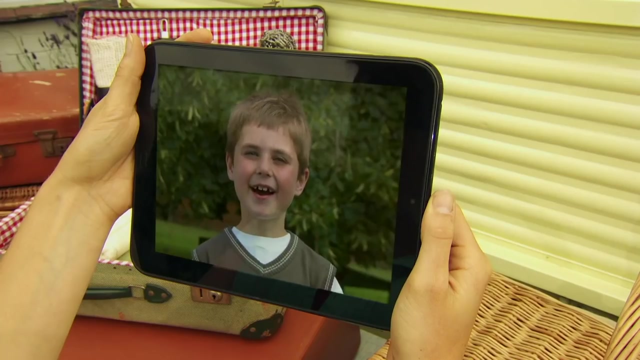 With you. Hello, Oh, great to see you. I'm just getting everything ready to go on a journey and I hope that you're going to come with me and make some new friends. Aha, Hi, Katie, I love bike rides and my favourite fruit is blackcurrants. Oh, that's exciting, Katie. 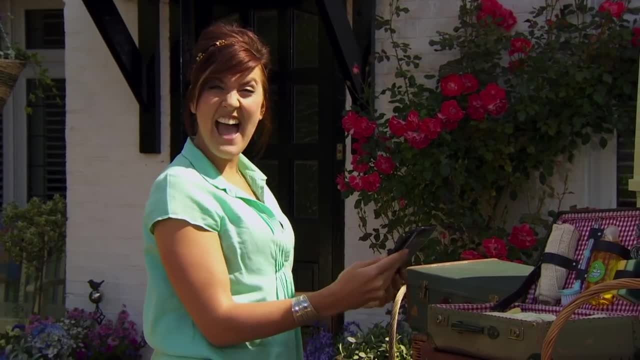 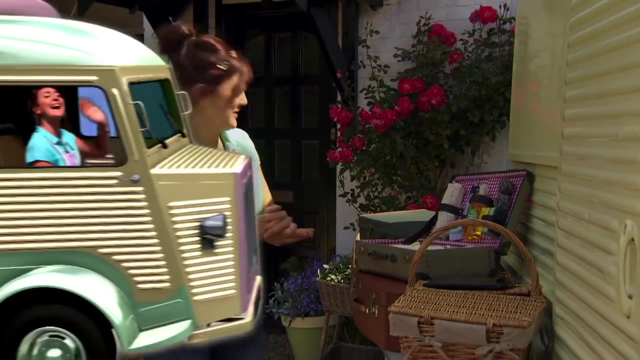 can you cook with me please? I certainly can, Sam, And I love cycling on my bike, and you can cook with me too, So let's pack up and go. I've been on a journey and I'm coming to you. It's going to be busy and it's going to be. 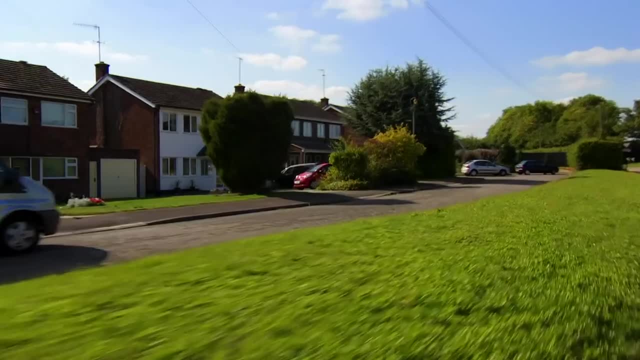 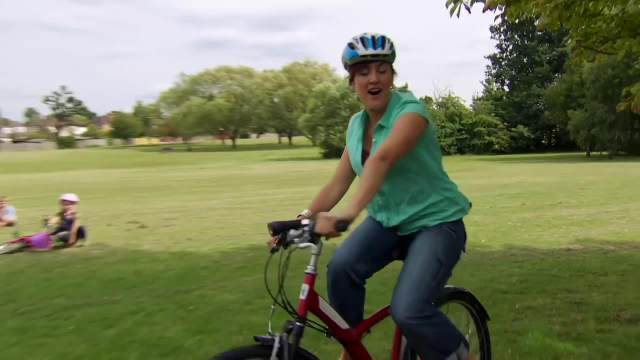 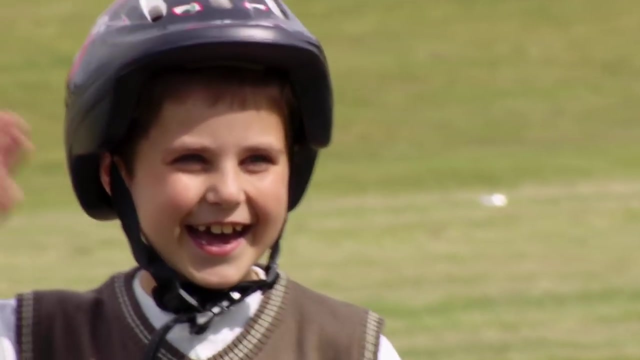 busy and there's lots to do. Get ready to help, Join in and have fun. Let's cook a feast for everyone. Here we are at the park where I've been invited by Sam, And there he is over there with all his friends. Hi, everyone, Hi, Come on over. Oh, it's great to see you. 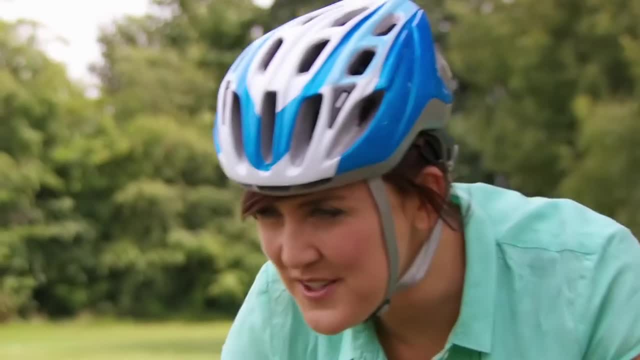 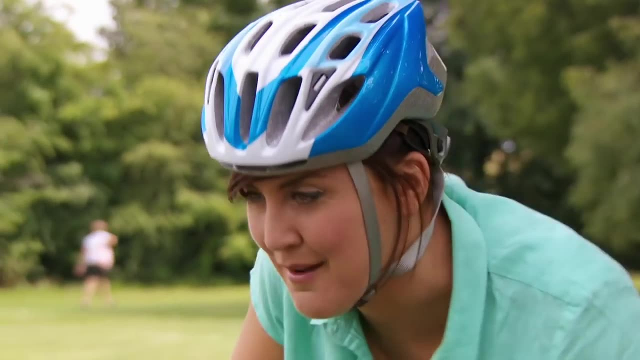 all. So, Sam, are these all your friends? Yes, What are your names? Eddie, Megan, Ria. Oh, that's great to see you, Great to meet you all. Hey, Sam, what are we going to do today? 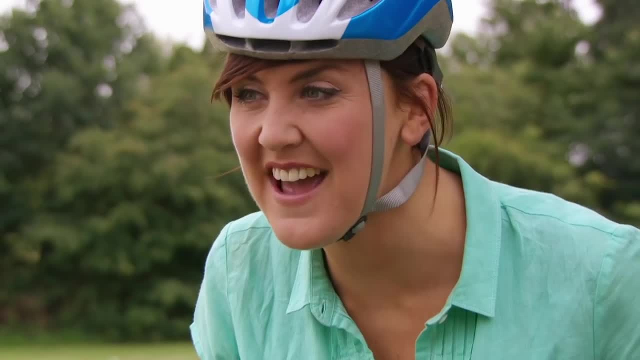 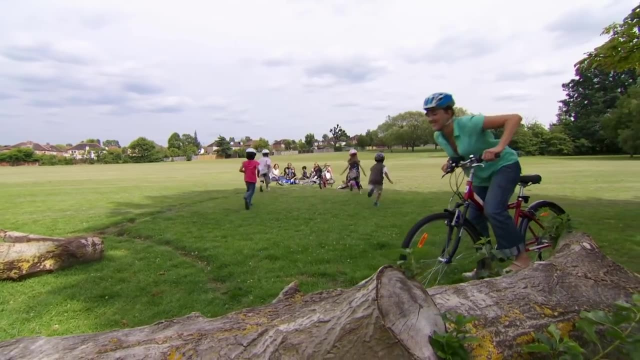 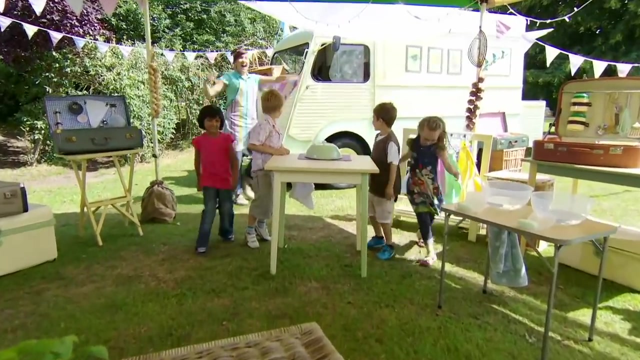 Make some food for our bike ride. I have got such a delicious recipe to make with you all, Why don't you get your bikes and I'll show you what it is? Welcome to my outdoor kitchen, Hey. do you want to know what we're going to cook today? 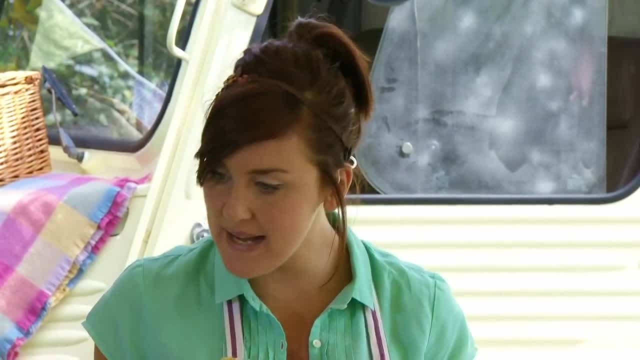 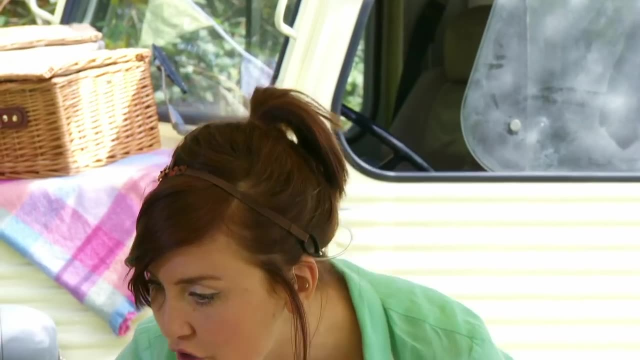 Yeah, Okay. today's recipe is baked blackcurrant rice. Oh, Mmm, Mmm. Before we get started on the cooking, there's something really important that we've got to do first. Does anyone know what it is? Wash our hands. 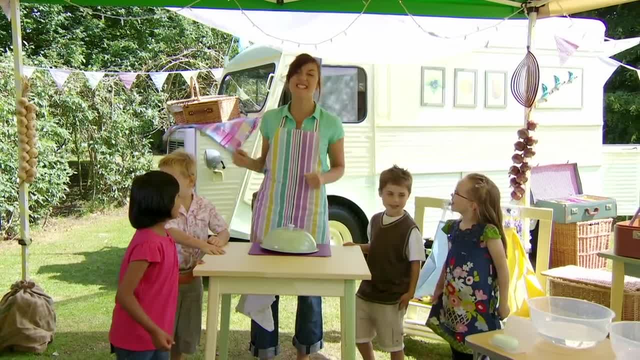 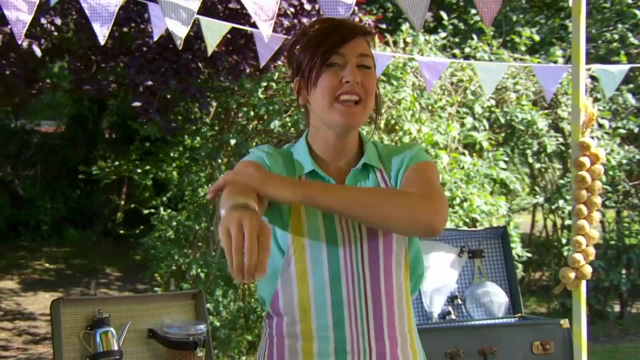 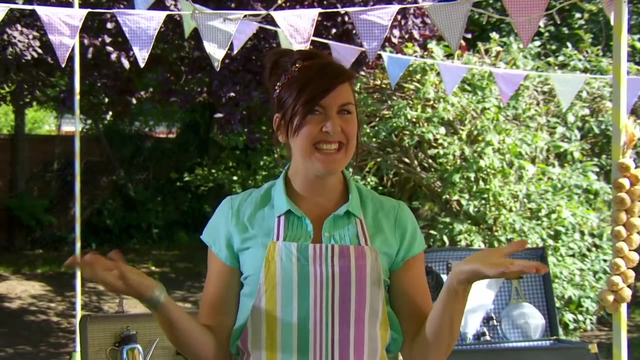 You've got it. We've got to wash our hands, of course. So let's get going. Roll up your sleeves, Give your hands a wash with slippy dippy soap, Splish, splash, blosh. Have you done your hands, Washed and dried? 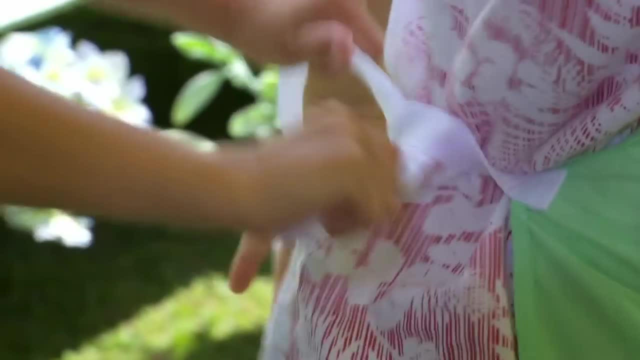 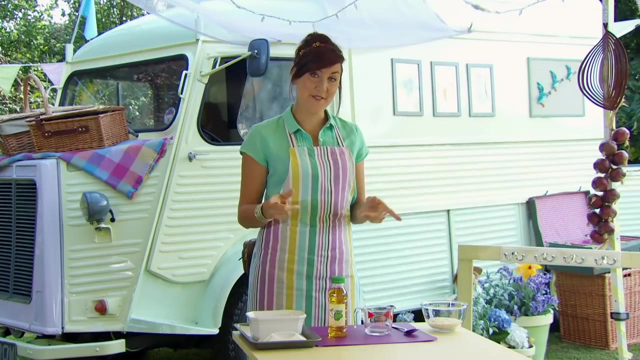 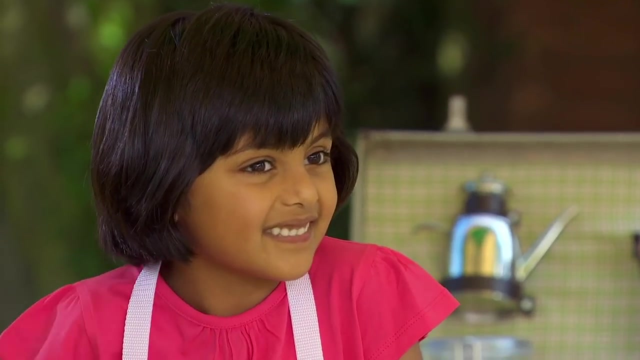 Sleeves rolled up, Apron tied. What can you do? I can cook. Let's get started Now. the first thing we need for our baked blackcurrant rice is apple juice. How do you normally get juice out of fruit? 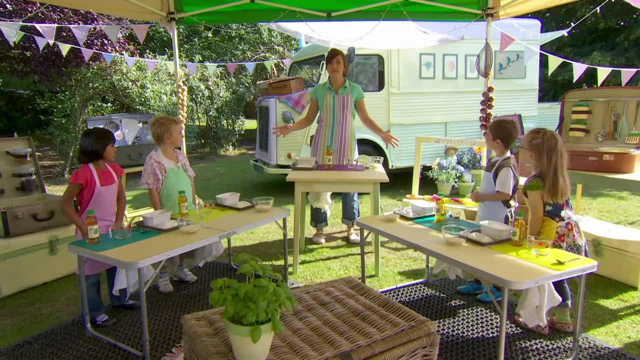 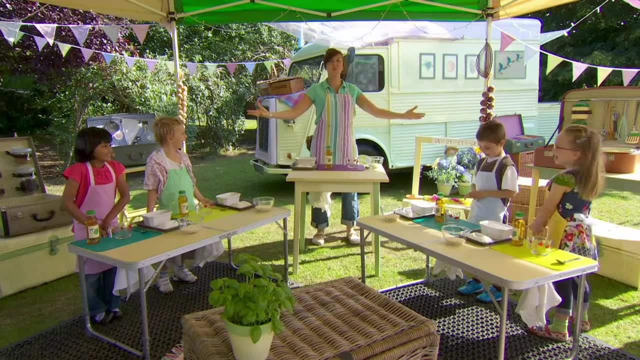 You squeeze it Like this. you mean Squeeze? Yeah, Well, go on then. What are you going to do? Squeeze? Well, go on then. Why don't you squeeze with me? You can join in too Ready. 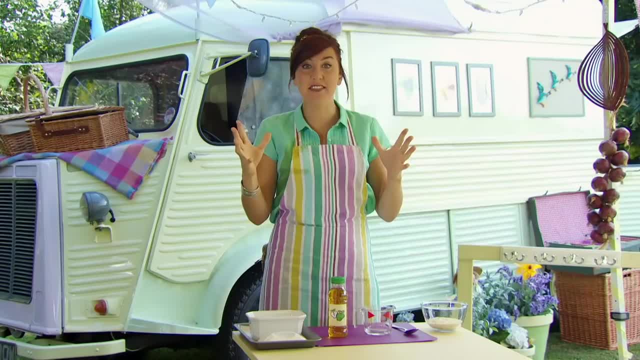 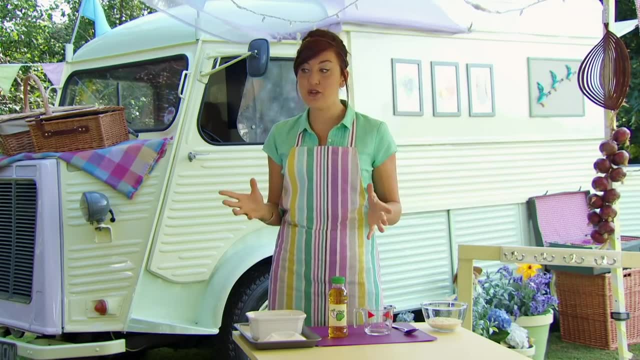 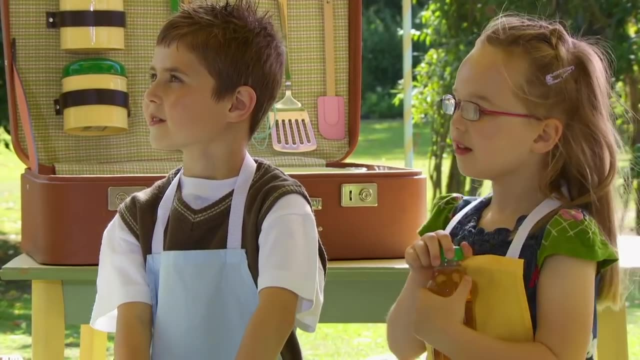 Squeeze, And when you've done that, you get lovely juice, just like this apple juice that we've got here in a bottle. So we need to measure it and to do that we need to work in pairs. One person's going to be the pourer and the other person is going to be the watcher. Now 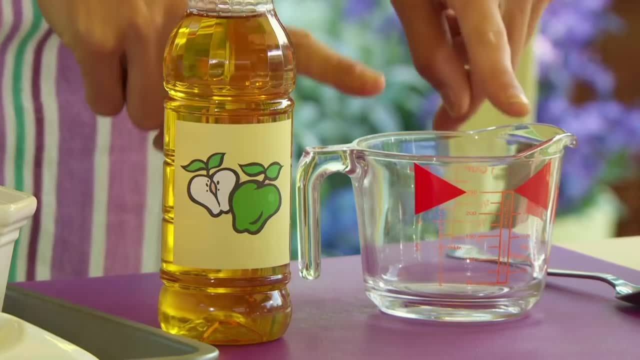 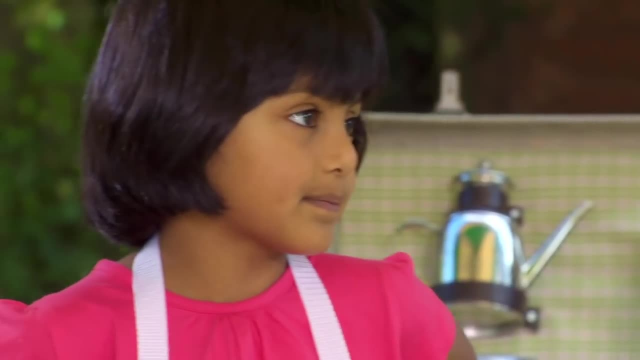 the pourer needs to pour the apple juice into this jug that we've got on our mats and the watcher needs to make sure that the pourer fills the jug up to where the red arrows are pointing. Can you see that line, everyone? Yeah. 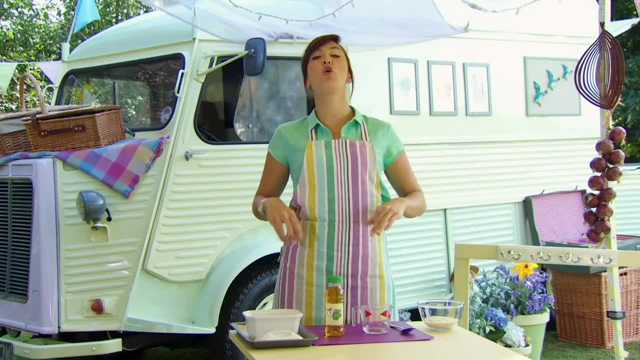 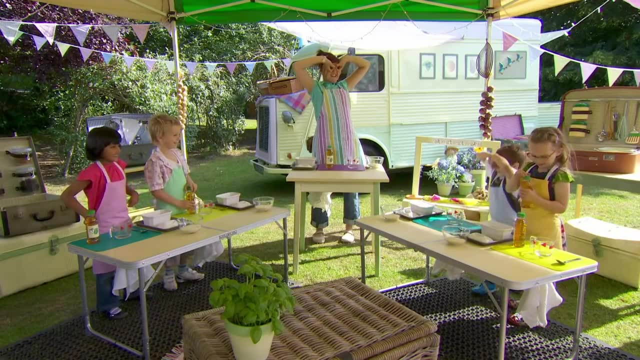 Okay, that's really important, And to be the watcher, you need to put on your watching goggles like this: Ooh, You've got your watching goggles. Yeah Well, let's have a look then Can you be a watcher as well? Brilliant So, everybody. 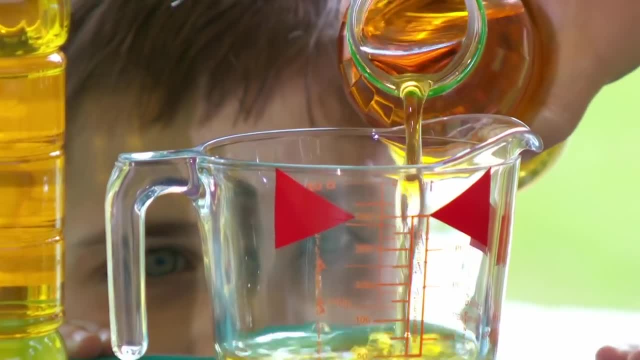 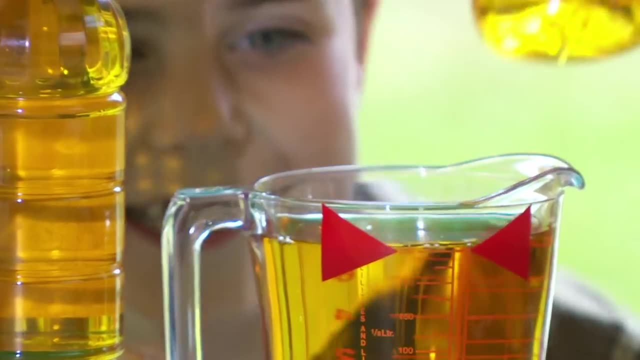 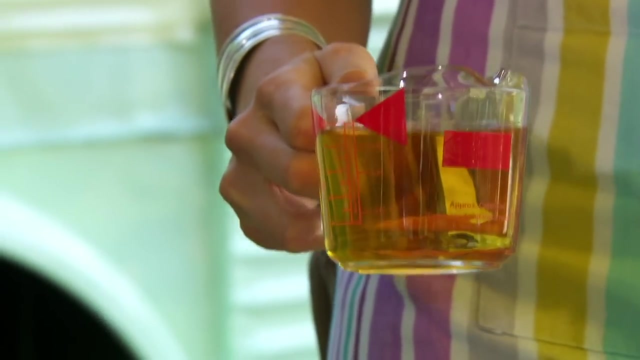 let's get pouring Off. you go, Watch carefully. Tell me what you're going to do. Okay, Tell her when to stop, Sam, Stop. Did you do it Brilliant? Take your jug of apple juice and pour it into your dish. One. 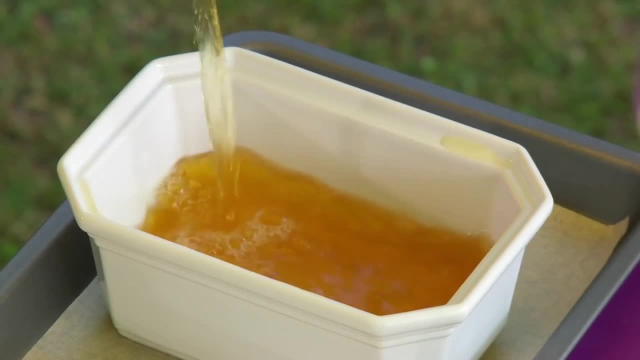 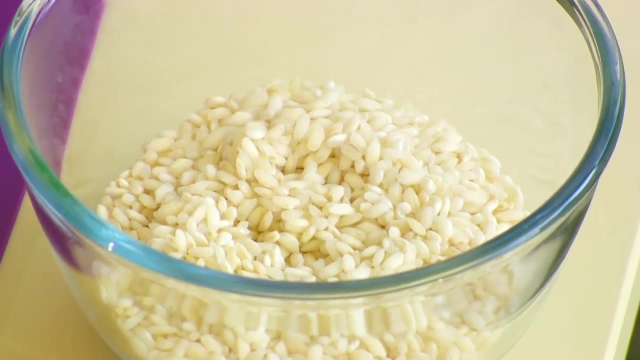 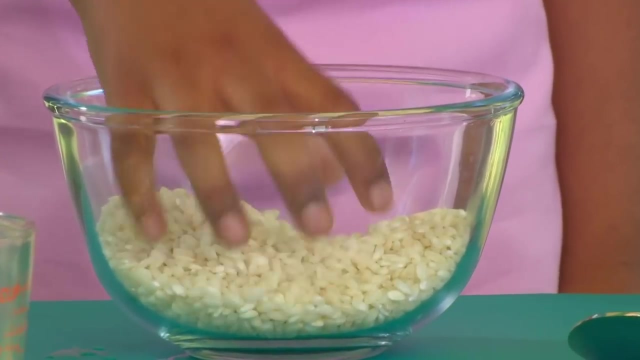 two, three splash. The next thing we need is some arborio rice, and this rice is great to use for risottos and rice puddings. Does it feel nice? Yeah, Ooh, it feels all funny on my fingers. 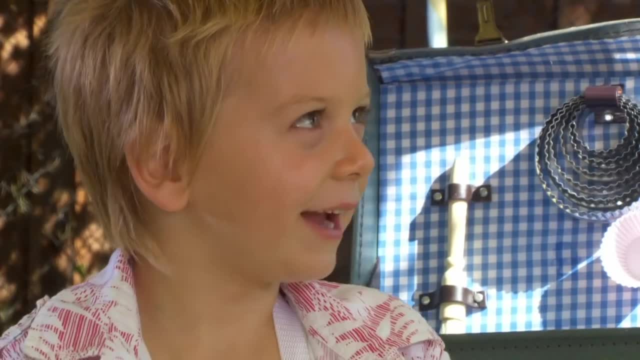 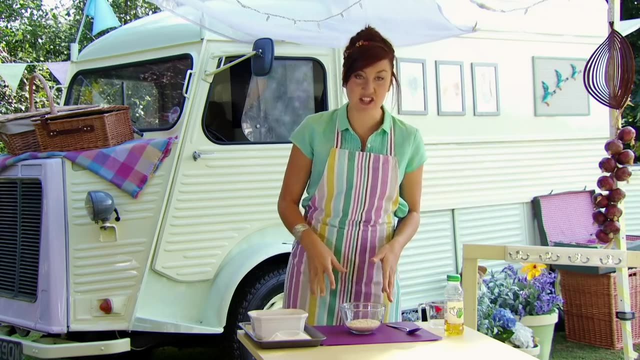 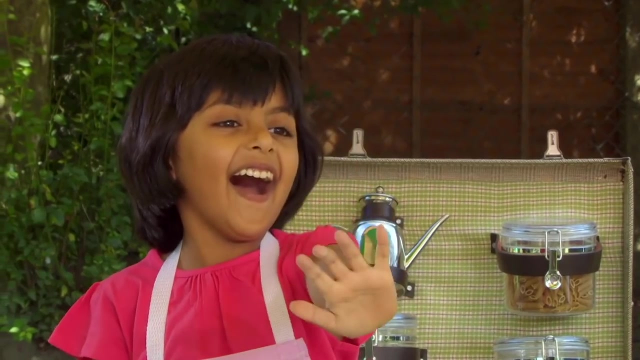 Yeah, me too. What sound does it make Rain? Let's listen. Oh yes, it does sound like rain. Now we need to measure five dessert spoonfuls of arborio rice. How many dessert spoonfuls? Five? 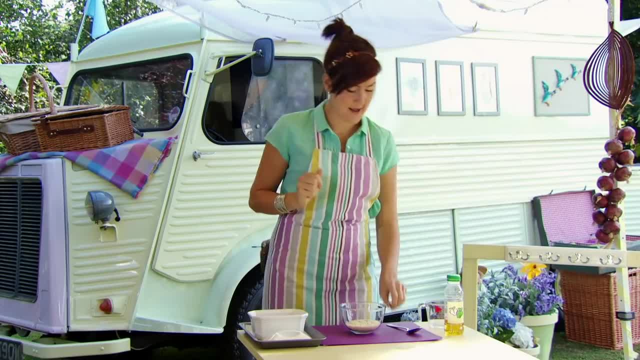 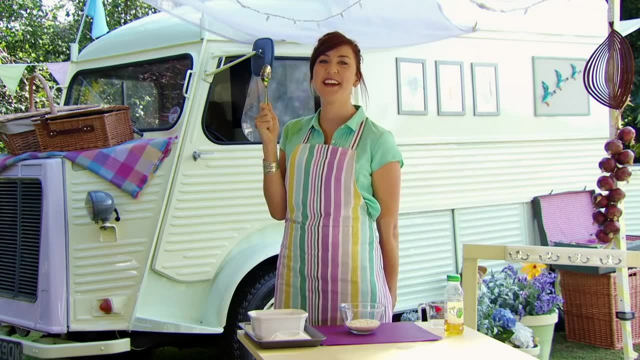 That's it, And to do that we need to use our good friend Mr Spoon. Hello, Mr Spoon. Oh hello. Katie, How are you today? I'm very well, thanks. How are you? Oh, fantastic, Can't wait to do some measuring. 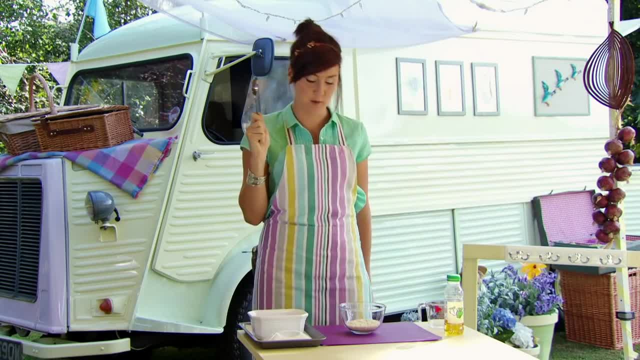 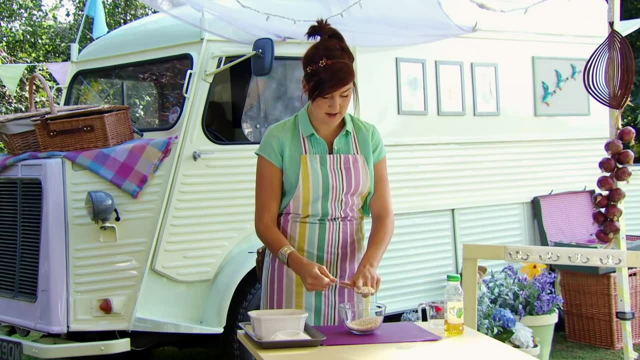 Okay, Mr Spoon, Let's measure five dessert spoonfuls of our arborio rice Ready- Here's one- And pat it. so it's nice and flat: Pat pat, pat, pat, pat And then put it into your. 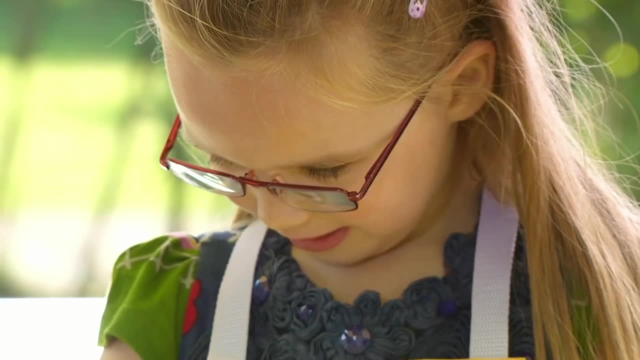 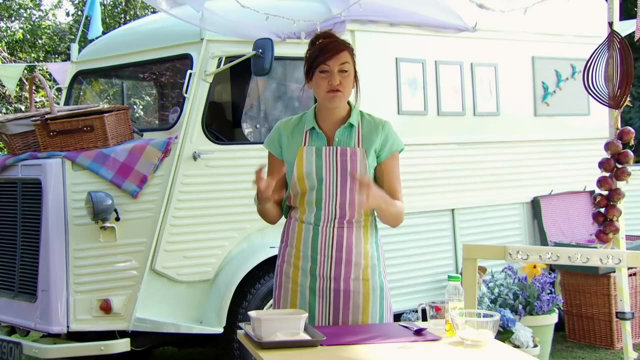 dish with the apple juice, And when you've done your fifth one, you just put your spoon back into your bowl. Now what's going to happen is quite exciting. The rice is going to soak up all of the apple juice like this. 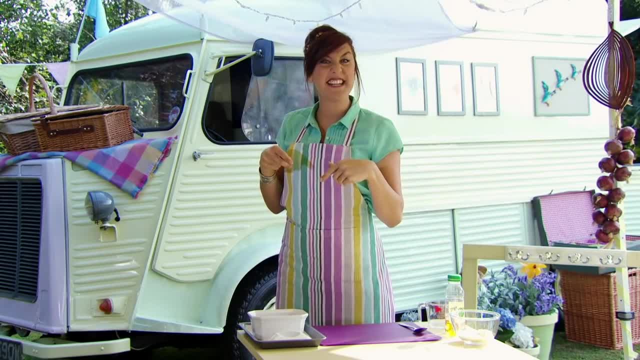 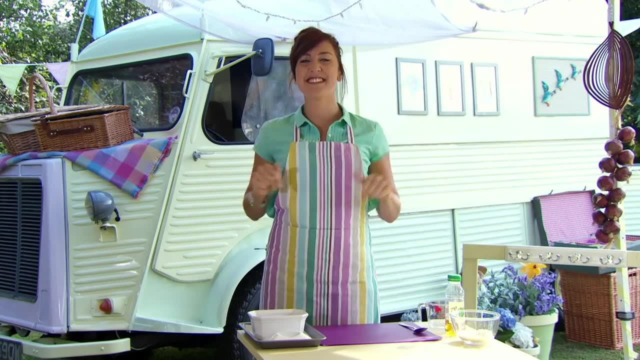 Shall we all pretend to soak up the apple juice altogether? You can join in with us, Ready, Brilliant. So what do you think we're going to need next in this recipe? What's next? Well, let us see if you can guess what it could be. 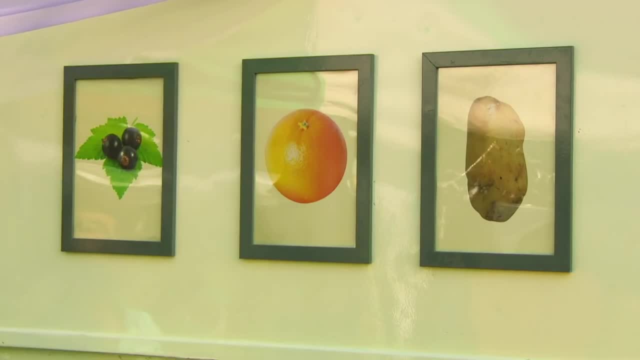 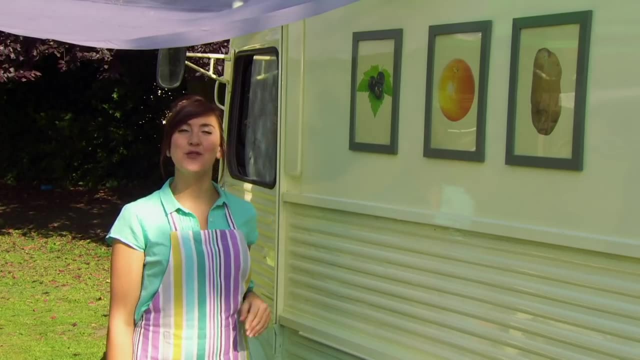 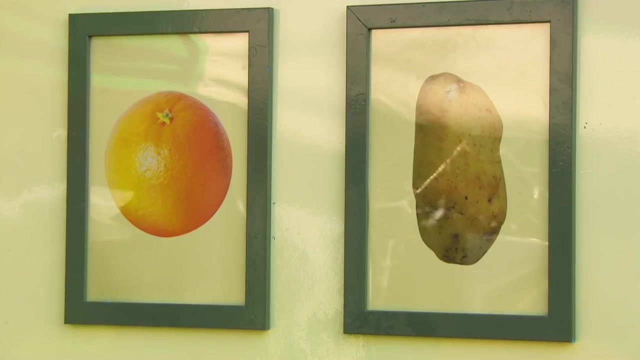 So we have got a potato, an orange and some blackcurrants. What would you choose for our baked blackcurrant rice? Oh, I know, I'll give you some clues. The special ingredient is a fruit. Well, potatoes are a vegetable, aren't they? So we can take that one away. 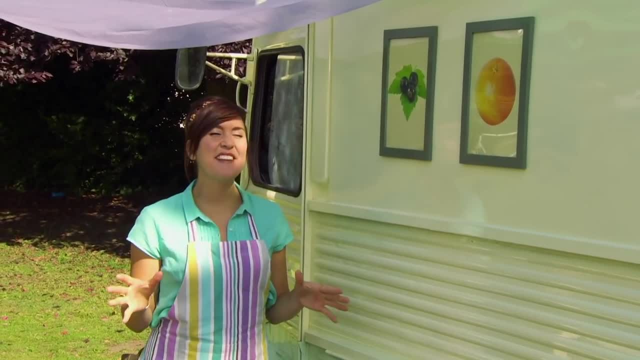 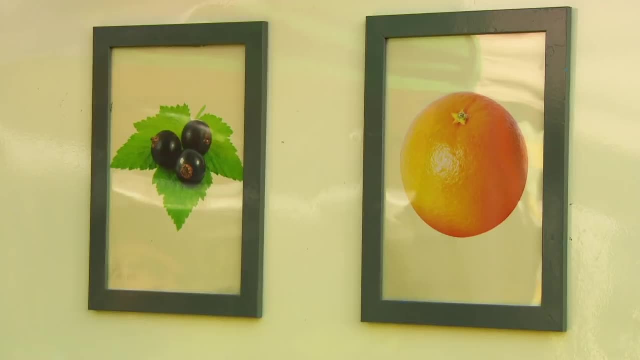 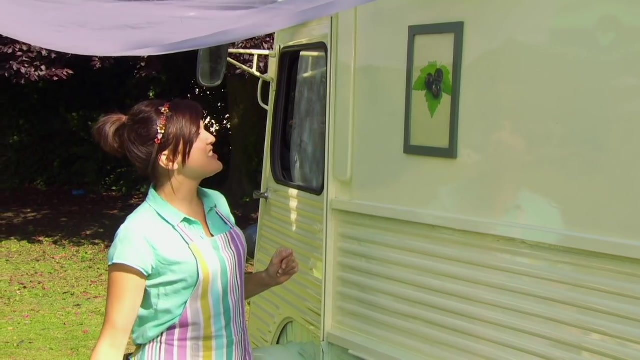 There we go. Okay, I'll give you another clue. The special ingredient is a fruit that grows on bushes. Well, oranges grow on trees, don't they? So we can take that one away too, Which leaves us with blackcurrants. We're going to need some blackcurrants for our baked blackcurrant. 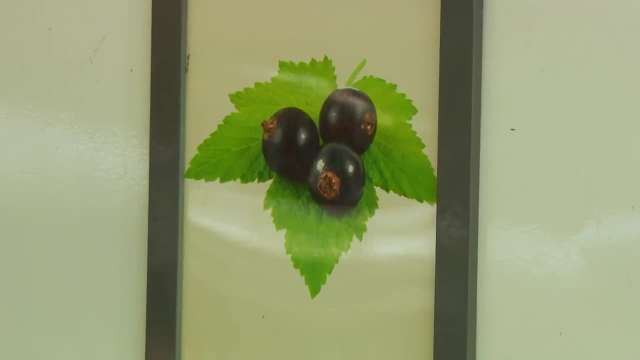 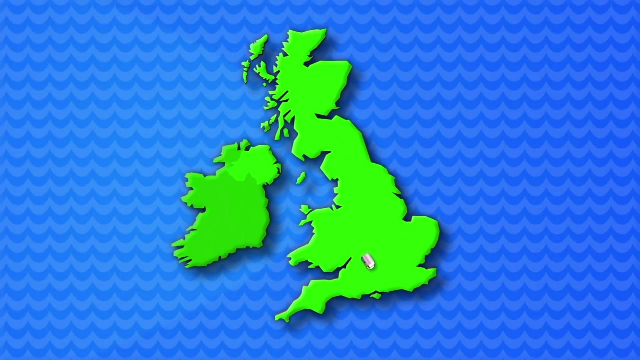 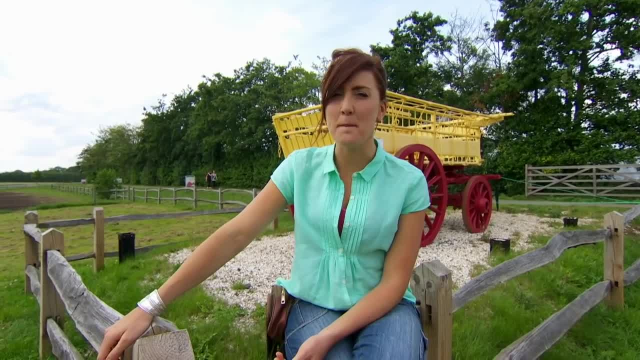 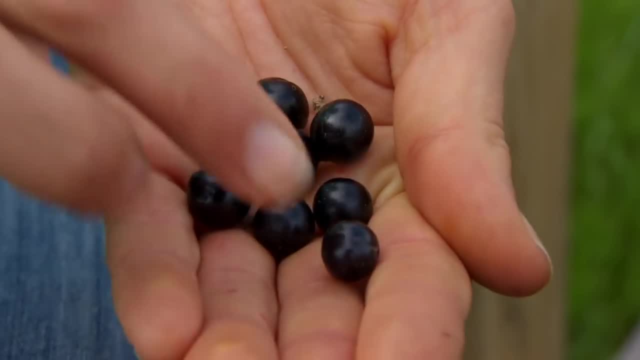 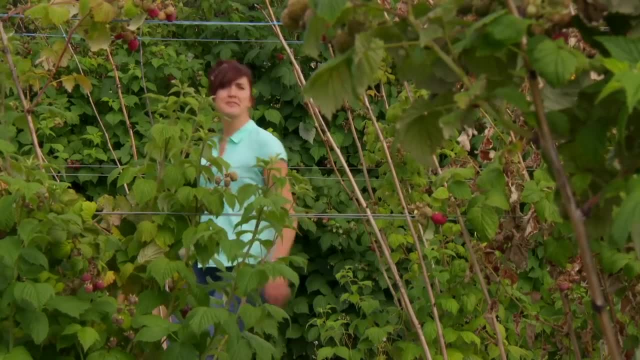 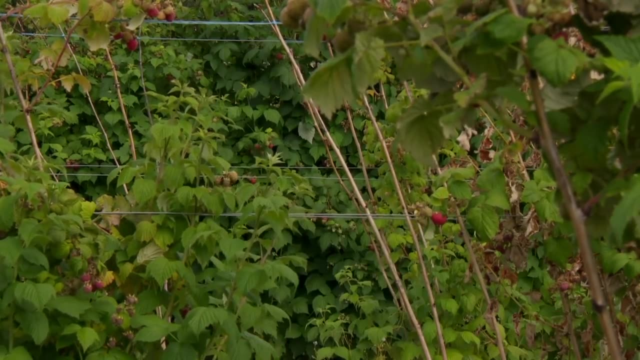 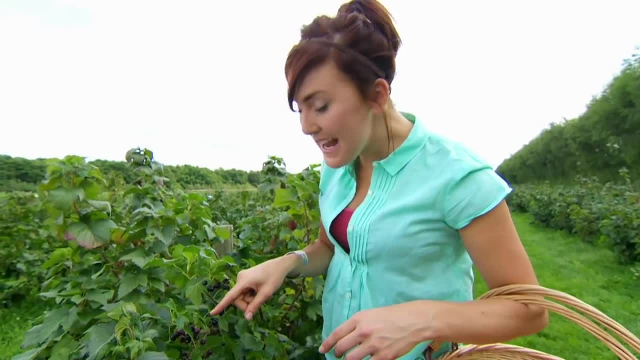 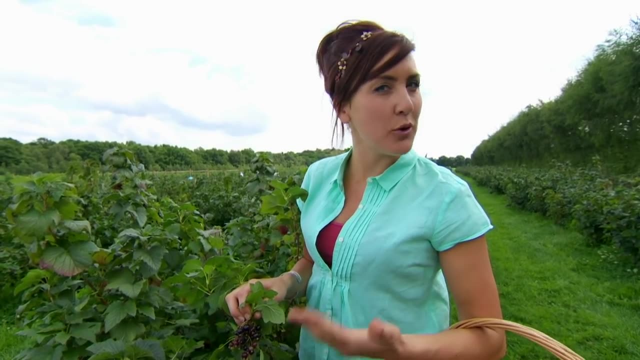 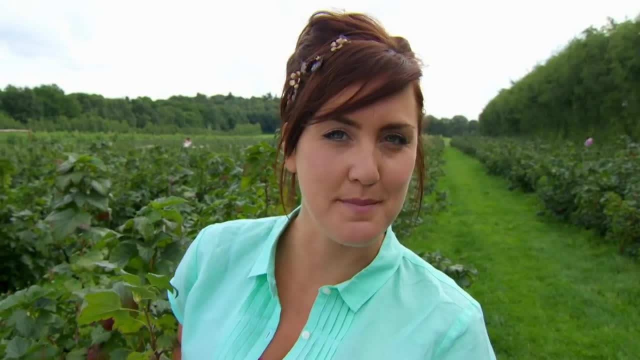 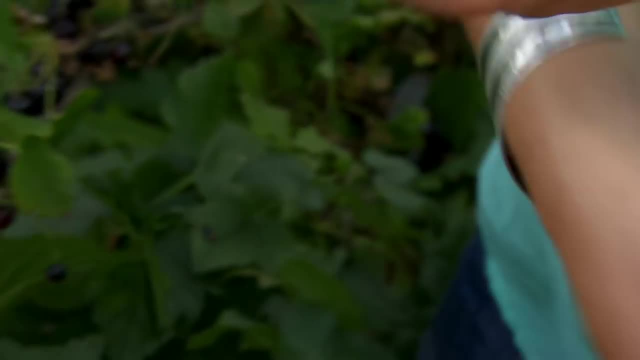 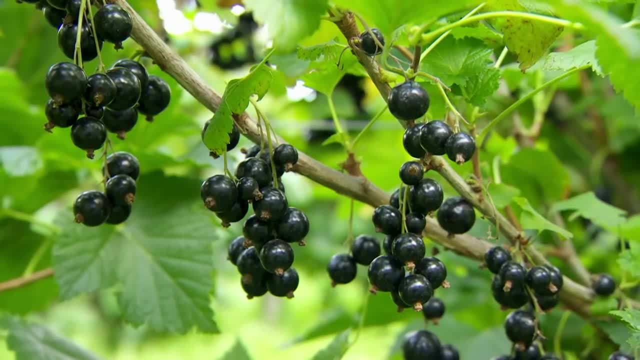 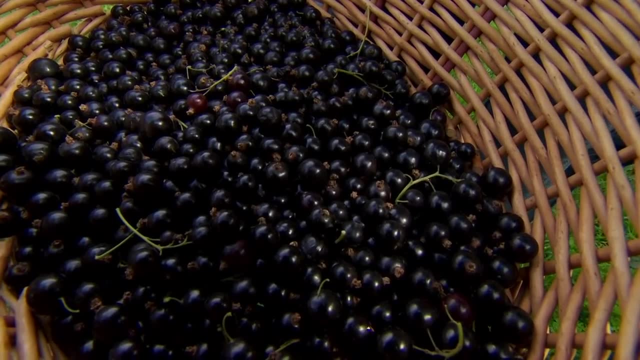 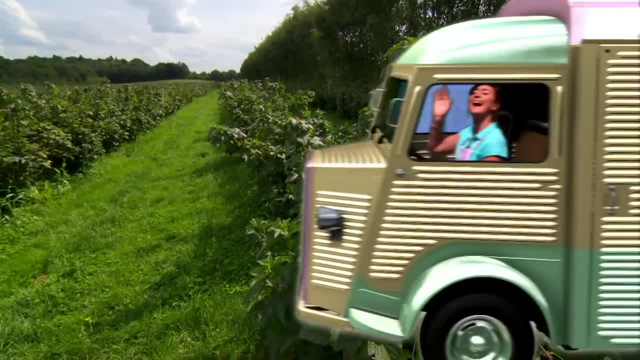 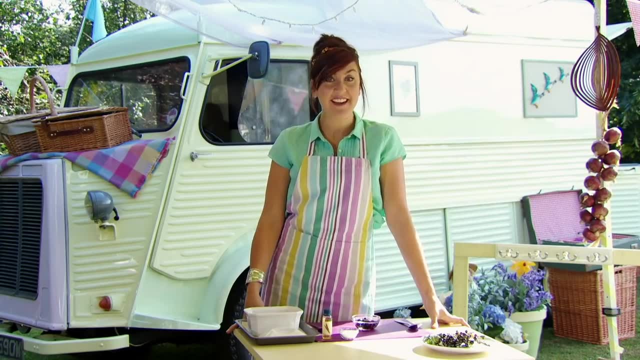 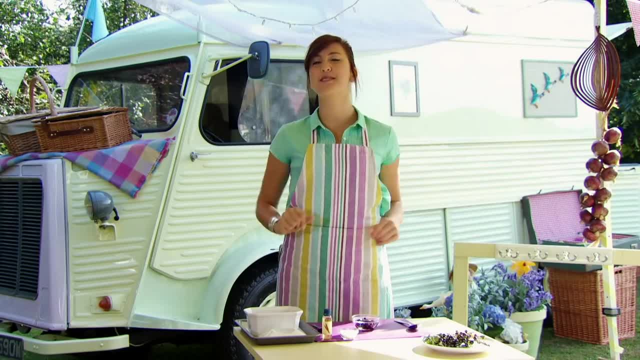 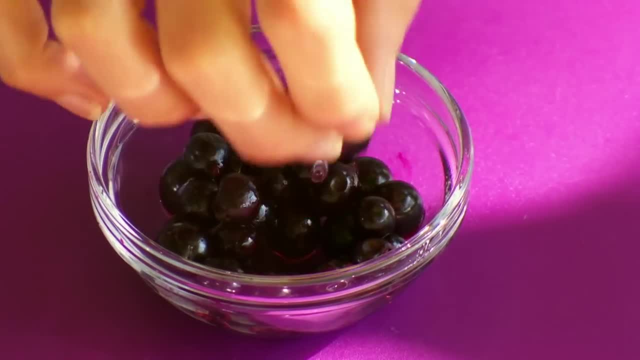 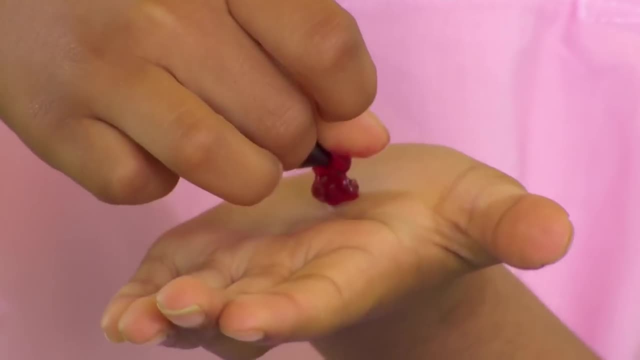 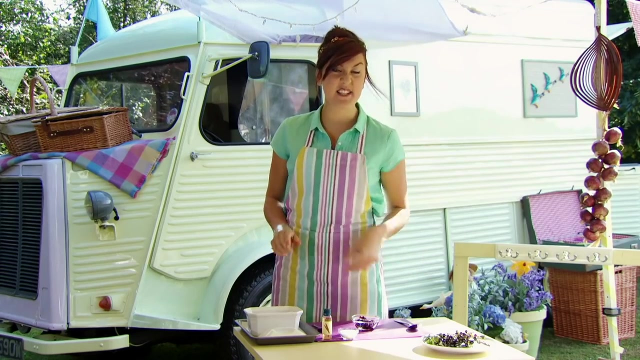 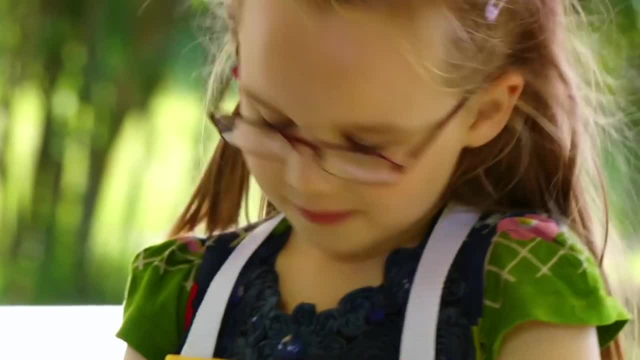 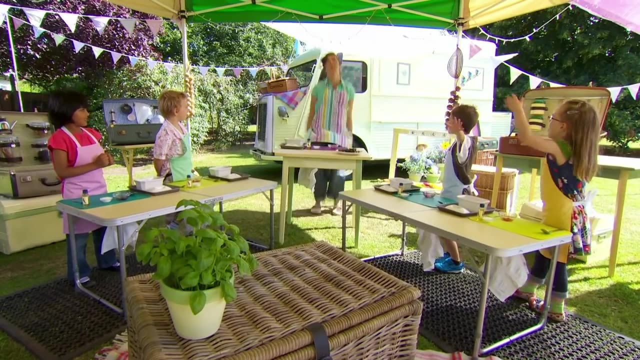 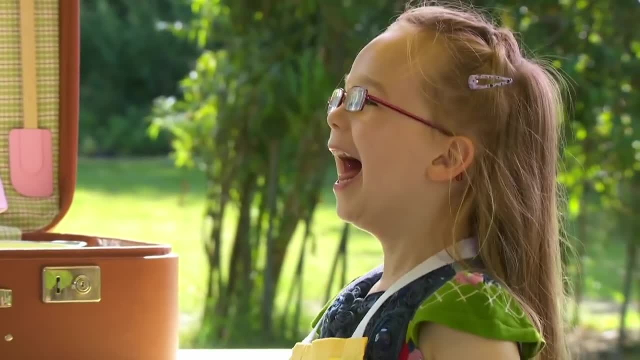 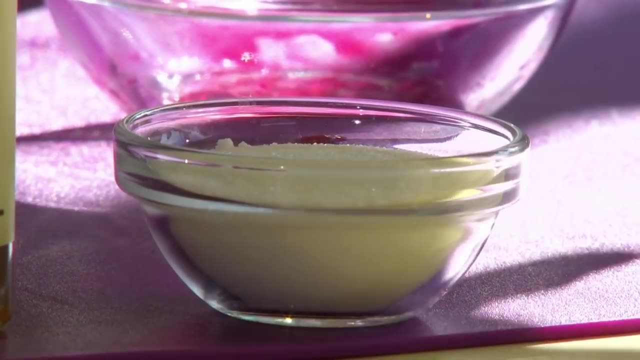 One, two, three pop. OK, now the next thing we need to add is some sugar, and we're going to use caster sugar. Now, caster sugar's a little bit different to the kind of sugar that you might be used to using when you're at home. 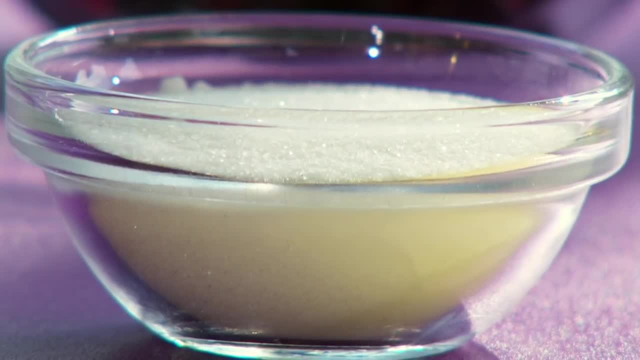 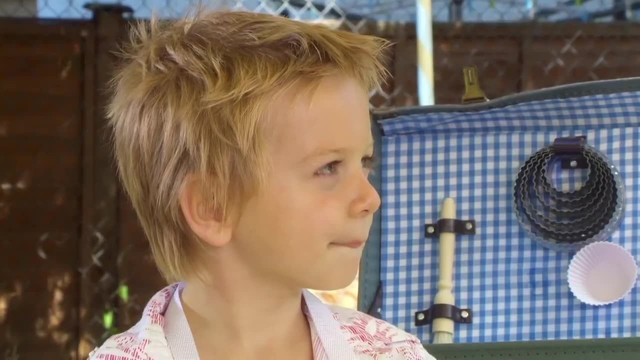 and that's because the granules, which are the little pieces, are much smaller. Now we need to sprinkle this sugar into our dish, and we're going to do it by doing the sugar shuffle. Shall I show you how to do the sugar shuffle. 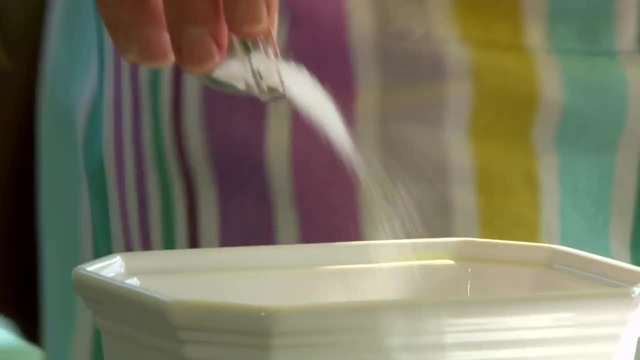 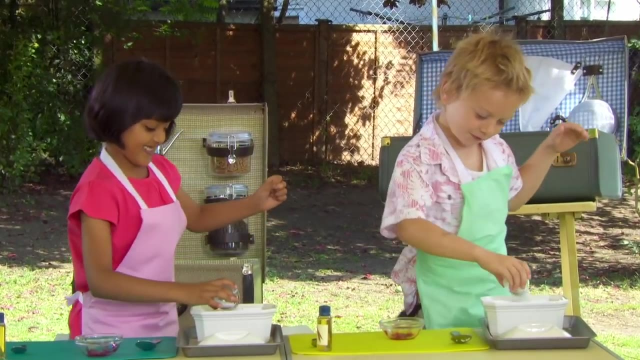 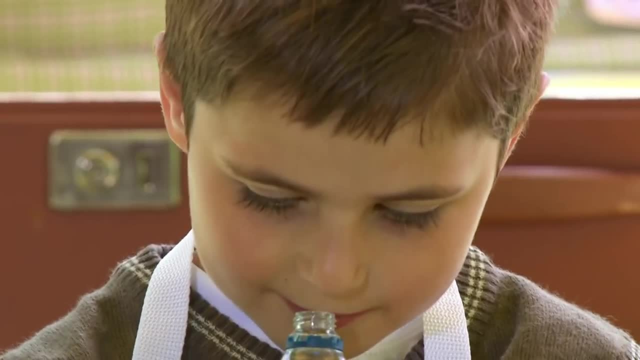 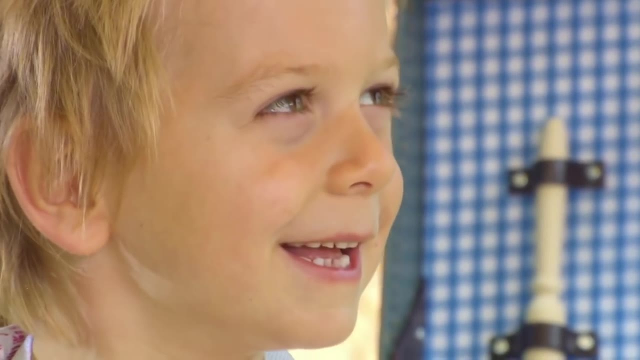 Shall we give it a smell before we add it? Yeah, OK, Eddie. what does it smell? like? Ice cream, Vanilla ice cream. Do you like vanilla ice cream? I love it, And we need to measure half a teaspoon of vanilla extract. 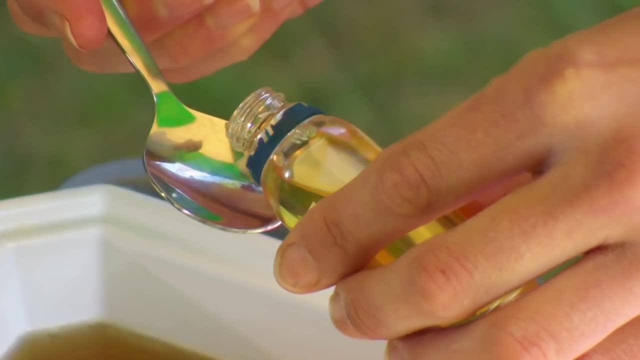 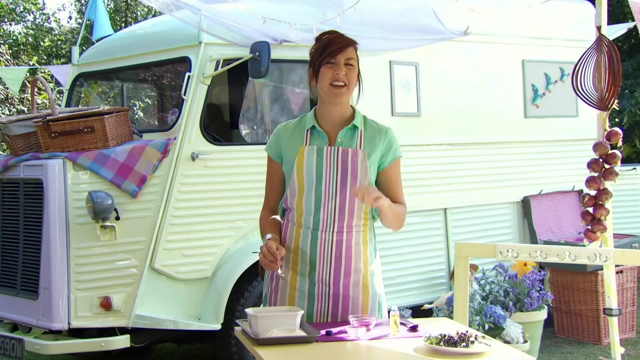 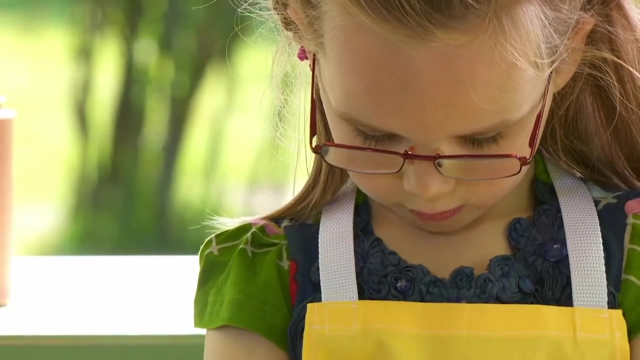 So hold your teaspoon over your dish- and very carefully, That's enough- and splash it in. Now the last thing we're going to do is give everything in our dish a good stir, but we have to give it a really slow stir, because otherwise all the things are going to splash out of the dish. 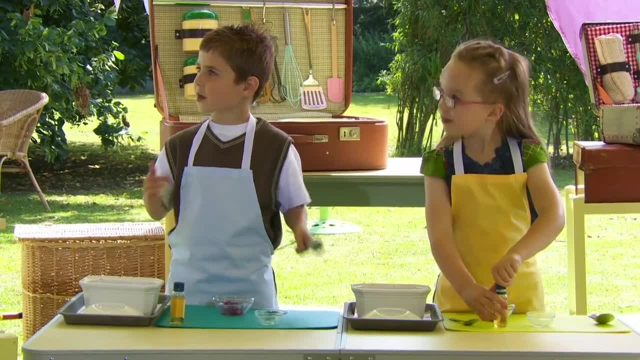 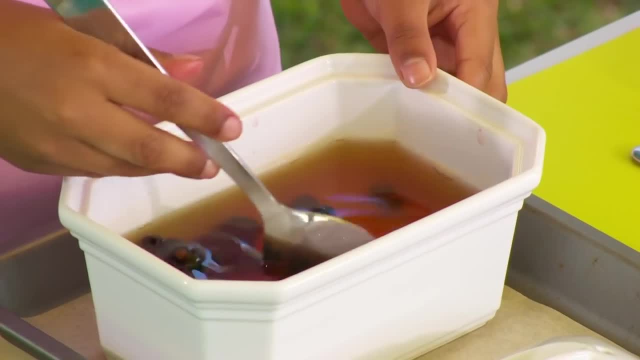 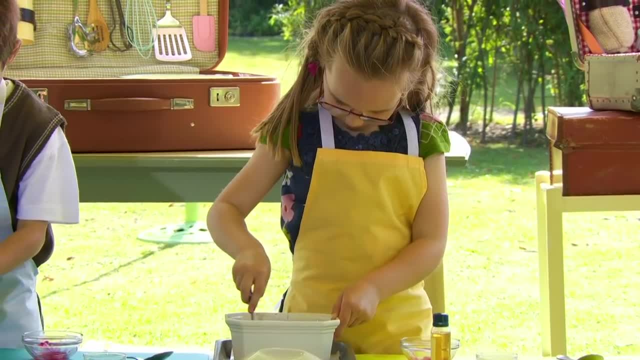 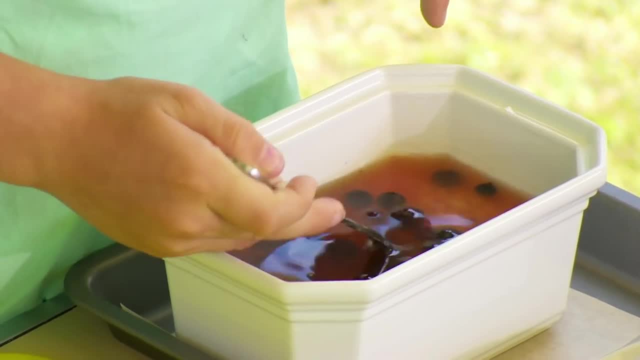 Oh, the colour's coming out of the black currants in mine. Yeah, I can see the juices coming out because it's red all around. Is that the juice from the black currants? Yeah, What do you think is happening to the sugar? 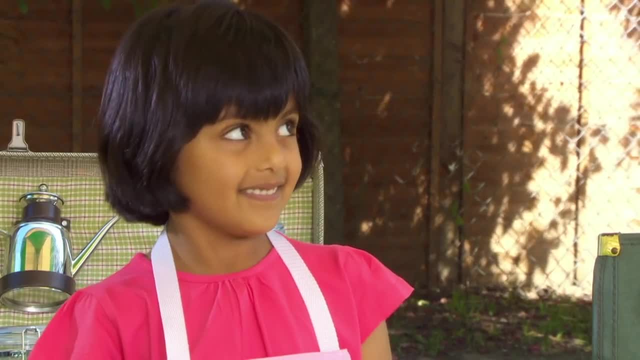 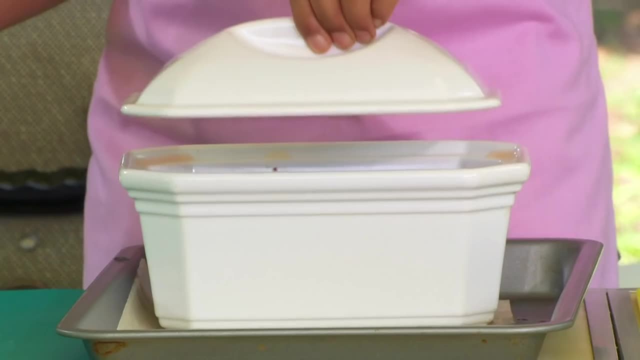 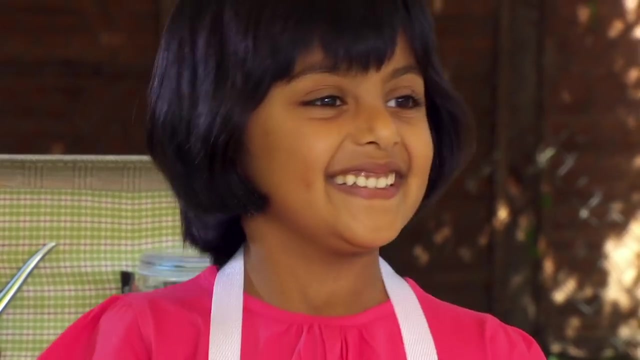 It's gone. Do you think it's dissolved like this? Yeah, OK, put your spoons down and then you can pop your lid on Excellent. And that is it everyone. You did it. You put all the ingredients together for your baked black currant rice. 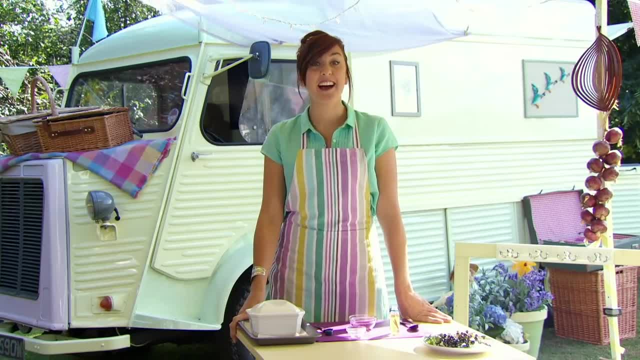 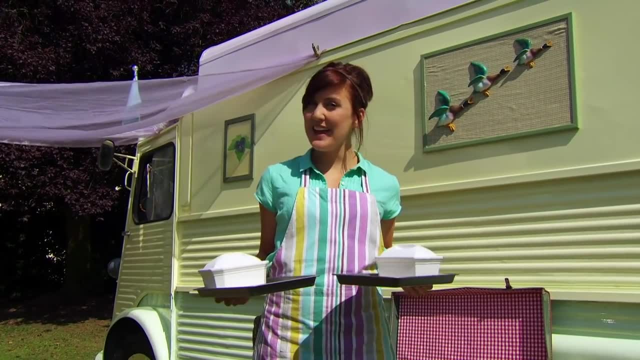 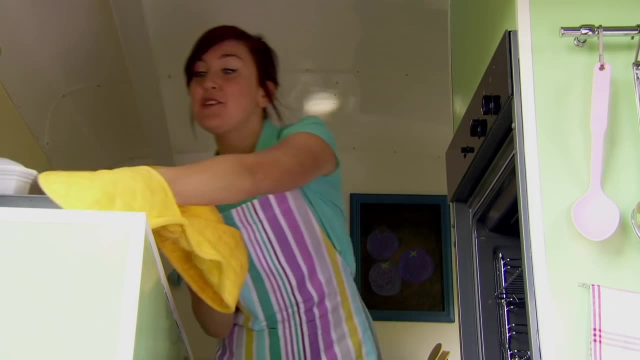 and you did it all by yourself. Well done, And now let's put them in the oven. Remember, ovens are hot, so don't go near. Ask a grown-up to help you here Now. we've cooked with you and had lots of fun. 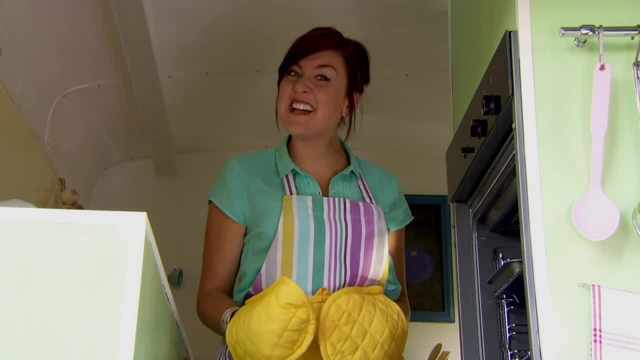 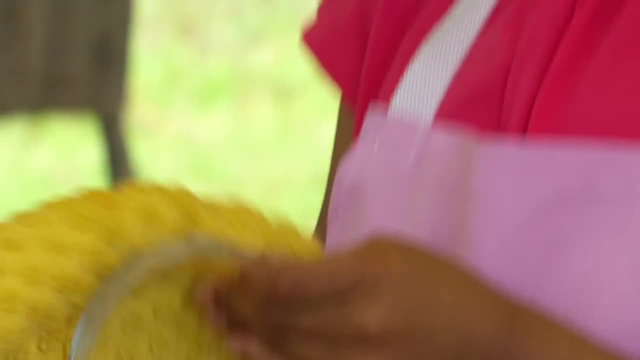 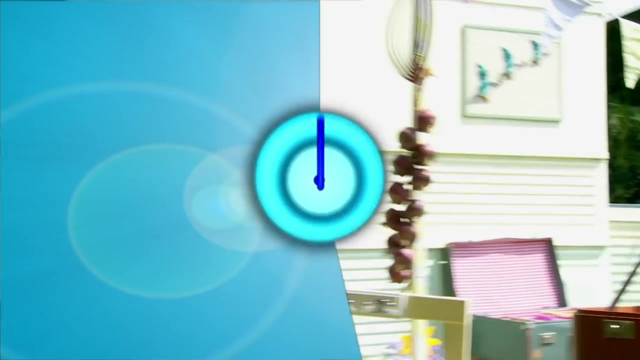 Let's tidy up and think of all the things that we have done. There was measuring, scoring, sprinkling, stirring, clearing any mess and putting things away. It's always fun to do at the end of the day. And here they are, all ready to eat. 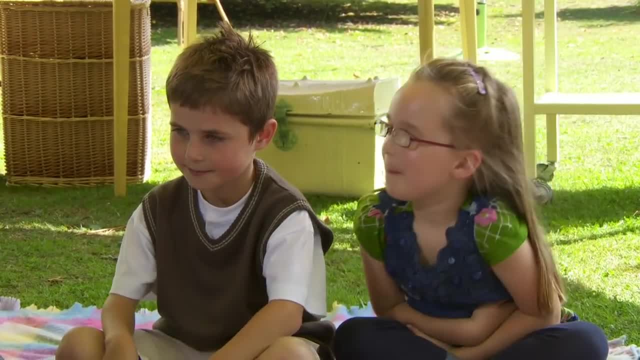 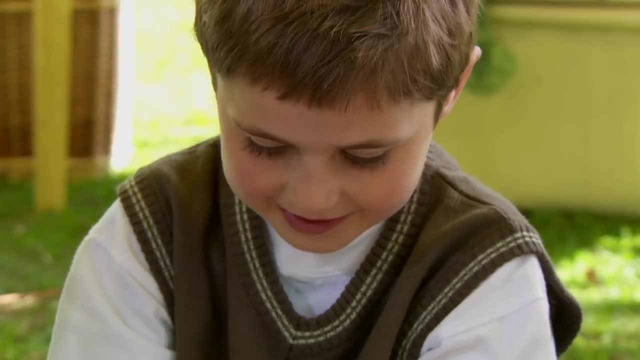 I'm so excited to see how they've changed, Are you? Yeah, OK, Sam, let's have a look at yours. Ready Open, Oh wow. What colour's it gone, Sam Red? Why's it gone red? 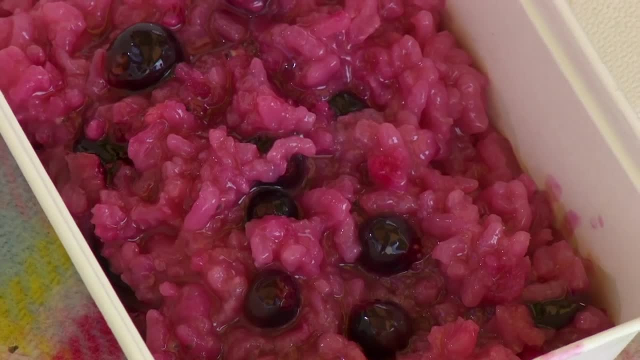 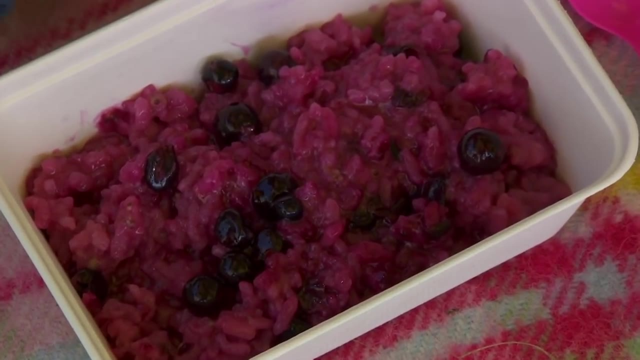 It's because the black currant juice has squirted all over the rice. OK, Ria, are you ready for yours? Open sesame. Ooh. What does it smell like Fruit? Of course, because it's got the black currants in it. 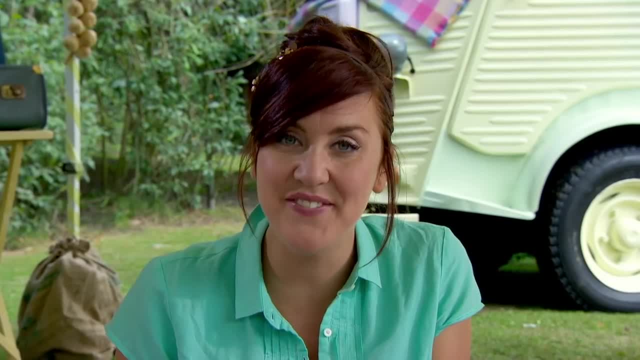 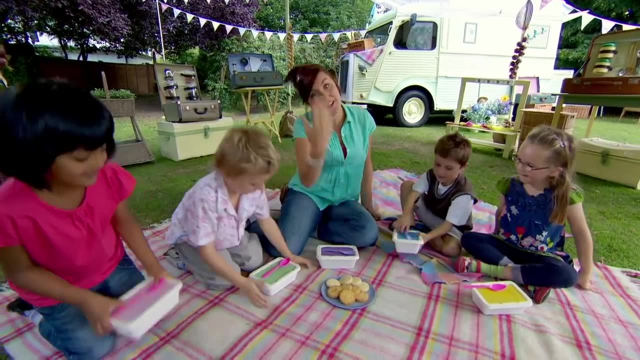 Shall we put the lids back on. We've travelled to you, cooked and had fun. Now let's have a party with everyone. Yay, Yes, I can't wait And you can come too. Come on, follow me, I'll carry the biscuits. 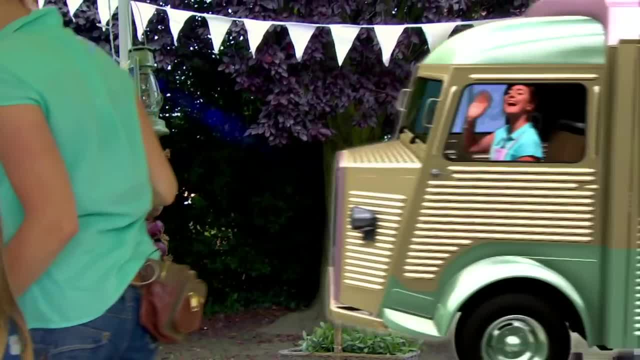 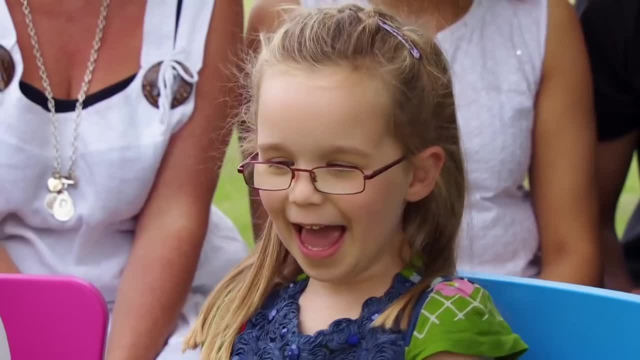 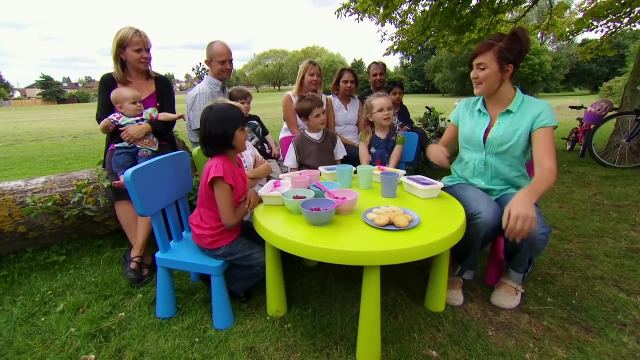 Oh, let's carry them together, Ria. Well, here we are at the park and we're all ready for a picnic, aren't we? everyone? Yay, Oh, I am so hungry and I've made some extra baked black currant rice for everyone else. 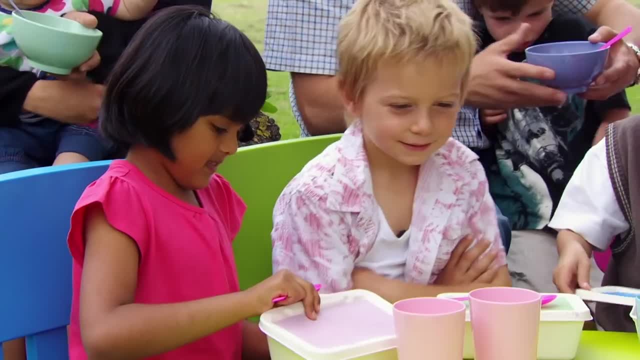 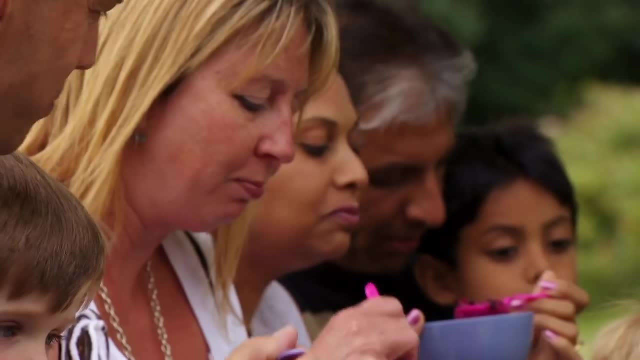 So here you are. everyone Dig in. Oh yes, biscuits, Mmm, Mmm, Mmm. That's really nice, Very delicious. Oh damn, We could do this again, but we could use a different juice. What? 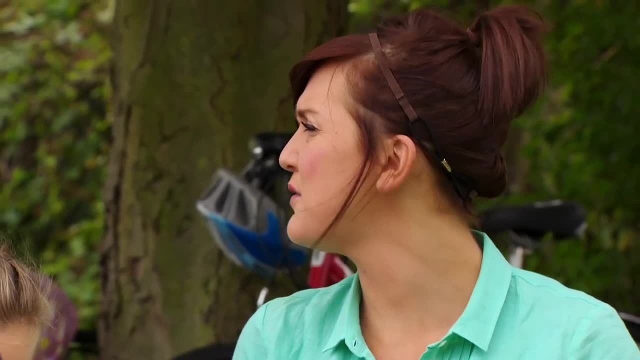 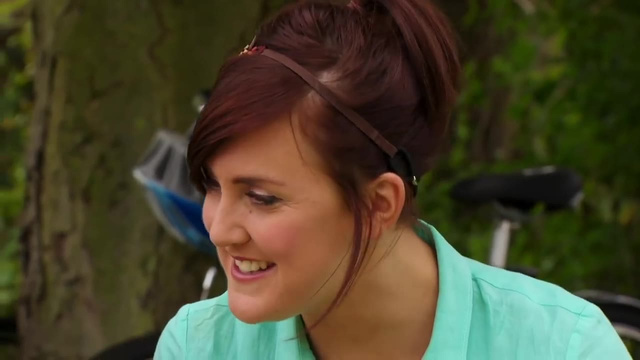 What juices do you think we could use everyone? Strawberry, Strawberry juice. What about peach juice? Blueberry juice, Sam, are you happy with what you've made today? Mm-hm, How many marks out of ten does your baked black currant rice get? 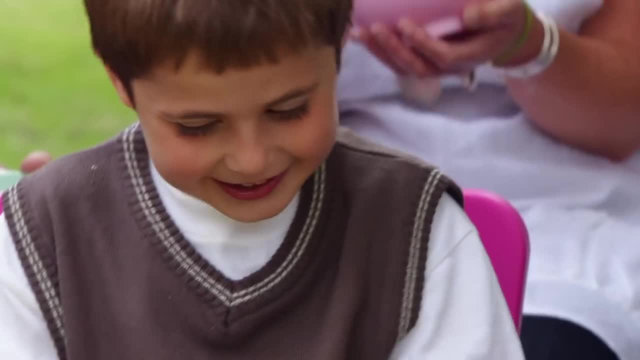 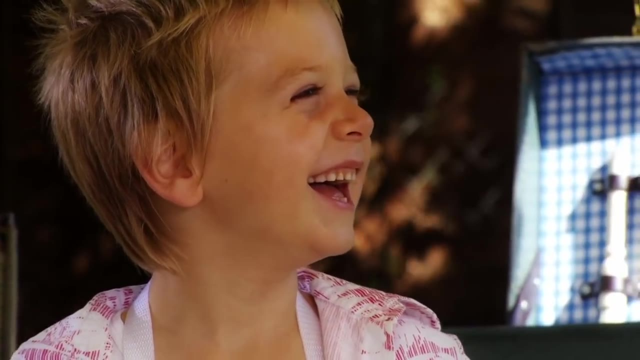 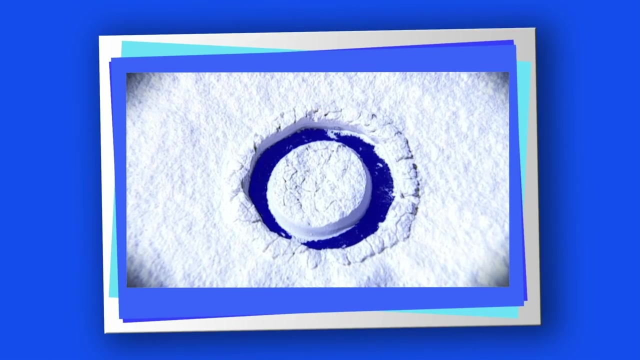 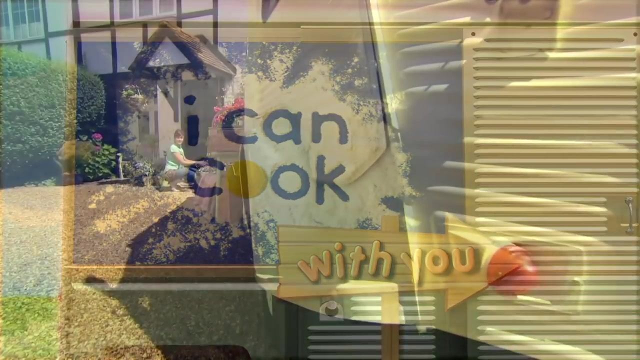 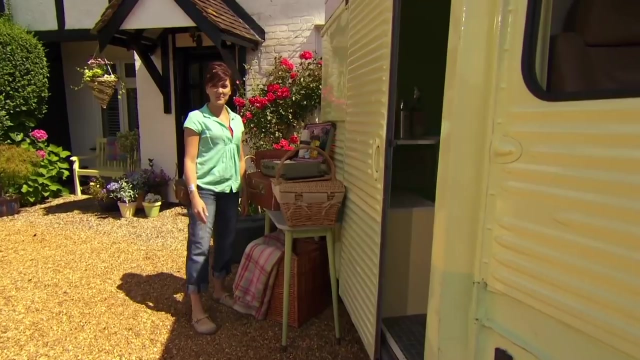 20.. 20?. So what can you do? everyone I Can Cook With you. Oh great, I've been waiting for you. I've got everything ready to go on a journey. go on a journey. I hope you're going to come with me and meet some new friends. Aha, here. 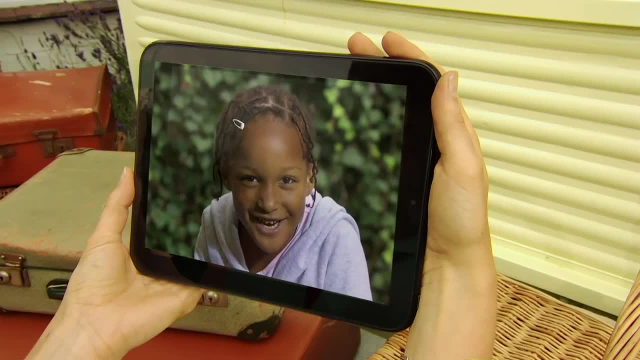 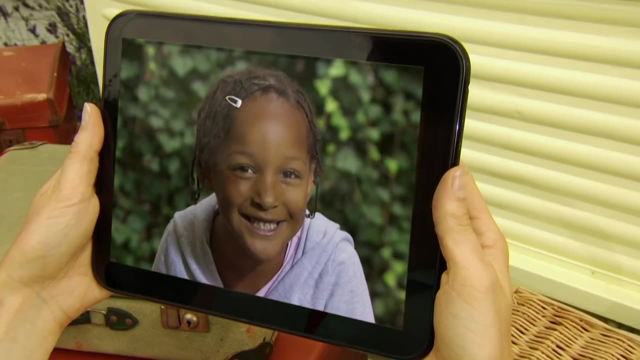 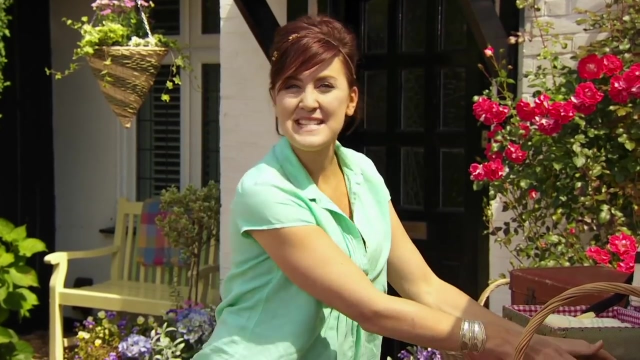 we are. Hello, Katie, I love playing basketball. Can we make something with mushrooms? They're my favourite. Katie, can you cook with me, please? I can, And you can cook with me too. Gosh, I love mushrooms, don't you? Come on, let's pack everything up and be on our way. 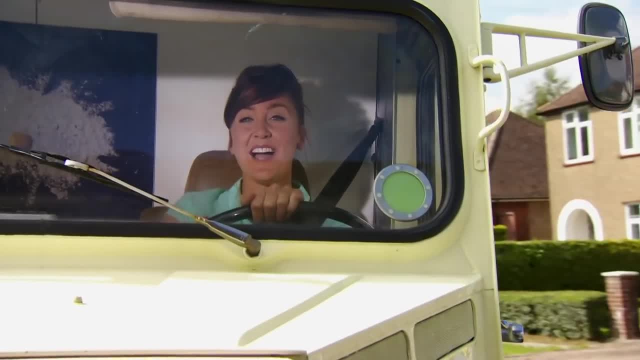 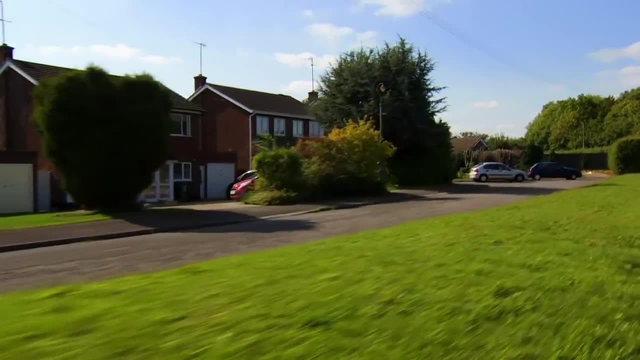 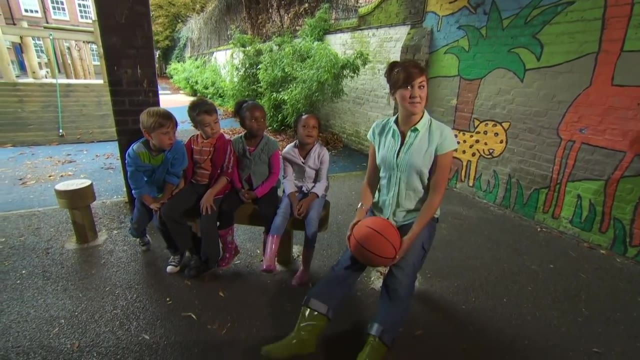 I'll be on a journey and I'm coming to you. It's going to be busy and there's lots to do. Get ready to help, join in and have fun. Let's cook a feast for everyone. Well, I've got my basketball and I'm ready to play, and I've just found Tiffany and all. 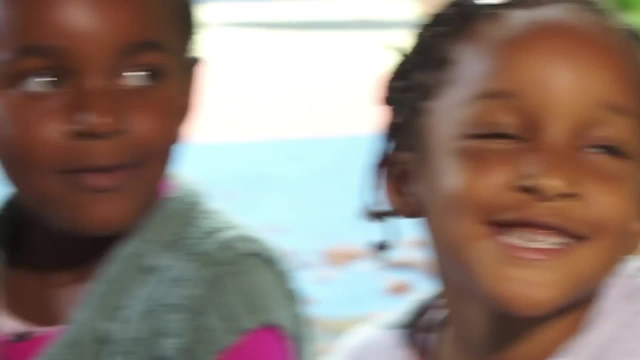 of her friends. Hello Tiffany, Hello Katie. And what's your name? Diana, David, And how about you at the end, Honey? Well, it is brilliant, It's a great day. It's a great day, It's a. 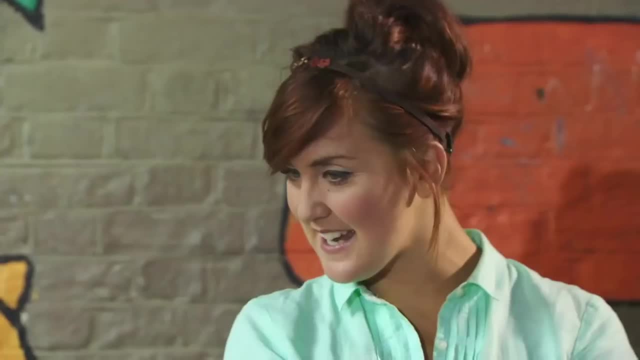 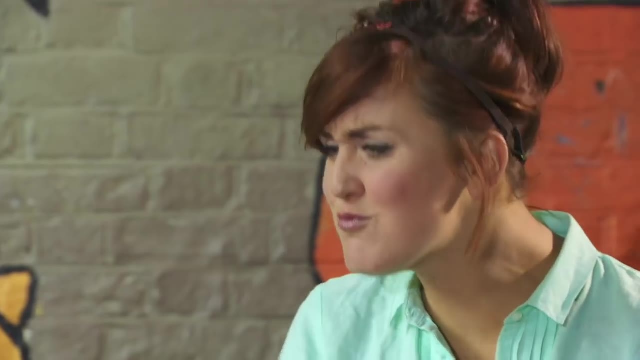 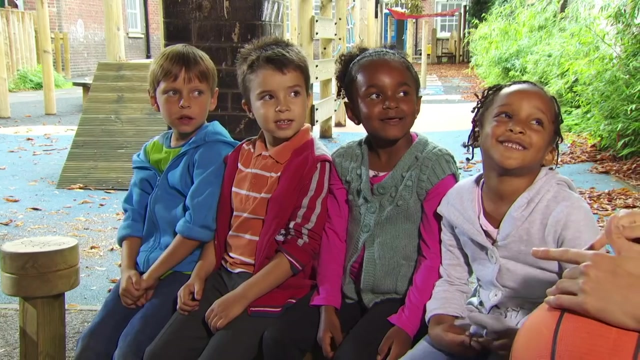 brilliant to meet all of you and I'm so excited. What are we going to do today? Tiffany, Make something with mushrooms and play basketball. Oh, brilliant, I have got the best mushroom recipe. Do you all want to cook it with me? Yes, And, and, and. should we play basketball? 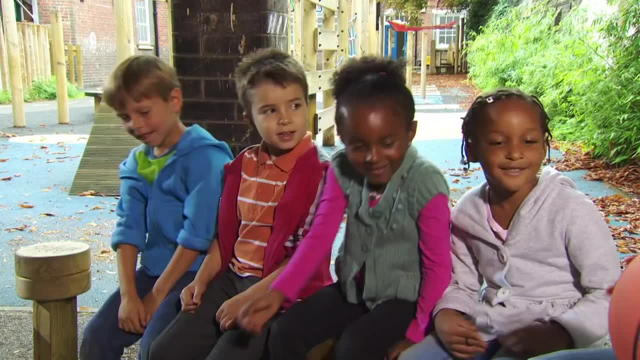 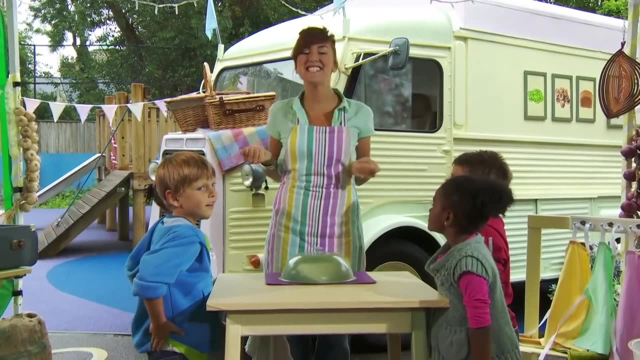 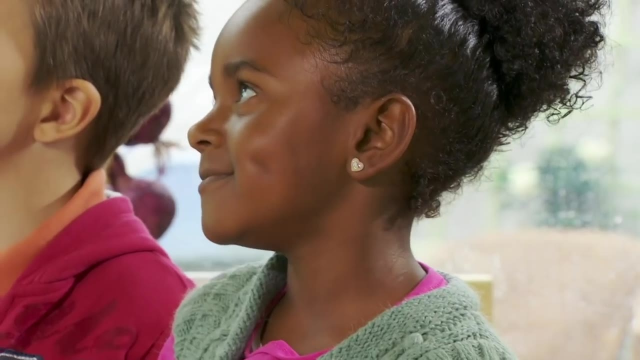 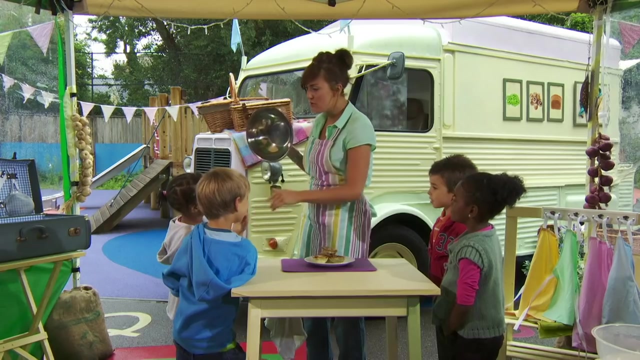 afterwards? Yes, Sounds like a plan. Come on, everyone follow me. Welcome to my outdoor kitchen. Yay, Who wants to know what recipe we're going to cook Me? I'll tell you what it is. Today's recipe is playtime popovers. Mmm, Hey, they look tasty, don't they? Oh, don't you take. 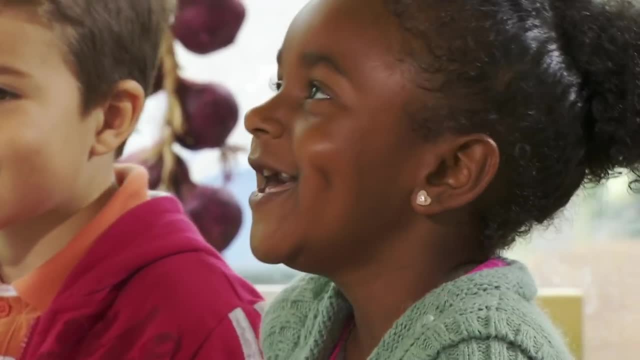 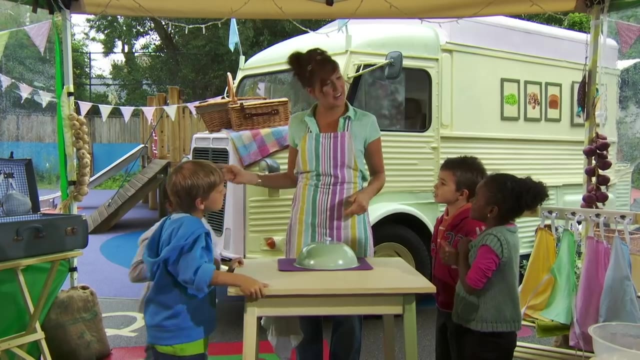 one. yet, you cheeky pickles. Now, before we get started on the cooking, we've got to do something first. What do you think it is? Wash our hands, Wash our hands. You've got it Off. you go, team. 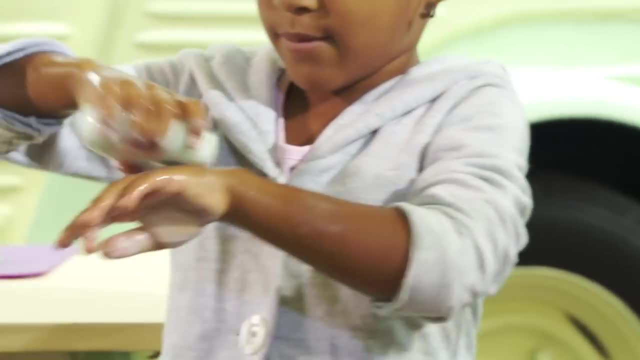 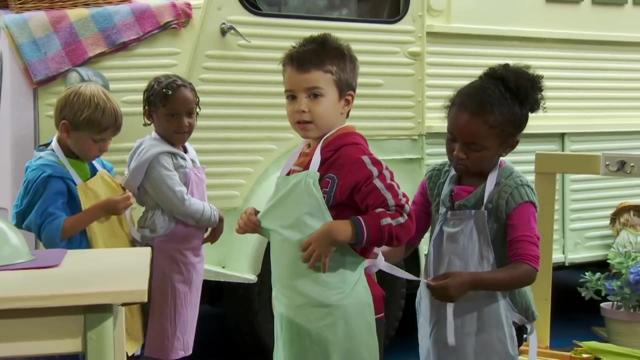 Roll up your sleeves. Give your hands a wash With slippy dippy soap, Splish, splash, blosh. Have you done? your hands Washed and dried? Sleeves rolled up, Apron tied. What can you do? I can cook. 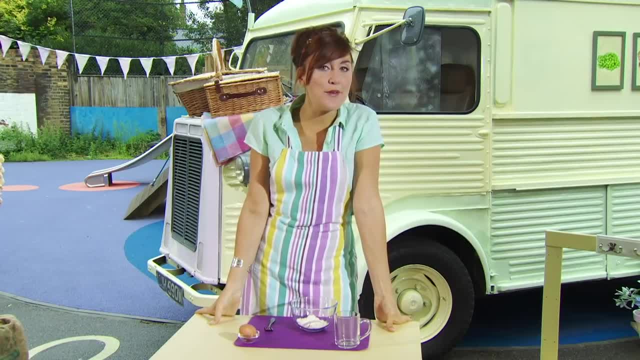 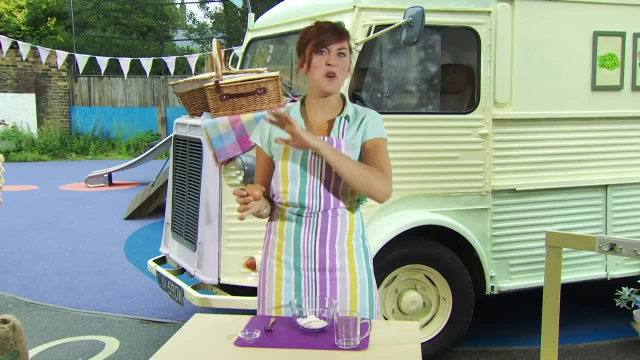 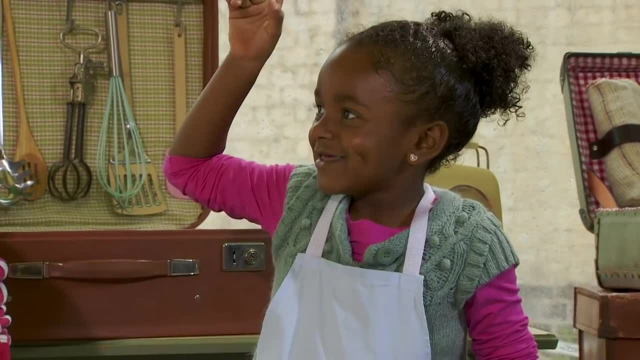 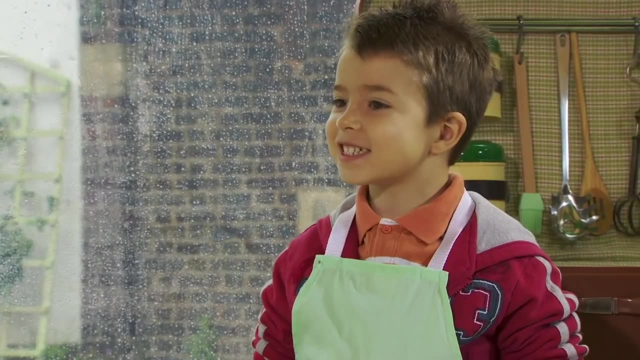 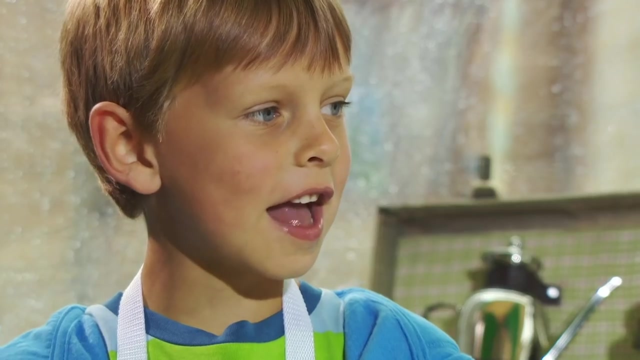 A chicken, A chicken Who can pretend to be a chicken. And we're going to crack our chicken's egg into this cup. Knock, knock, knock, Make a nice big crack. Can you see it Like that? Yeah, And then we've got to use our thumbs to open it up. Watch this Ready. Ooh, open sesame. 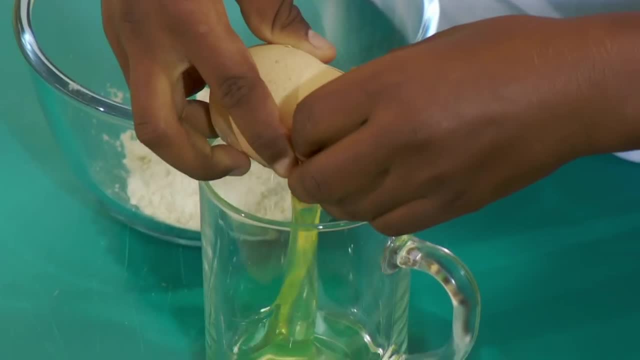 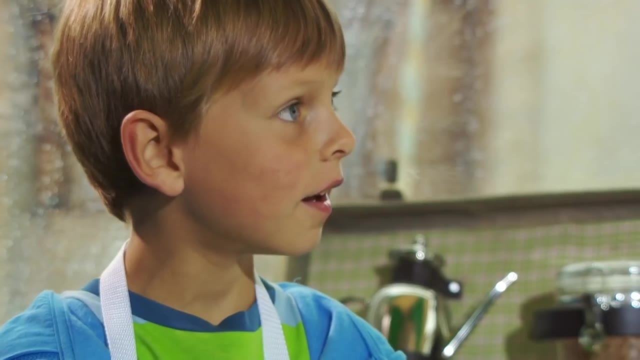 And there's our egg. Look at that. That was a good one actually. Oh, We all love it, We all did it. Everyone say yeah, Yeah, Yeah. The next thing we need to do is some whisking, And we're going to whisk using our fork. 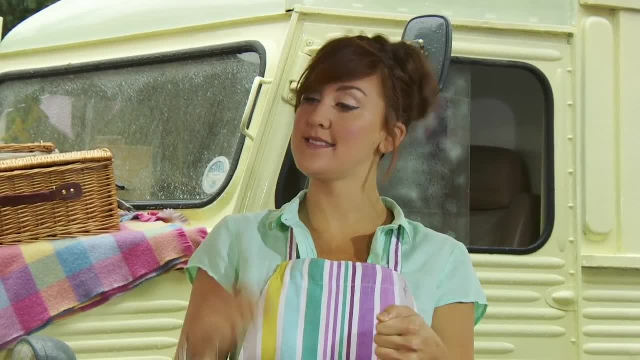 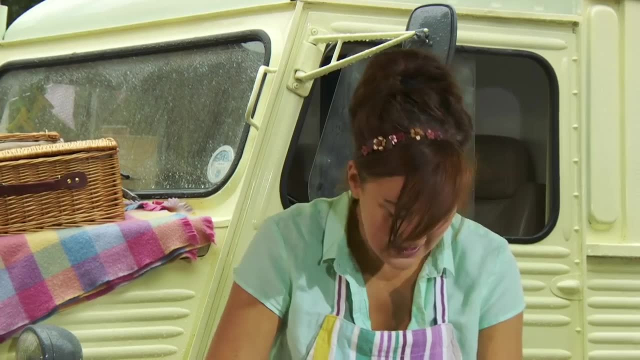 And you can do whisking at home too. You just get your cup like this and your fork like that And you go whisk, whisk, whisk, whisk, whisk. Are you ready? team Yeah, Hold the handle And let's get whisking. 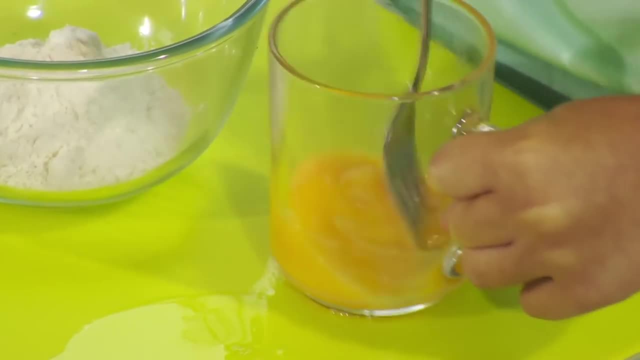 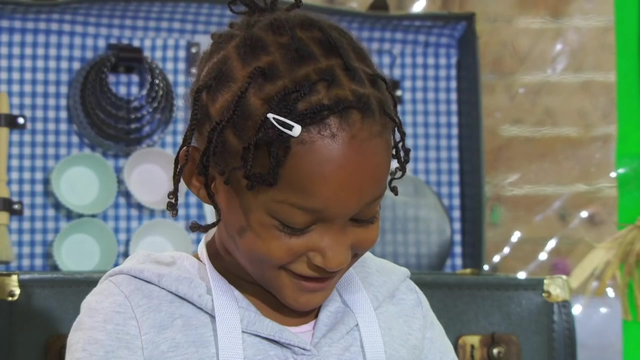 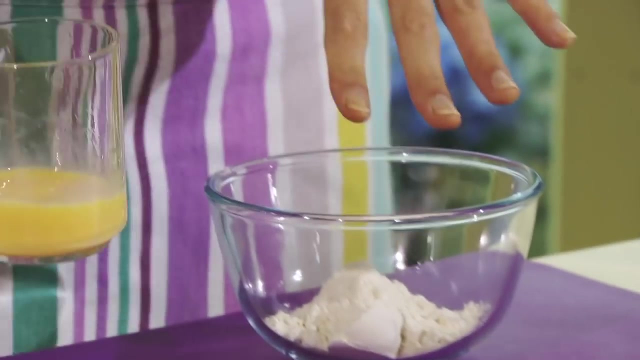 This is fun, And when you've whisked your egg up properly, it'll look all gloopy. Look at this, See, Ooh Ooh, Ooh, Gloopy. That's just right. And we need to splosh this egg into this bowl of flour that we've got here Ready everybody. 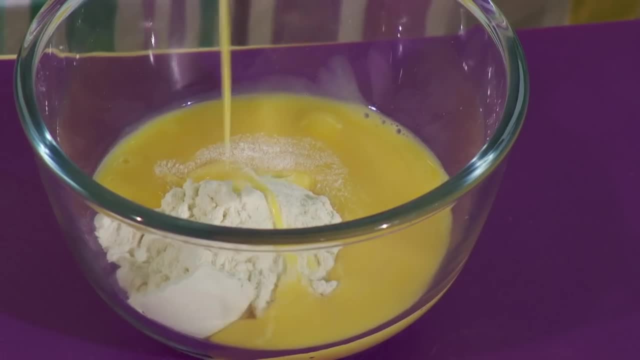 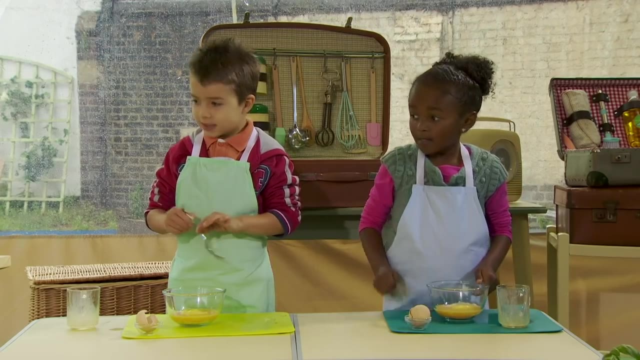 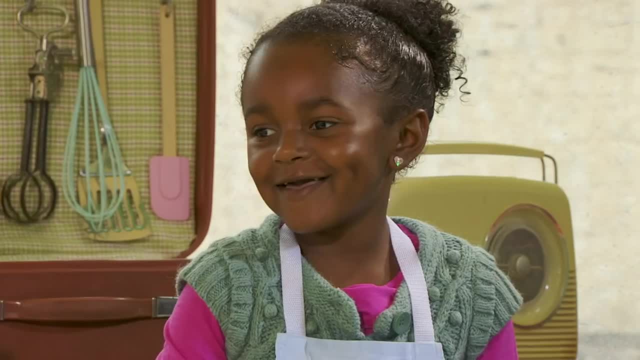 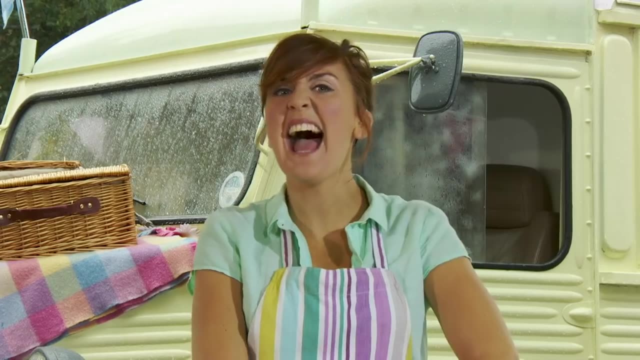 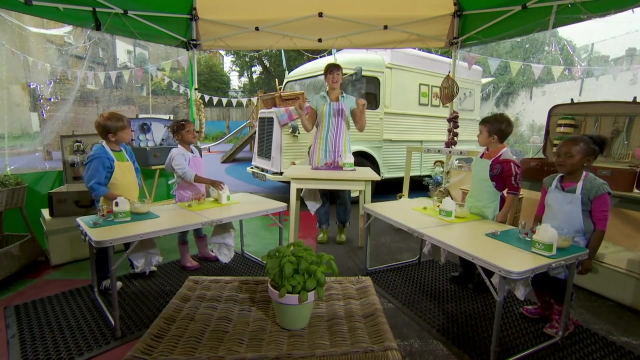 I'm mixing Mine's all gooey. Get right round the edges everyone. Next, we're going to measure some milk, And milk comes from cows. And what noise do cows make? Moo, And we are going to play the measuring game. Right, this is how you play One person's. 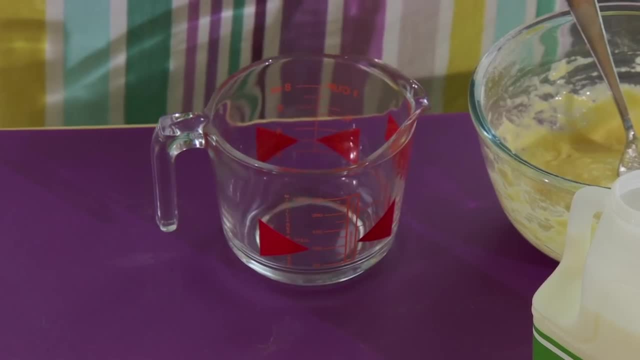 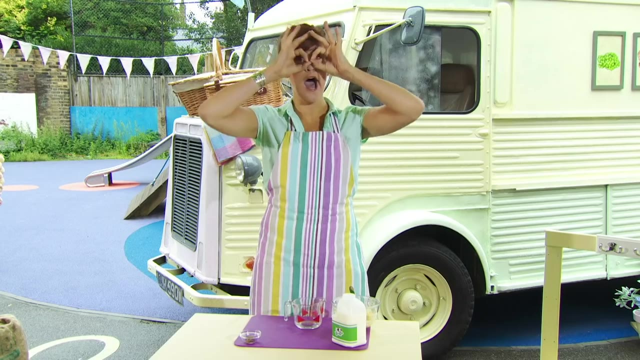 going to be the pourer And they're going to pour the milk And they're going to pour the milk into this jug, And then the other person is going to be the watcher And they have to put their watcher goggles on like this. 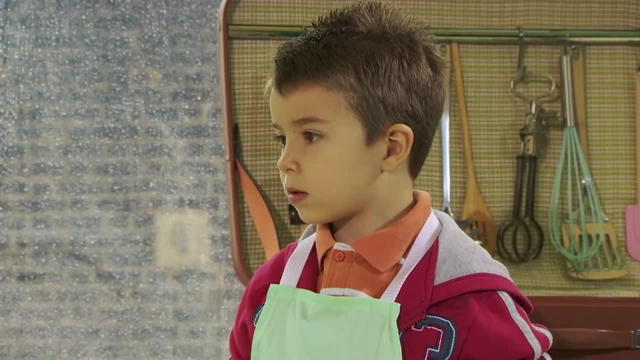 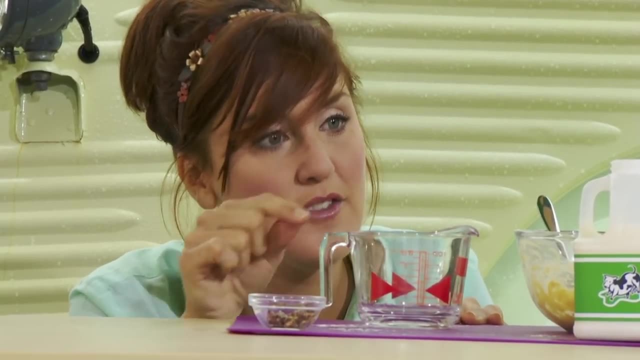 And the watcher needs to stay down low with the jug to make sure that the pourer fills it up to where the red marker is, And if they've put in too much, they need to tell them to pour a little bit out. Kajana, tell him when to stop. 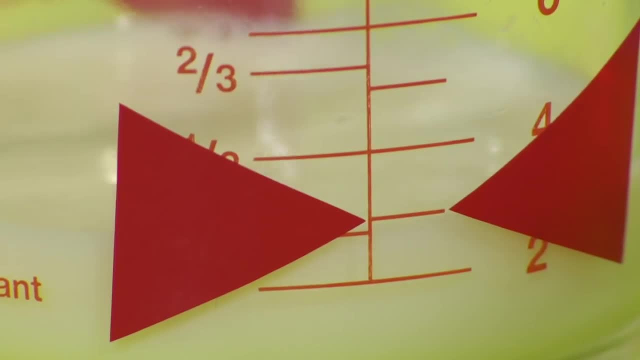 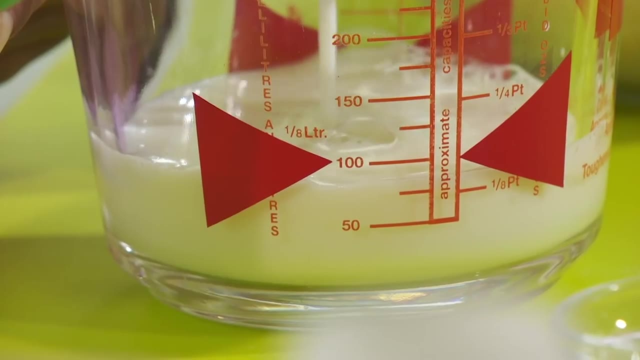 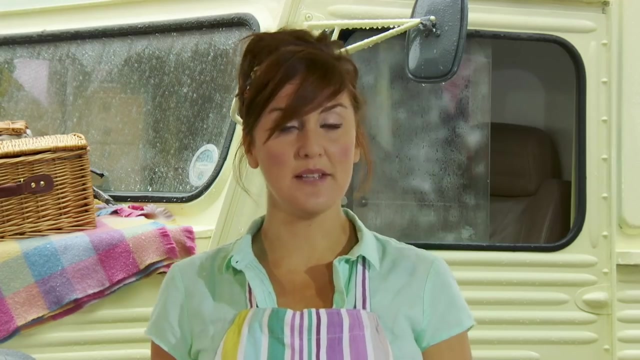 Go, go stop. Oh, good job, David. More, more, more, more, Stop. Perfect, What a good team you are. So now we've got our milk, We're going to pour it into our batter mix, which is in the bowl with a big splash. 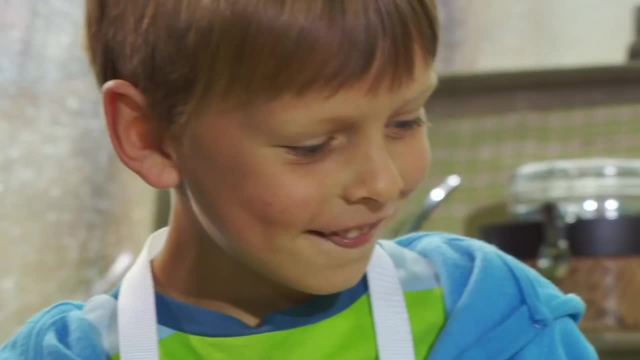 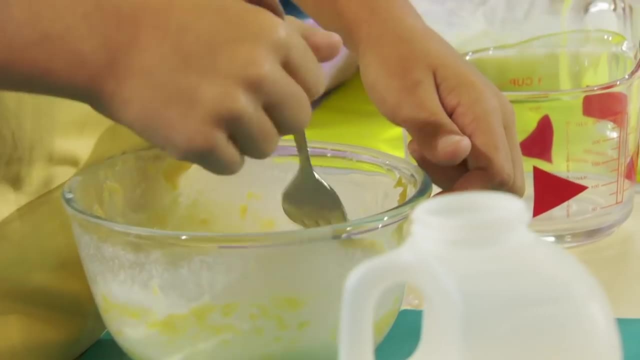 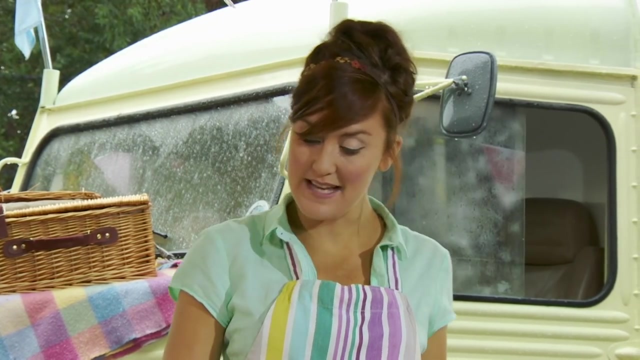 Splash. Wow, Oh my gosh, That's a cool mix. OK, let's give it a quick mix everyone. But we have to be very careful because the milk is very naughty And sometimes it escapes out of the bowl. We're going to add some flavour next And we're going to add whole grain mustard. 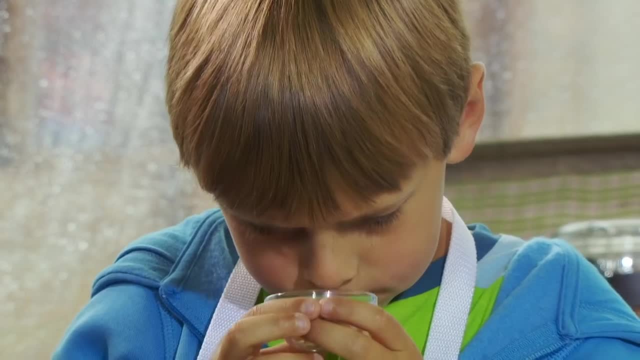 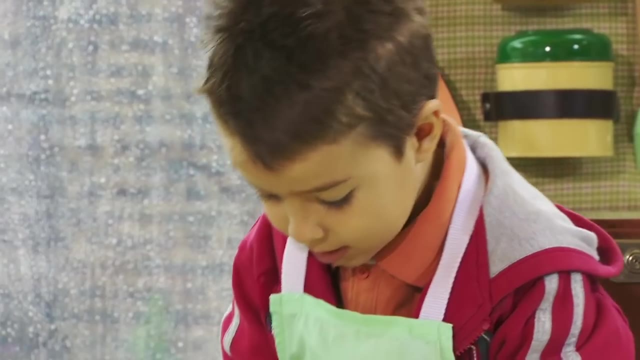 Can you see all the little bits in the middle, Loads of little mustard seeds? Now use your fork to scrape it into your batter. There we go. Can you see all the seeds swimming about? Yeah, Mine's going swimming. I think these seeds love having a good old swim, don't they? Harry? 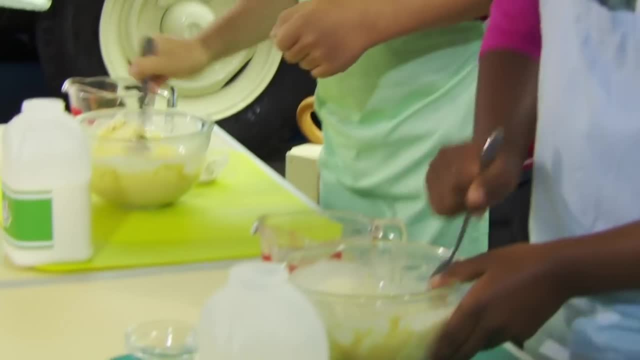 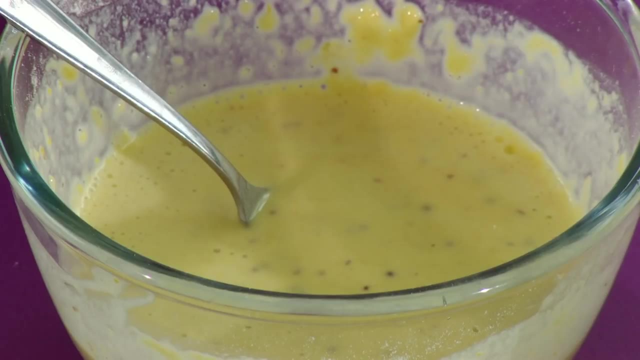 Keep mixing until we get a really silky, smooth batter. And that's our batter mix all finished. But I wonder what we're going to need next in our playtime popovers. What's next? Well, let us see if you can guess what it could be. 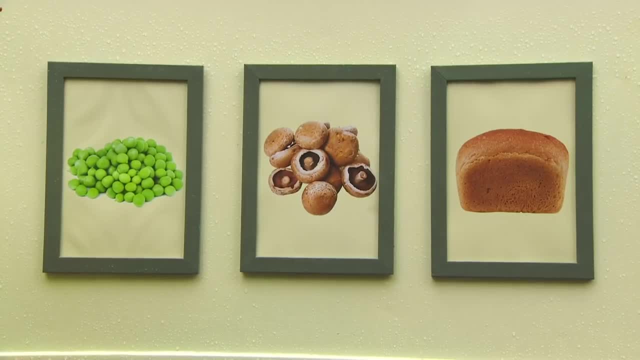 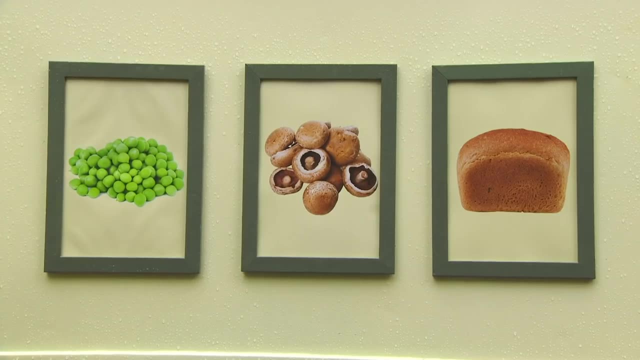 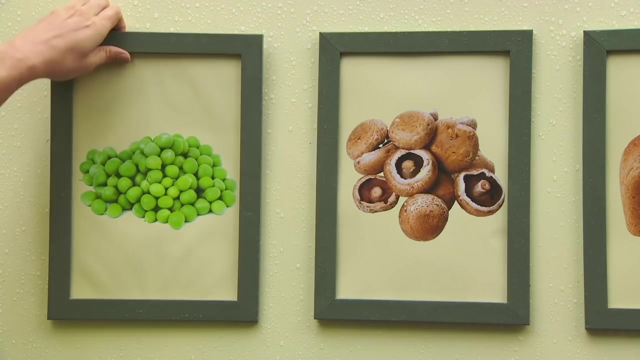 So we've got some peas, some mushrooms and a loaf of bread. What would you choose for our playtime popovers? The special ingredient can be white or brown Peas. They're green, so it's definitely not that one. Let's take that one away. There we go. 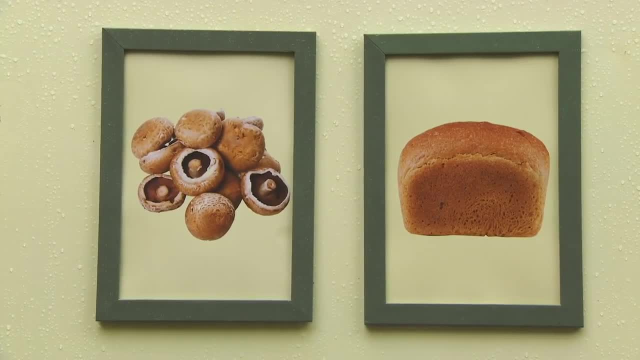 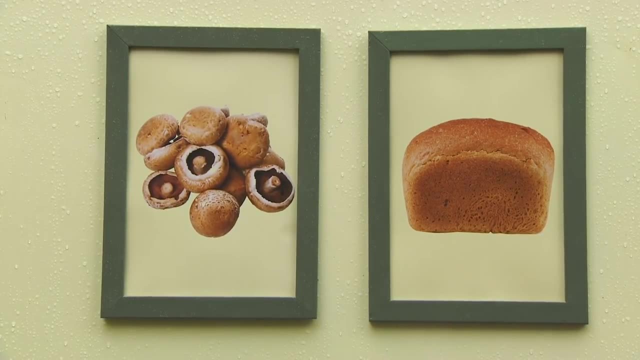 OK, here's another clue. So the special ingredient can be white or brown and it's in the shape of a little umbrella. Well, a loaf of bread can be white or brown, but it's definitely not in the shape of a little umbrella, is it? 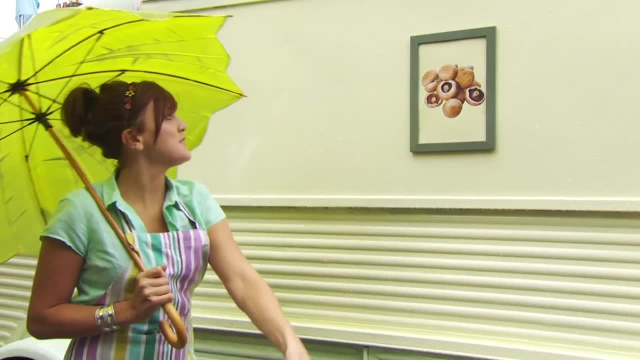 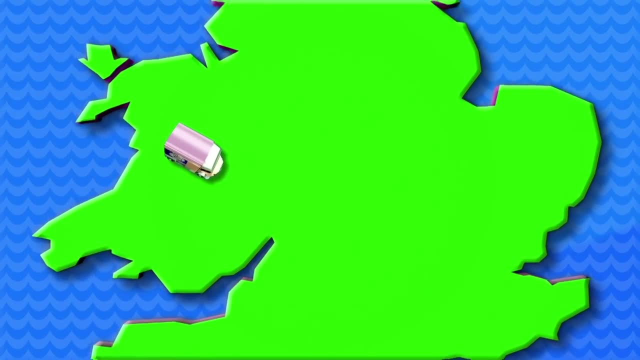 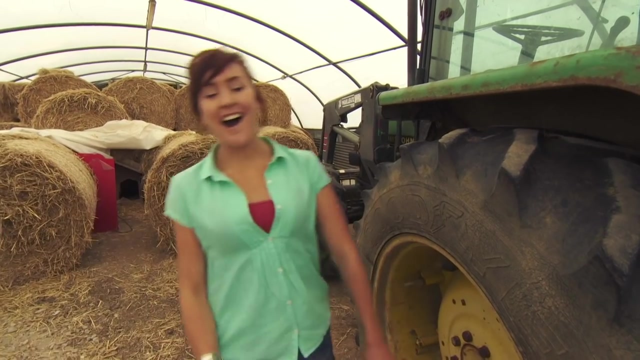 So let's take that one away as well, which leaves us with mushrooms. We're going to need some mushrooms for our playtime popovers And I went to find some. I'm at a farm in Northamptonshire to find some mushrooms. 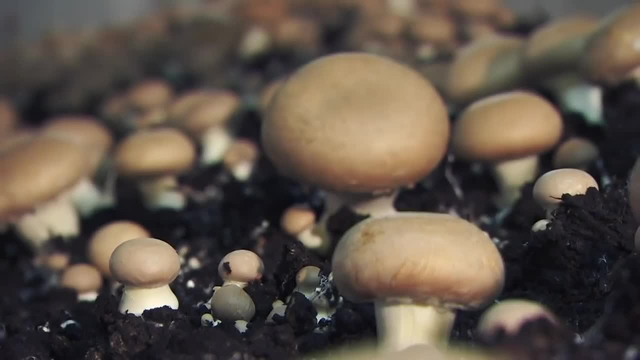 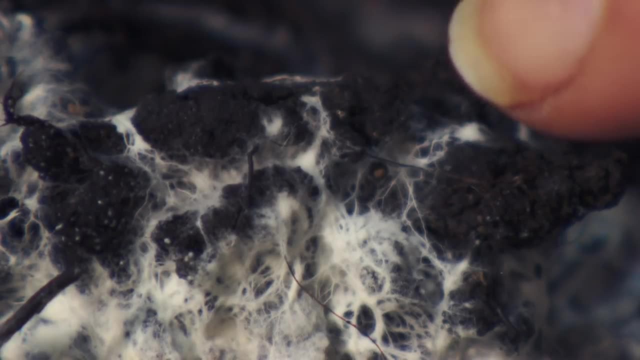 So let's go on a mushroom hunt. Mushrooms grow from millions and millions of little things called spores. The spores start growing and huddle together to make the head, To make the head of the mushroom which is called the pin. 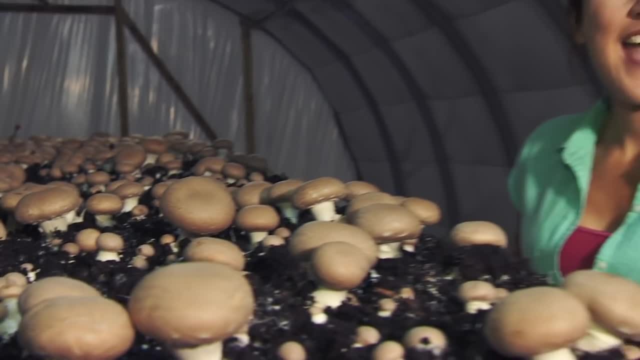 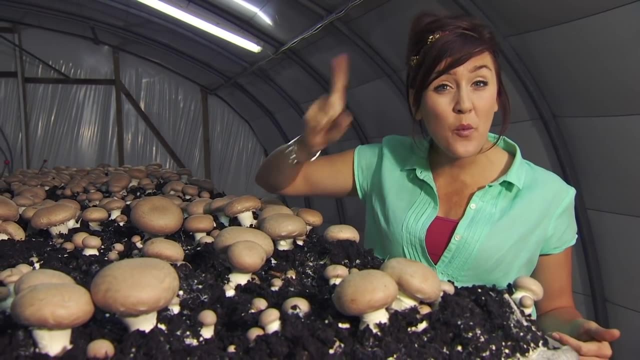 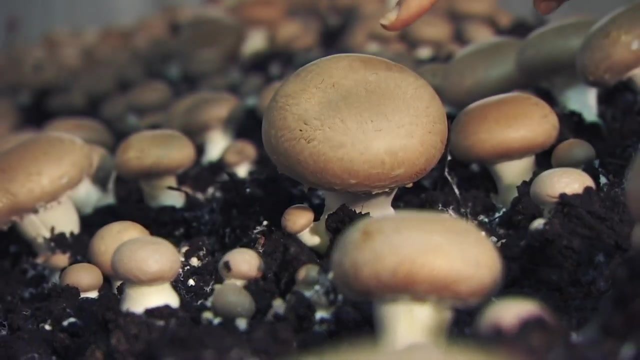 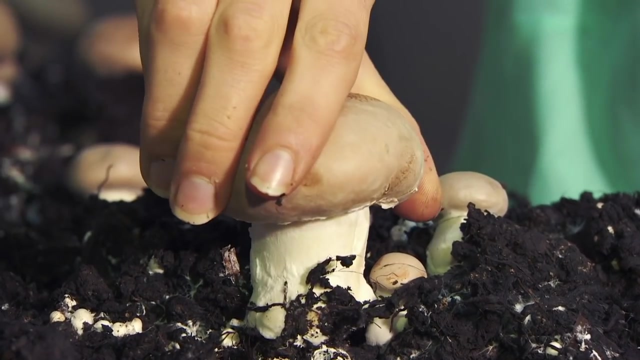 And you can see it just here: The mushrooms can grow from this to this in less than one week- How amazing is that? And you can pick them when they're small, medium, and when they're giant, like this one, You just have to twist and pick. 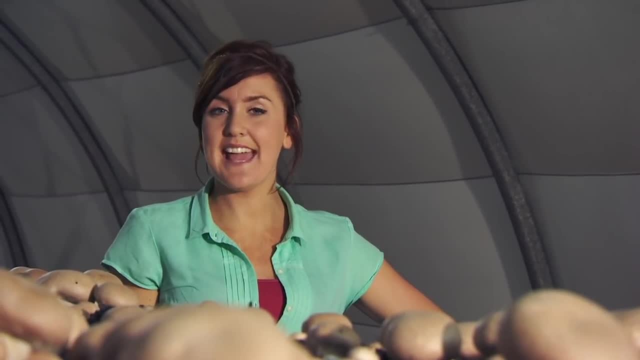 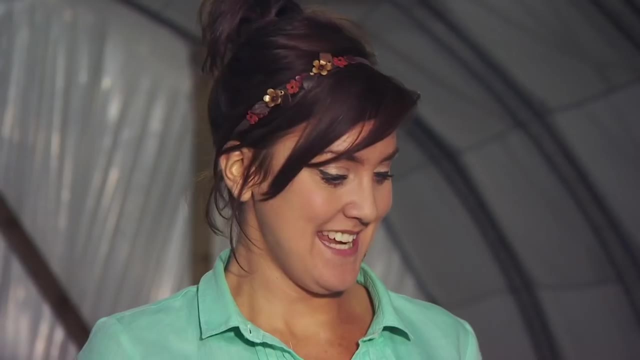 Now, you can't eat all mushrooms so, to be safe, only eat mushrooms that you get from the shops. We just need to give these a wipe and then they'll be great to use in our playtime popovers. Mushrooms are a really funny shape, aren't they? 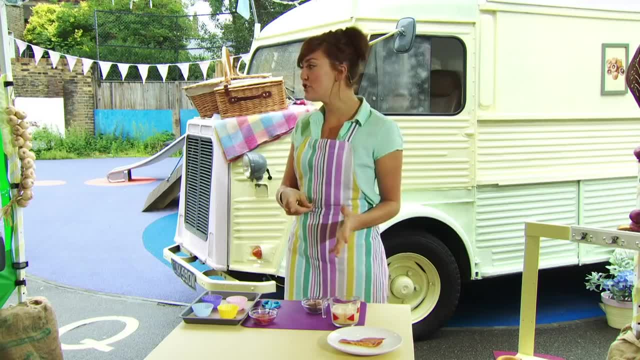 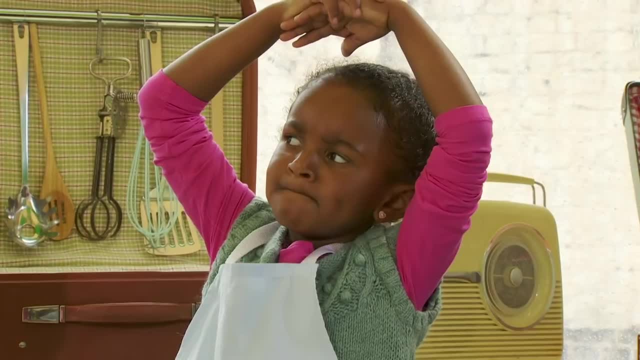 Look, Don't they look funny. Oh, who can do a mushroom face? We go like this and go: Oh, brilliant mushroom face. Now we are going to play the break and flake game with our mushrooms, And you play it by doing this. 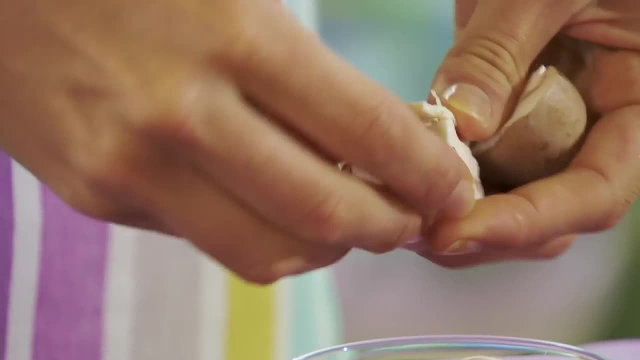 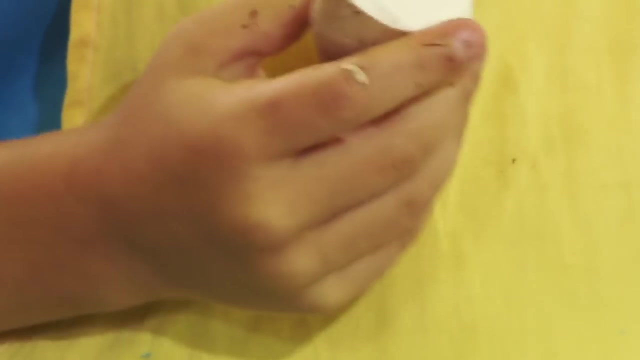 Look, Break and flake, Break and flake. Who can do that? Me Off. you go, then Break and flake, And again We're going to do the break and flake, The break and flake. Now we need to sprinkle a bit of mushroom. 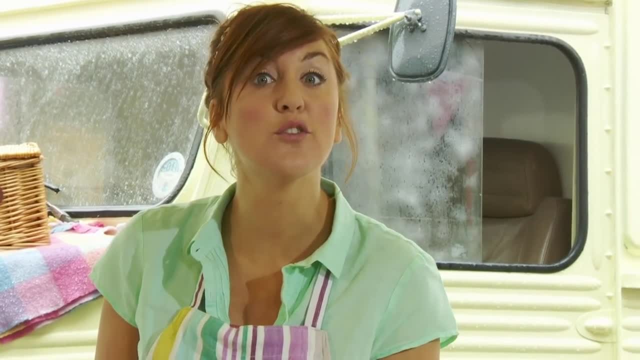 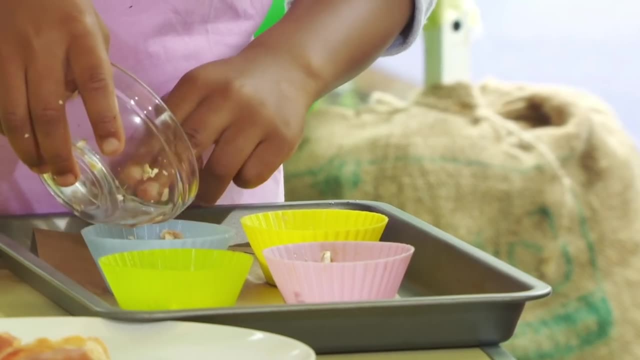 into each of these muffin cases, which I've already oiled for you. So sprinkle, Ooh, Sprinkle. Mushrooms are good for you, Yes, they are. Next, we're going to snip up some cooked bacon. 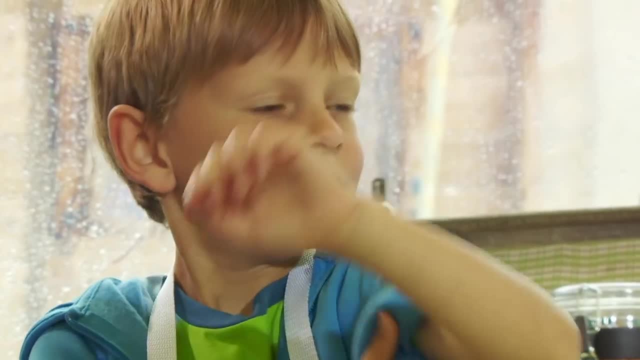 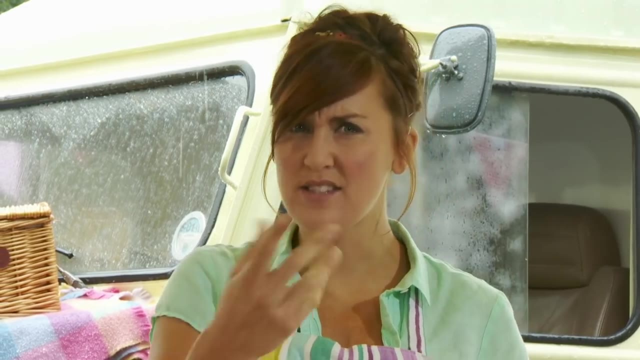 Who likes bacon, Me? Now, if you don't like bacon or if you don't eat it, you can just use something else, like spring onions or chives. That would taste really nice as well, But we're going to snip up our bacon using scissors. 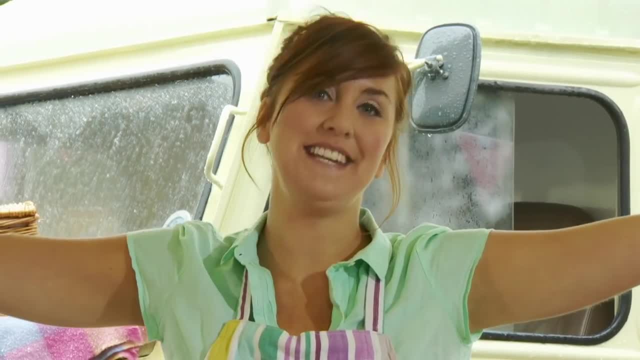 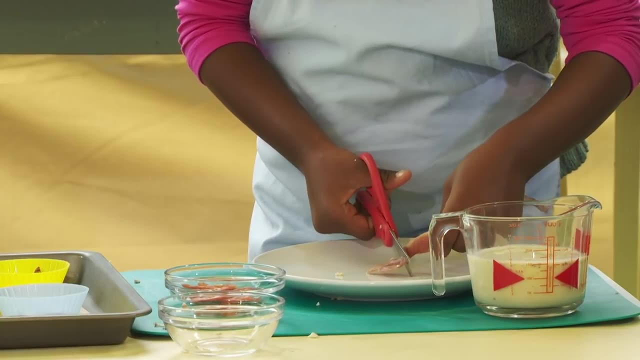 But remember, be safe with scissors. Everybody knows that we need to point them down towards our Toes. Toes One, two, three. Let's get Snipping, Snip, snip, Snippity, snip. 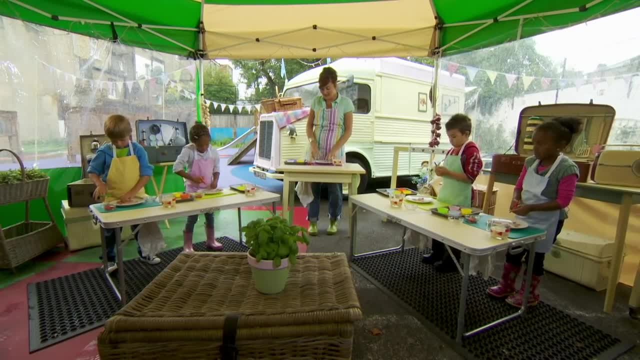 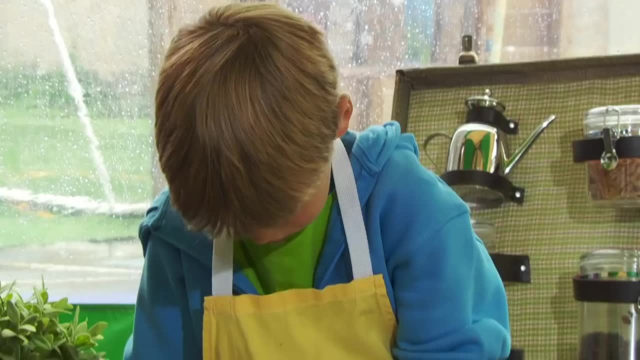 And once you've finished snipping, you can put your cooked bacon in with your mushrooms. Lovely, jubbly, Jubbly, Jubbly, lovely. I don't have any more bacon now. Next, we're going to add some colour. 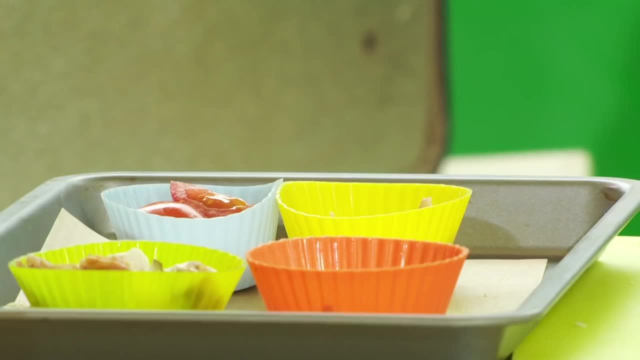 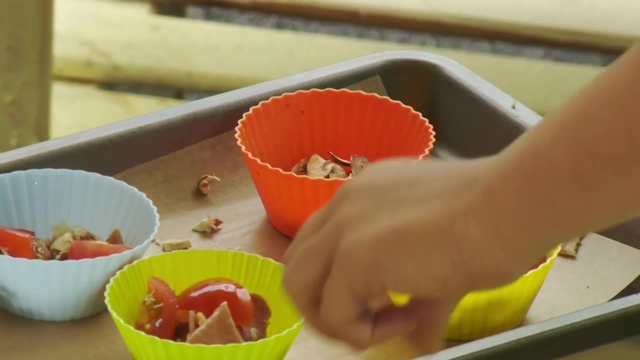 We're going to add some red chopped up tomatoes, So let's put some tomatoes into our cases too. Or one tomato for me. One tomato, two tomato. These are like the little cherries on top of the cake. Yeah, I've got the tomatoes on my cake. 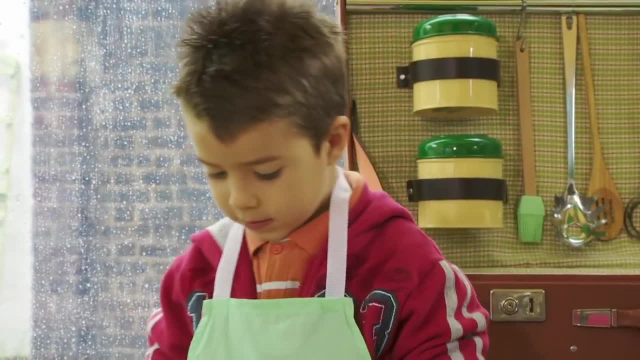 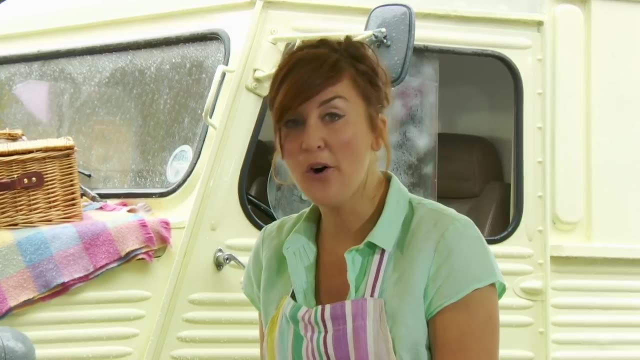 Hey tea, These are going to be so tasty. Has everyone done that? Yeah, We are going to pour the batter mix that we made earlier on into our muffin cases, and all of the ingredients are going to disappear. Are you ready? 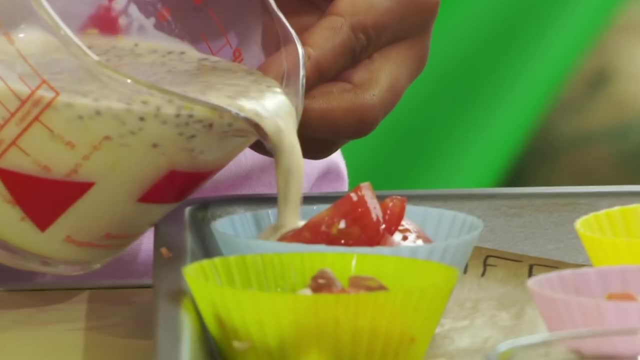 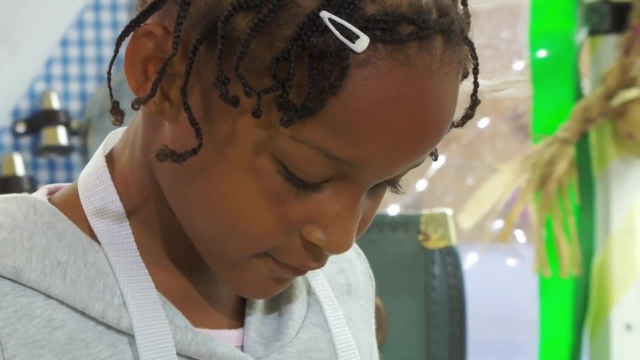 Go OK. when you've filled up your muffin cases and all of the ingredients have disappeared, that's when you need to stop. That's it, That's enough, And then do the next one. I'm not done, Emily. 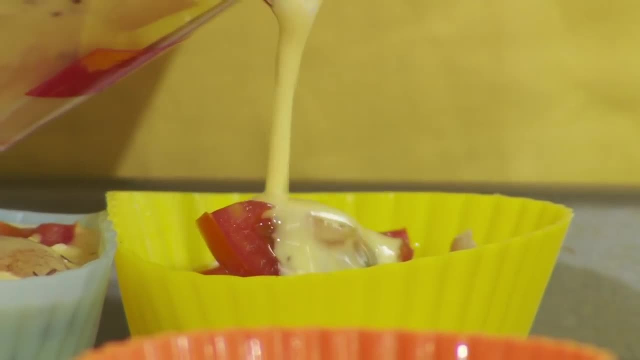 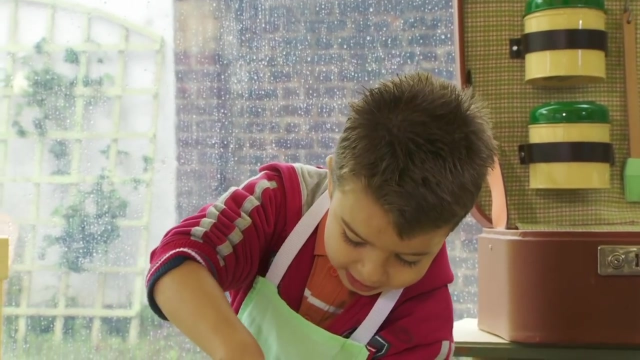 Stop Whoa And don't worry if any of the ingredients are sticking out of the top, because they're going to go really crispy when they go in the oven later on. Go on, dig out. Hey, mine's almost covered. They look like cakes. 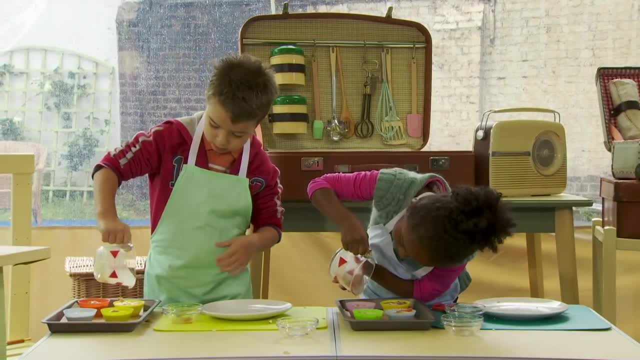 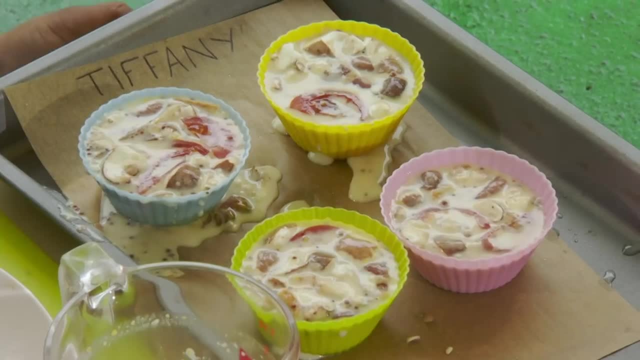 Let's make sure we get every last drip in. This is my last drip in And that is it. team, You've done it. You've put all the ingredients together for your playtime popovers all by yourself, And now it's time to put them in the oven to cook. 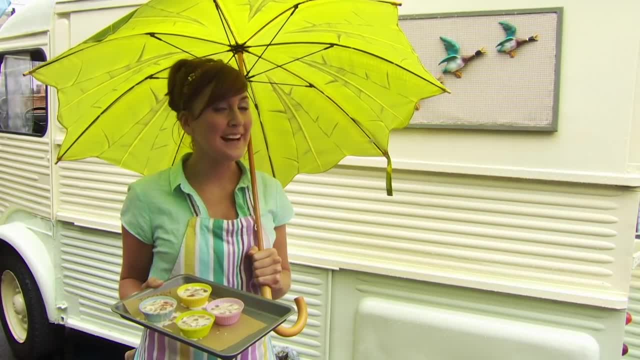 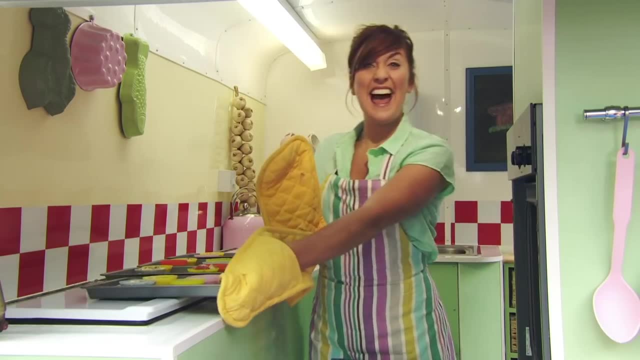 But remember, ovens are hot, so don't go near. Ask a grown-up to help you here. Now we've cooked with you and had lots of fun. Let's tidy up and think of all the things that we have done. There was. 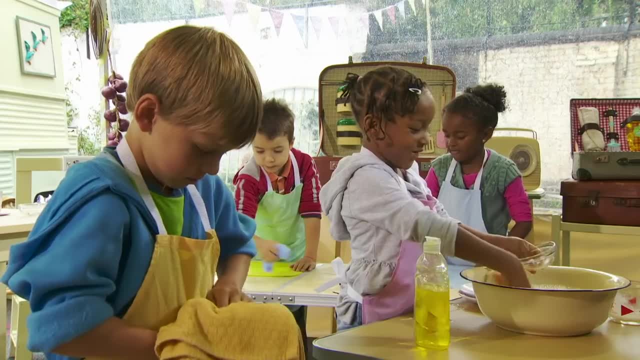 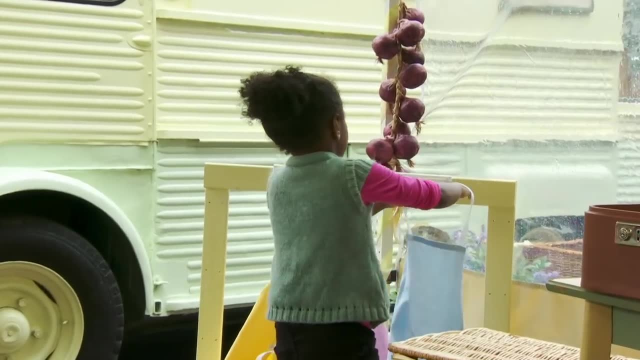 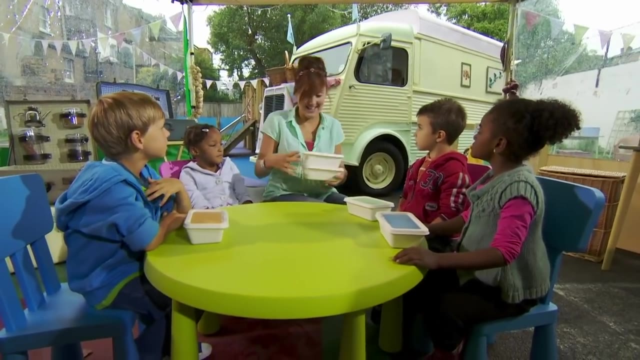 Whisking, Snipping, Cracking And Making any mess And putting things away. It's always fun to do. At the end of the day, All right, everyone. here's our food and it's all ready for us to have a look at. There's yours, Tiffany. 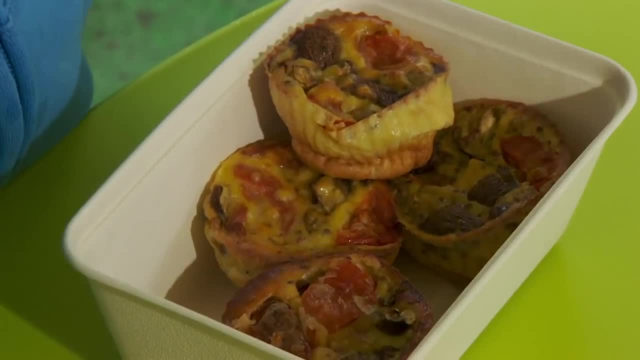 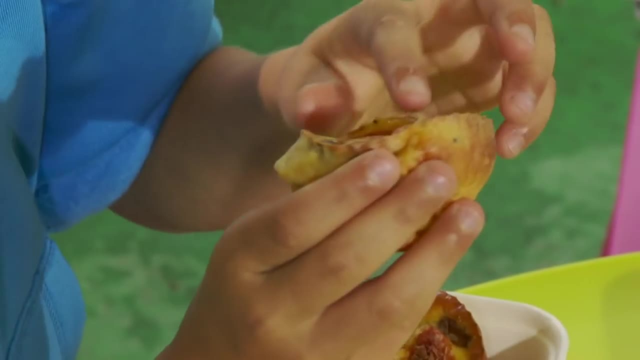 Let's have a look at Harry's. Oh yes, nice Harry. What's actually happened to the tomato in the oven, Harry? It's just gone all crispy. I've got an alien with one eye And two nose. 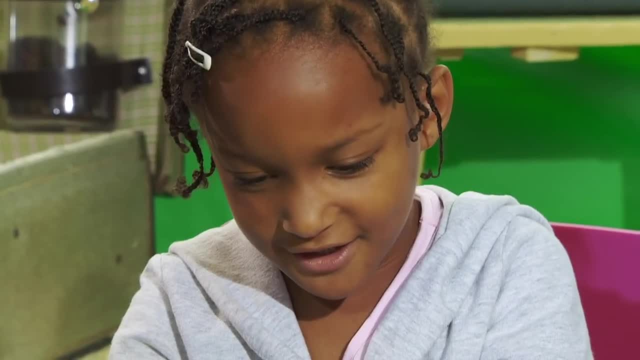 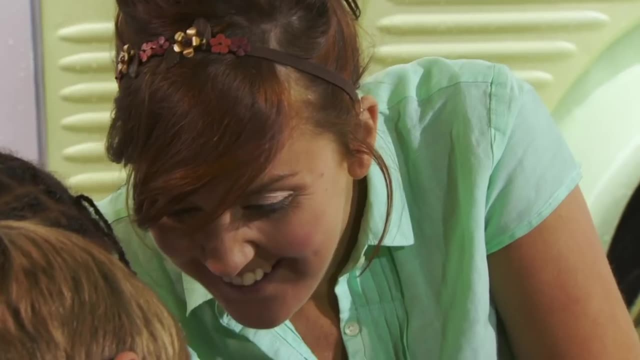 Let's have a look at Tiffany's. Oh, they're soft. Yeah, what were they like before? All gooey and wet? Yeah, look at his happy face. Oh, yeah, look, there's the eyes and the nose and the mouth. 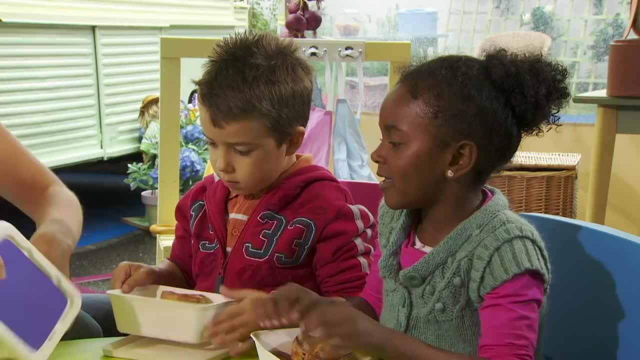 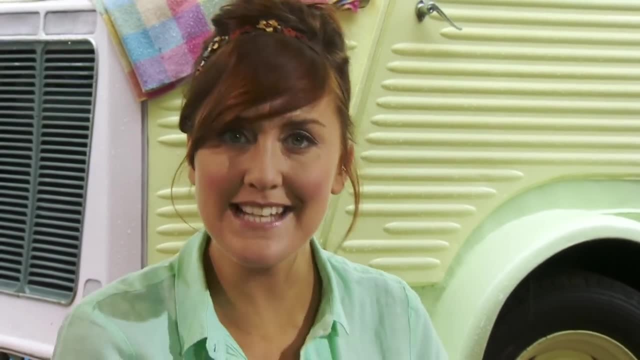 And it looks like a muffin too, And a mini pizza. Right, let's put the lids on everyone and save this for later. We've travelled to you, we've cooked and had fun. Now let's have a party with everyone. 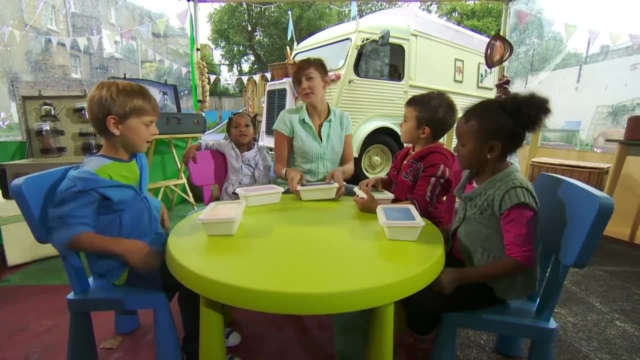 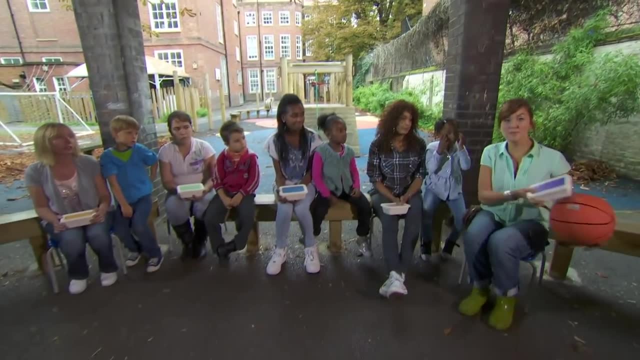 Yay, Come on, team, let's go, And you can come with us This way, This way. Well, I can't wait to have a game of basketball, but let's eat our food before we play. We've done the breaking flick. 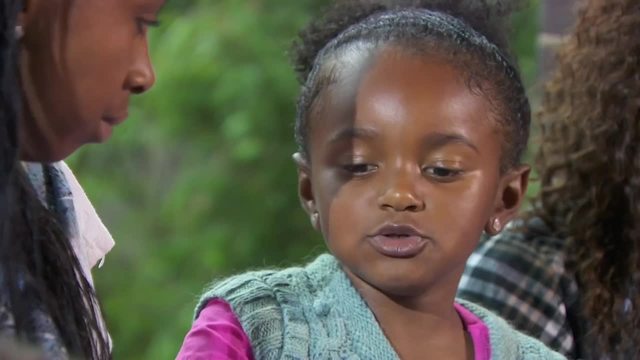 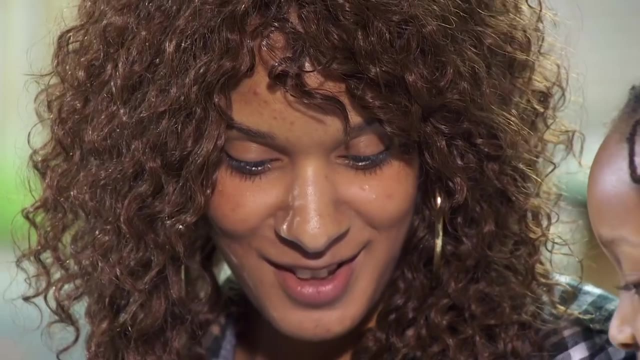 What's breaking flick? How did you do that? You just take something and you squish it on your hands. Wow, that's fantastic, That's really good. Look what I made. Wow, Mmm, that smells great. What is it? 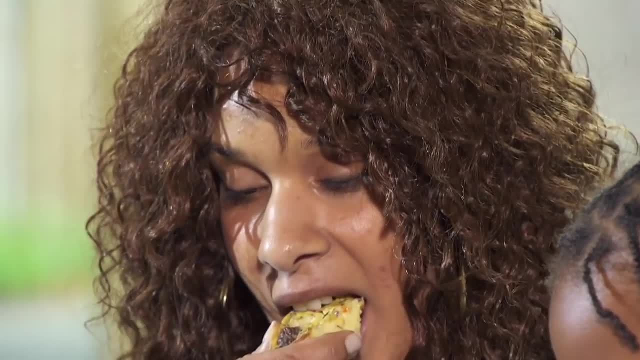 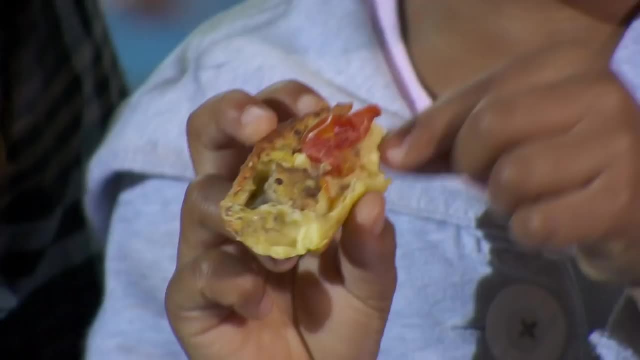 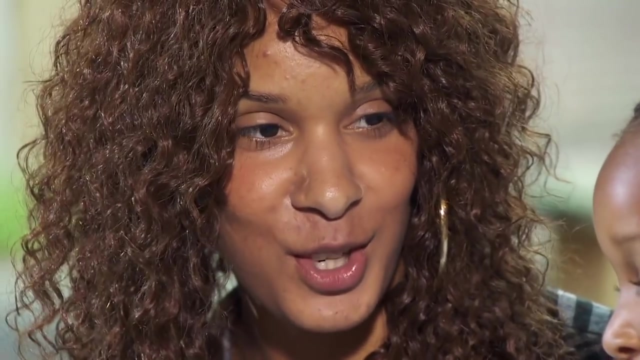 Playtime puffer. Mmm yummy, Here's a piece for you. Mmm, Oh, it's got mushrooms in it. We put egg, milk, flour. You made it all by yourself. Yes, They're delicious. They're really really nice. 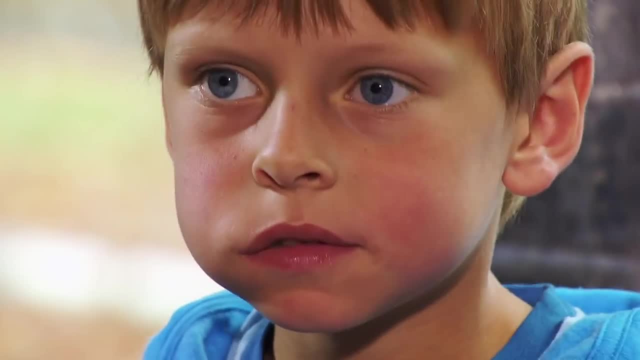 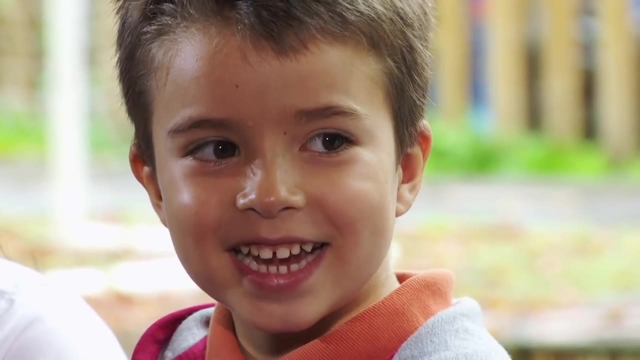 Mmm, it's nice. So, David, what other ingredients do you think we could put in our playtime popovers? Sausages- Yes, sausages would be delicious, wouldn't they? Yeah, Harry, what else would you put in it? 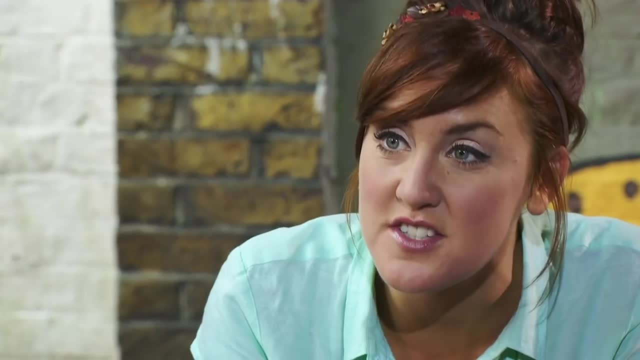 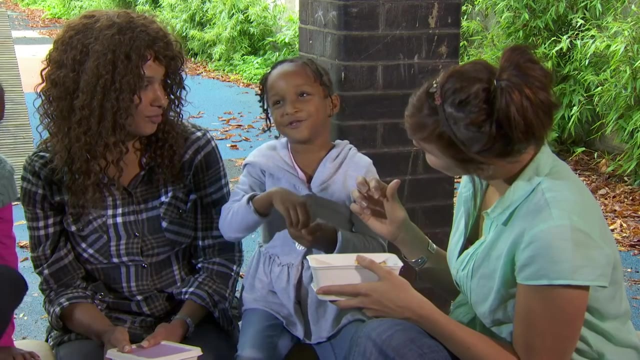 Beans. What baked beans. Actually, that would be nice on the side, Wouldn't it? What are you gonna cook next time? I'm gonna make a big white cake, And what flavour's the cake going to be? Strawberry flavour. 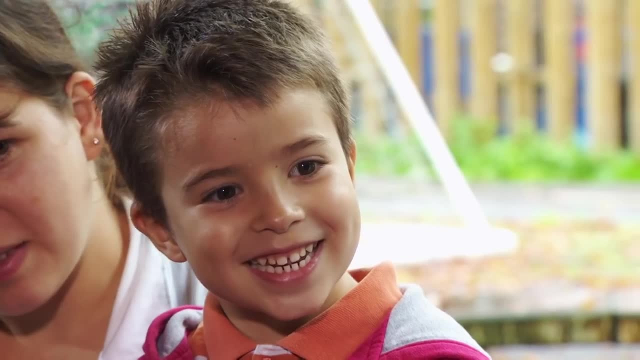 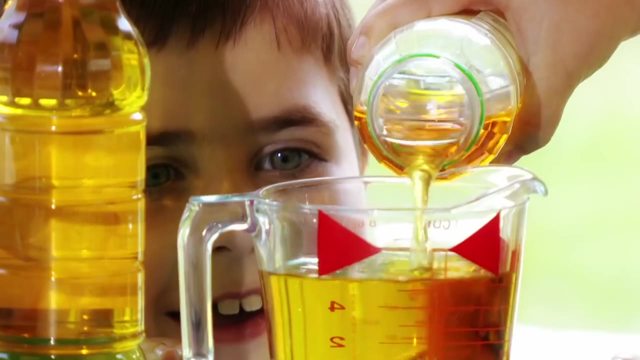 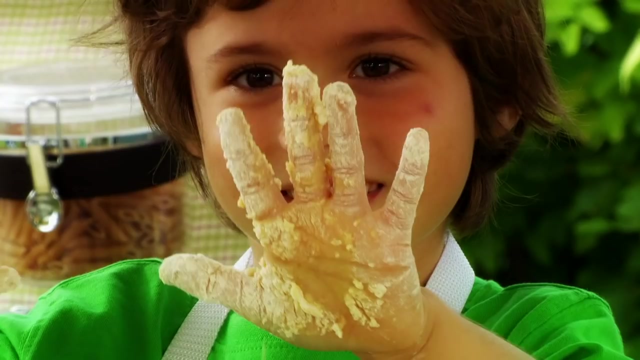 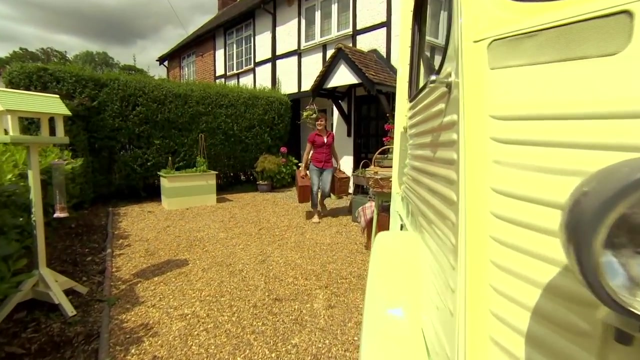 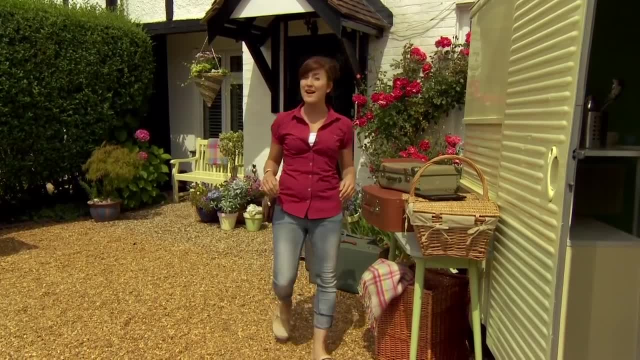 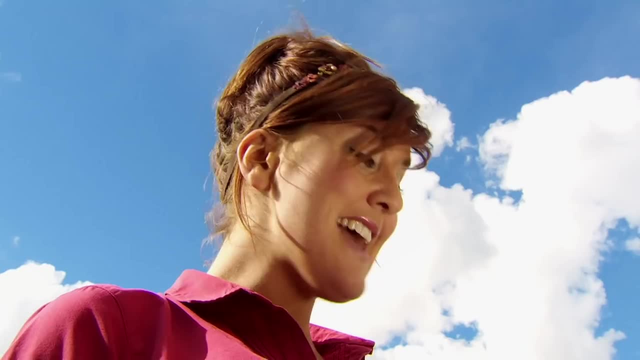 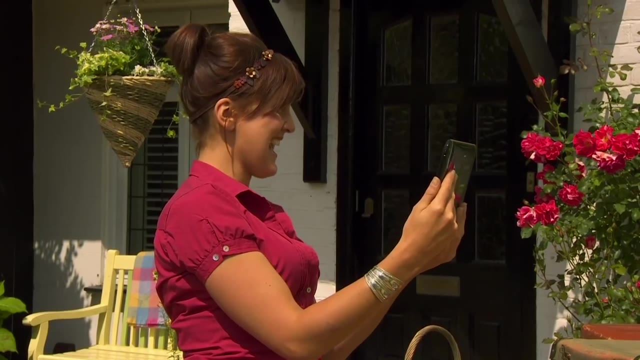 and I hope that you're going to come too and meet some new friends. Aha, Katie, can you cook with me please? Definitely That will be so much fun. Please help us make sight with Carrot Turf camping. I can, and you can cook with me too, and I love getting outdoors. 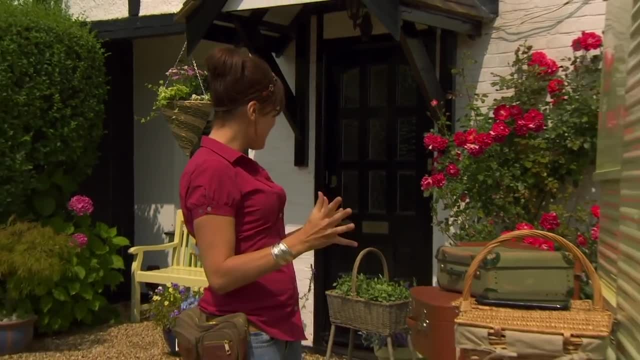 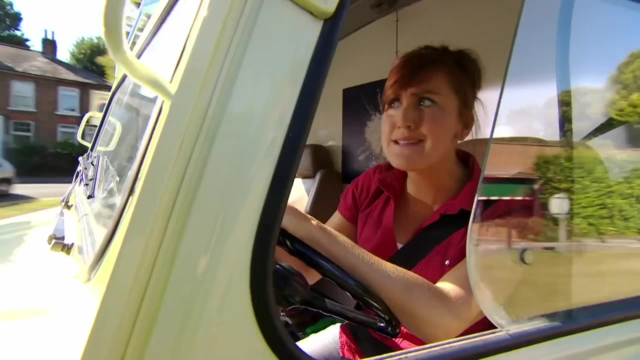 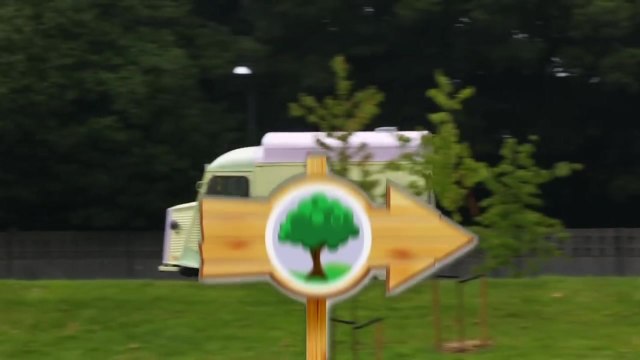 and doing some camping. That will be great. We just need to get everything packed up and then we can get on our way. All for the journey, and I'm coming to you. It's going to be busy and there's lots to do. Get ready to help, join in and have fun. Let's cook a feast for everyone. 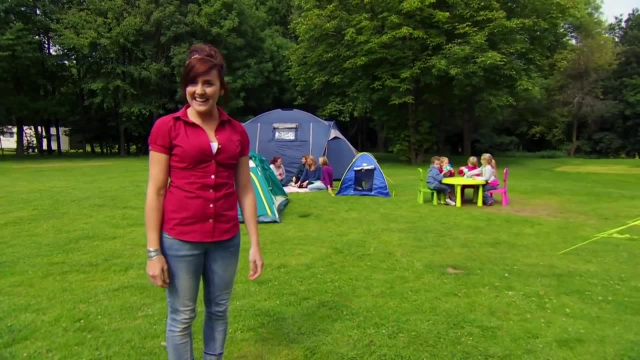 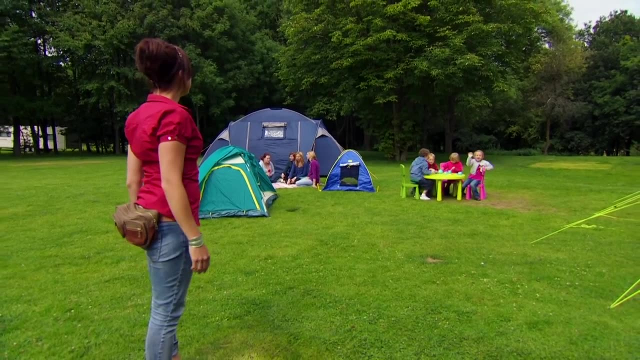 Well, here we are at the campsite where I've been invited. I'm invited by Caitlin. Oh, look, there she is over there with all of her friends having a tea party. Hi everybody, Hi Caitlin, Hi Caitlin. Great to meet you, Caitlin. Are these 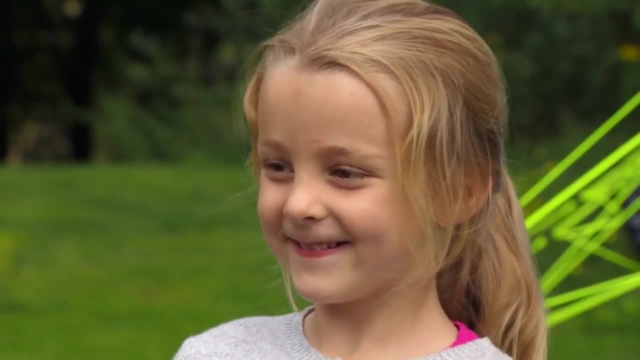 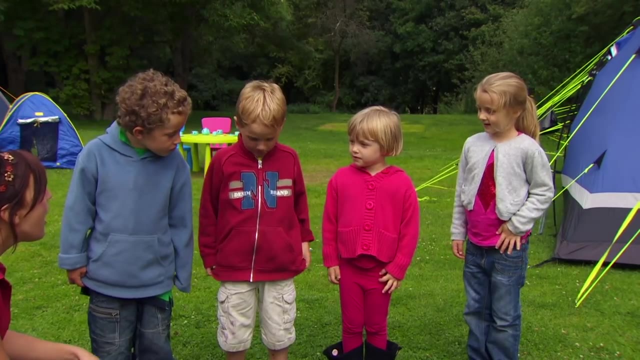 your friends. Aha. So what's your name? Olivia, William, Frankie. So, Caitlin, tell us all what we're going to do today, Make sight for when we're camping. Brilliant, because I have got such a fantastic recipe to cook with you all. 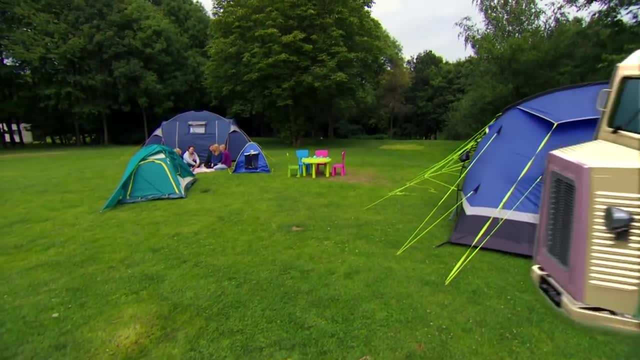 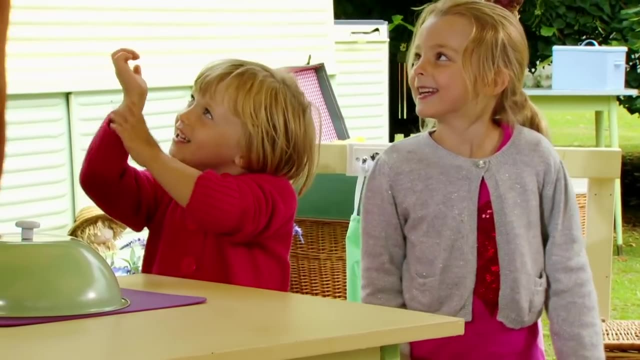 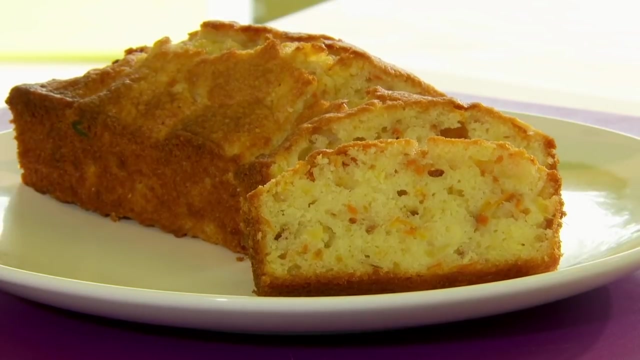 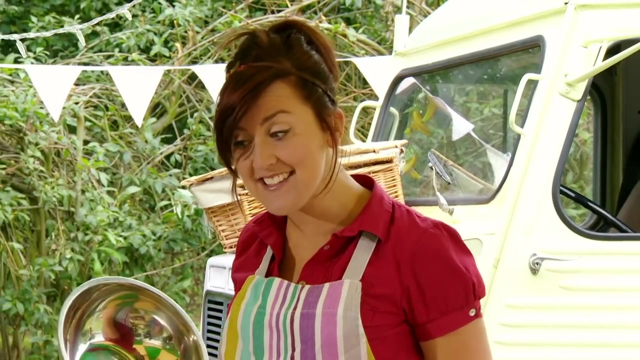 Quickly follow me. Welcome to my outdoor kitchen. Now. who wants to know what we're going to cook today? Today's recipe is Sunny Carrot Cake. Mmm, That's delicious. We'll get to have some, don't worry, William. 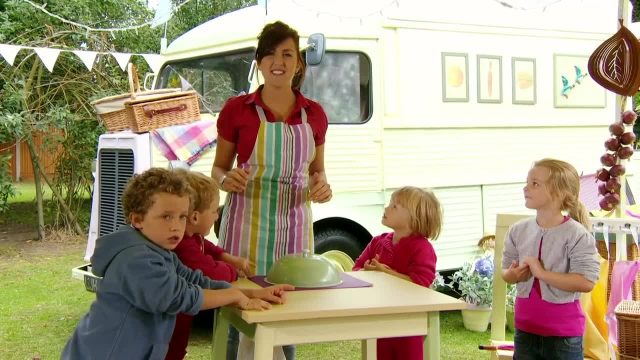 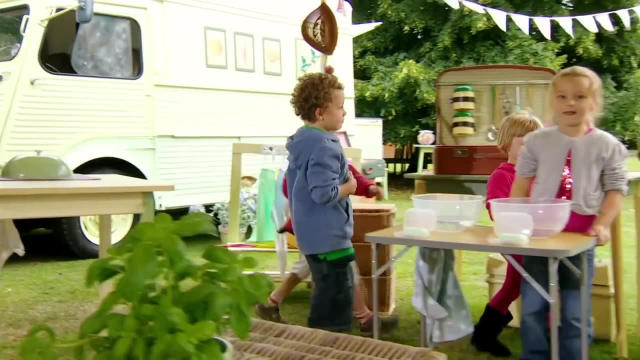 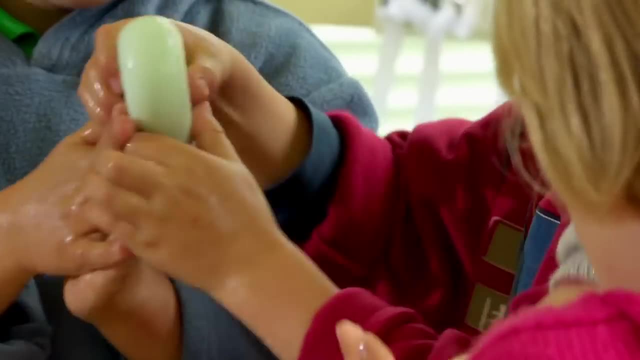 But before we get started on the cooking, we've got to do something first. What do you think it is? Wash our hands. Wash our hands, That's right. Let's get going. everyone. Roll up your sleeves. Give your hands a wash With slippy dippy soap. Splish, splash, blosh. 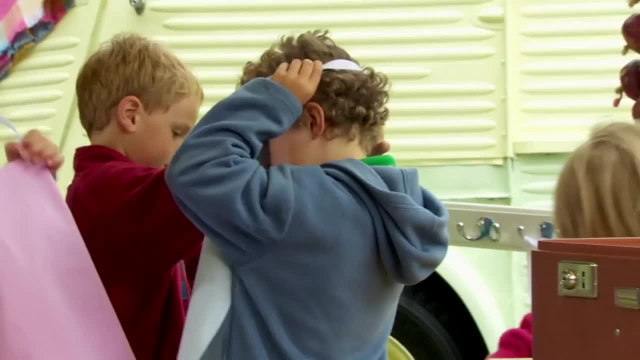 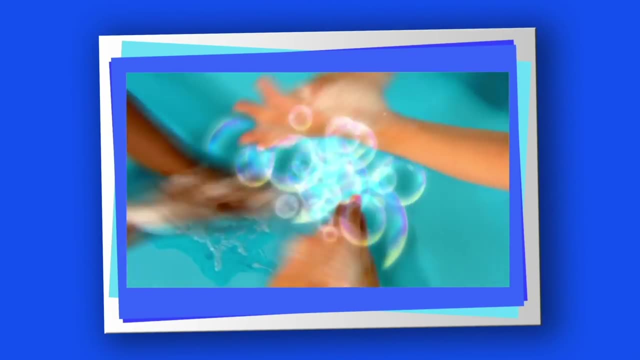 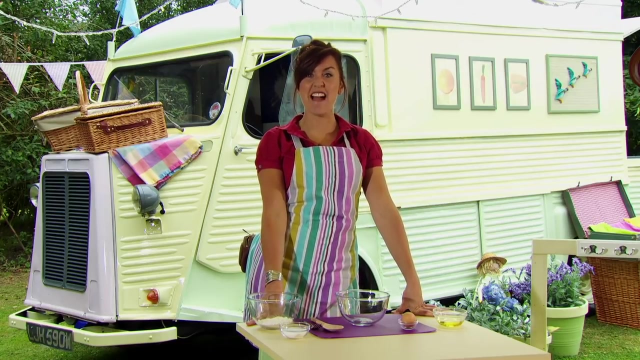 Have you done? your hands Washed and dried, Sleeves rolled up, Apron tied. What can you do? I can cook. Let's get started Now. the first thing we have to do to make our Sunny Carrot Cake is crack an egg. But 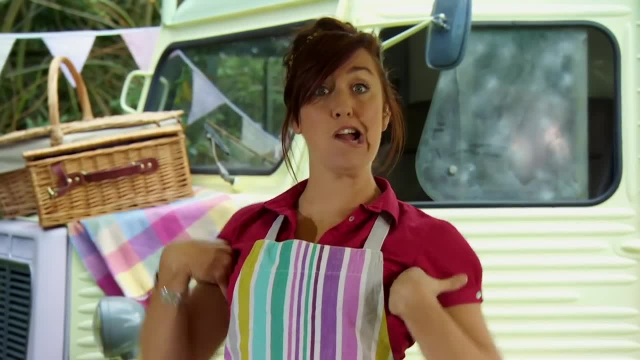 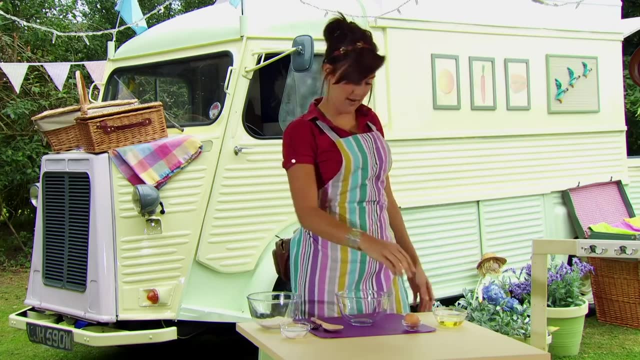 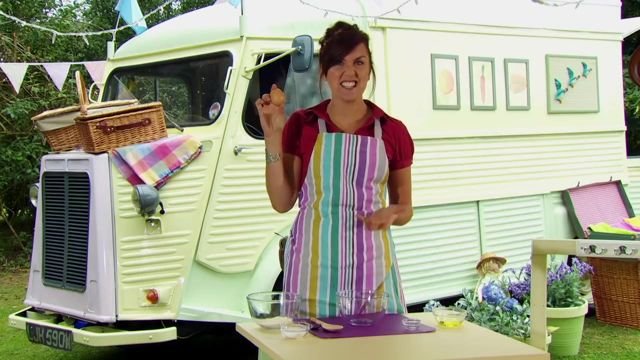 wait, What animal do you think? this is Chicken. That's right, It's a chicken, And that is exactly where an egg like this comes from. But eggs can also come from other animals like ducks or ostriches. Now we are going to crack. 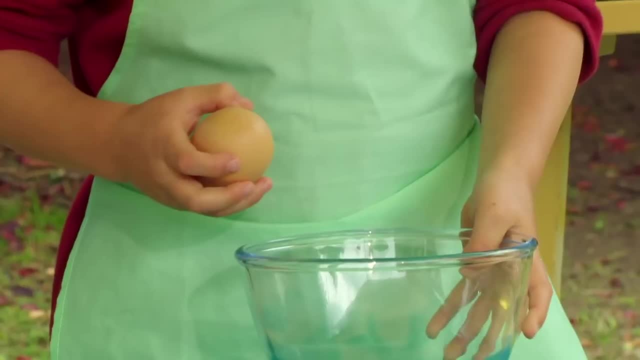 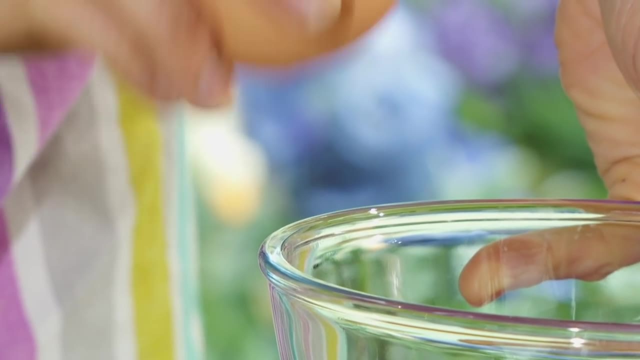 this egg into our bowl. Why don't you join in with us? First of all, we have to knock on the door of the egg like this: Knock, knock, knock, knock, knock And open sesame. Go on, Caitlin. Yes. 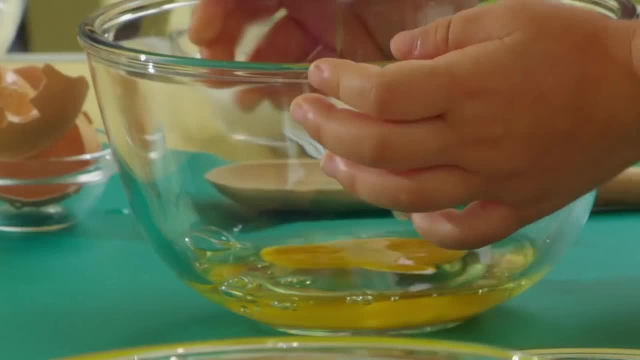 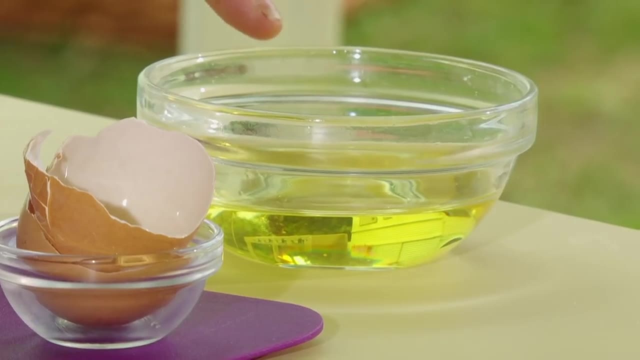 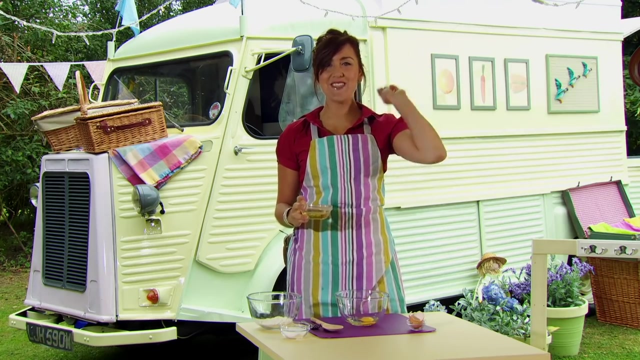 That's amazing. Okay, let's give our hands a little wipe, because they're a little bit eggy. Next we need to add some vegetable oil, which we have just over here. So let's pour that in with a big splosh Splosh, And you can splosh with us. One, two, three Splosh. Wow, look What's happened. 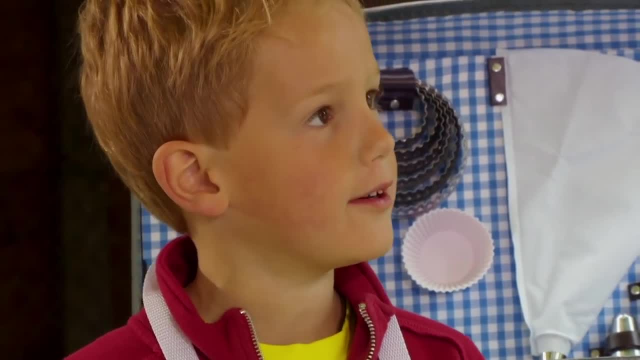 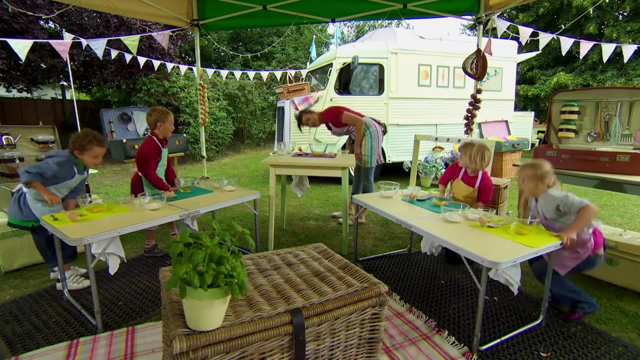 to the egg and the oil Bits round the egg is turning gold. Is that because of the oil? Yeah, Mine's gold. And it looks more gold if you look from underneath, Does it? Let's all have a look like that then? 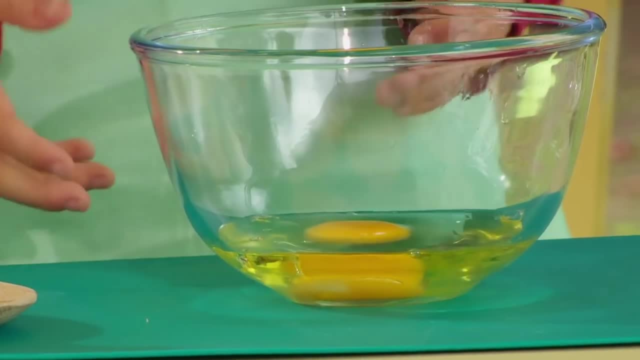 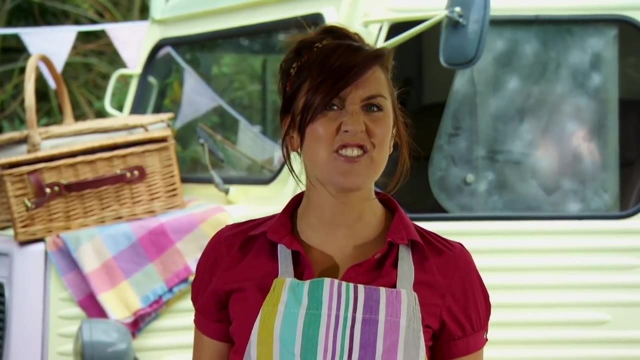 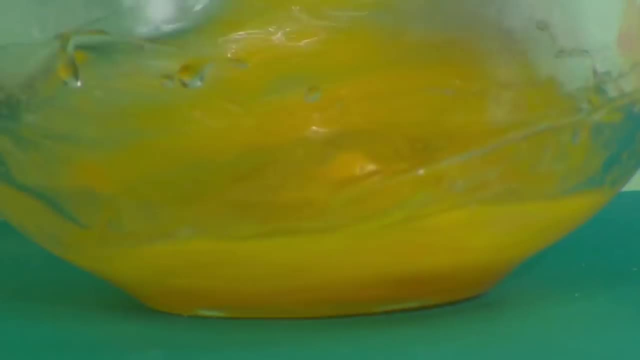 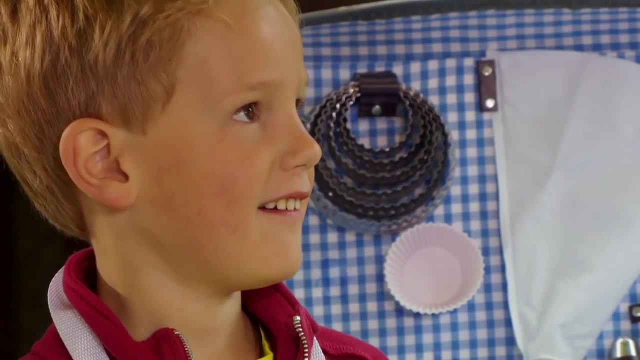 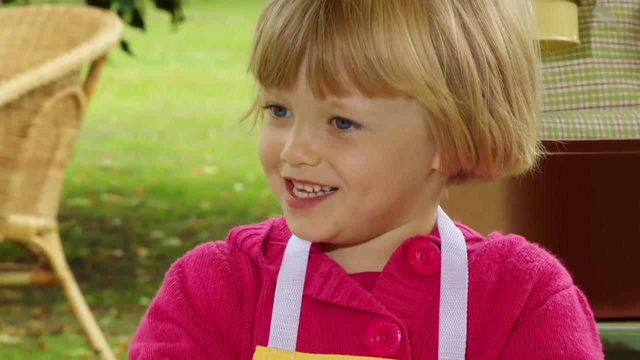 beep, beep, beep, beep, Whisk Going yellow. It's the same colour as spaghetti. It is actually, isn't it? It's the same colour as spaghetti. Okay, everyone press the stop button. Beep, There we go. You can put your fork down on your mat. Now I want you to swap this bowl. 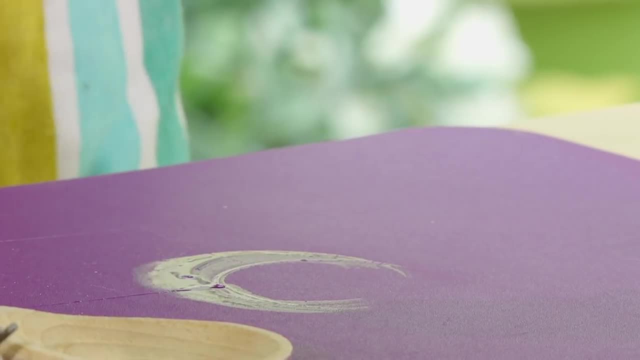 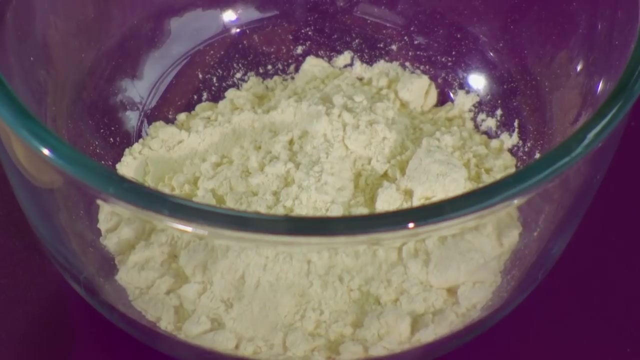 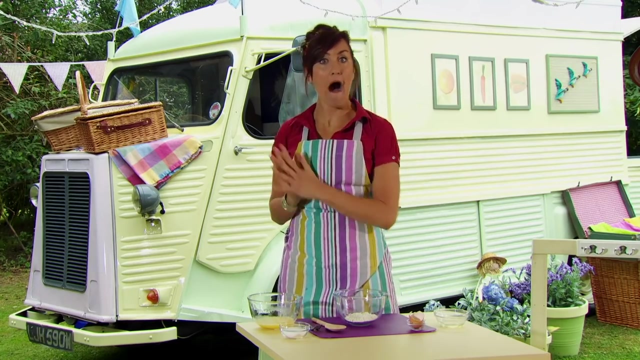 with the bowl of flour. Now this is your dry bowl, and the other bowl is your wet bowl. Now, in this bowl, we've got some self raising flour. And shall I tell you a secret? Self raising flour is magic. That's right, because when we put it in our recipe, it's going to 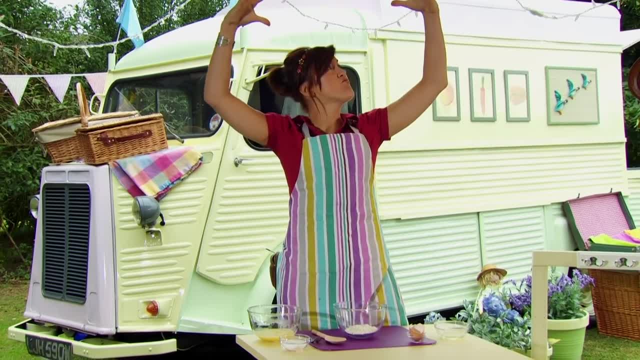 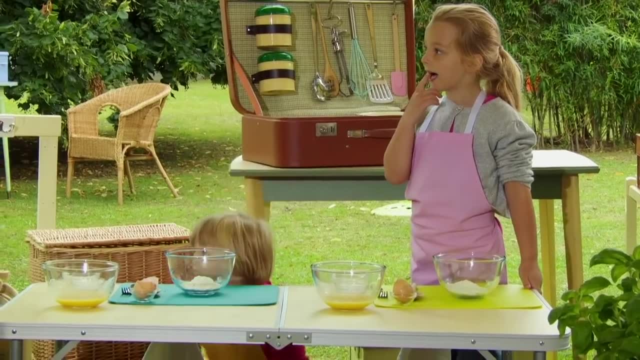 make our cake rise up really big when we put it in the oven later on. Shall we pretend to rise up like the cake in the oven. Yeah, Okay, why don't you join in with us? We start really small and then we pop. Shall we do. 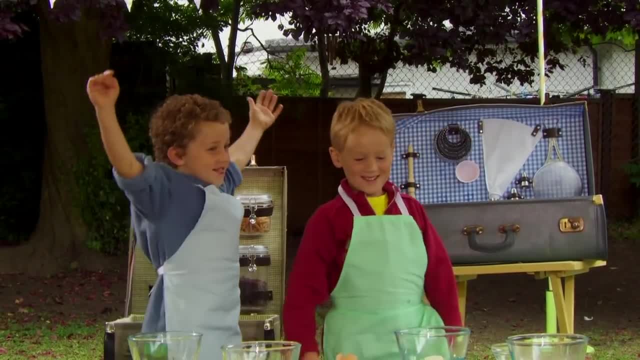 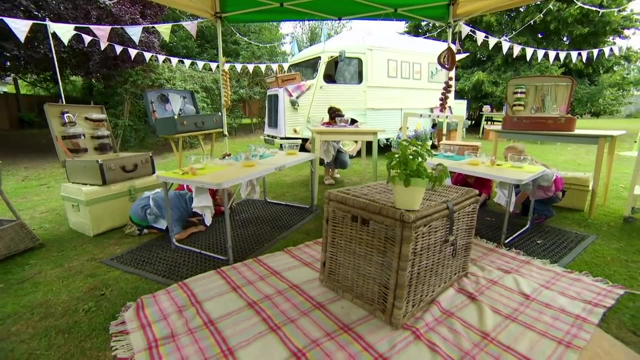 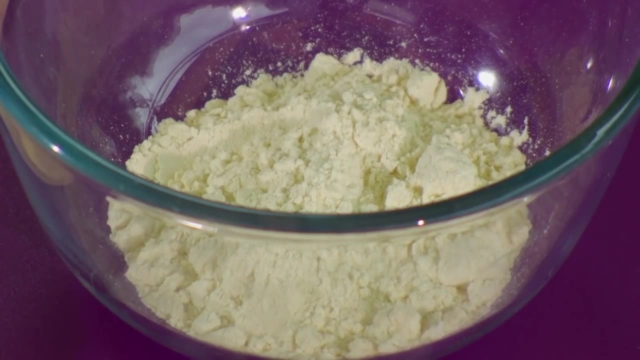 it again. Yeah, Let's do a really big pop at the end this time, And don't forget to join in with us: Pop Brilliant. Now, to this self raising flour, we're going to add some lovely caster sugar, And caster sugar is a little bit different to the kind of sugar that you might be used. 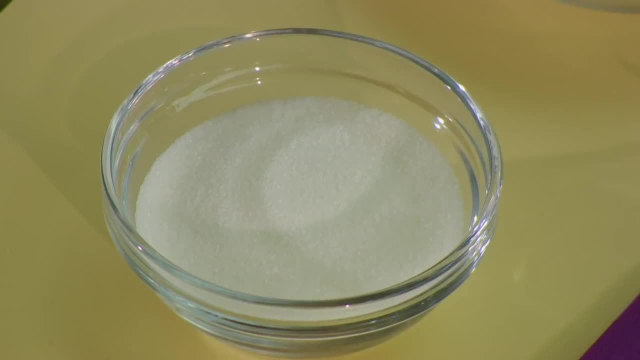 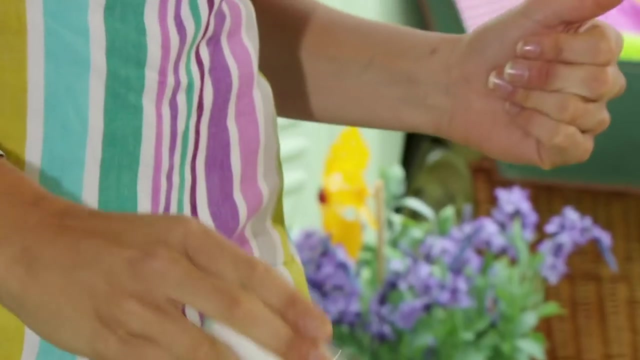 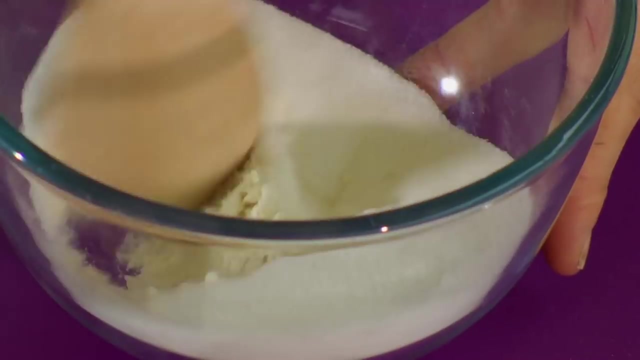 to using when you're at home, And that's because the pieces are a lot smaller. So let's pour that lovely sugar in with a big whoosh, Ready Whoosh, And then we're going to give everything a quick mix with our wooden spoon- Ready Whoop. 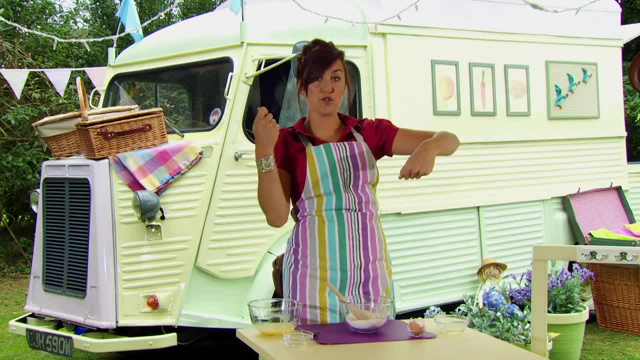 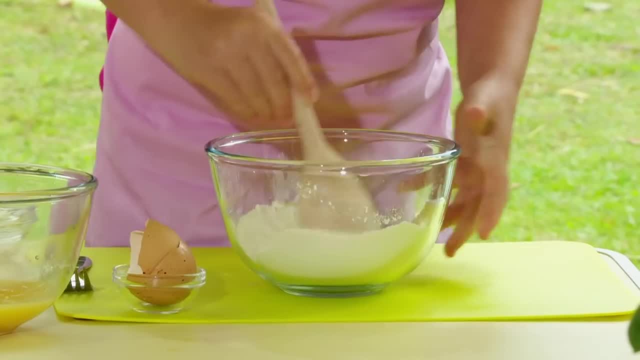 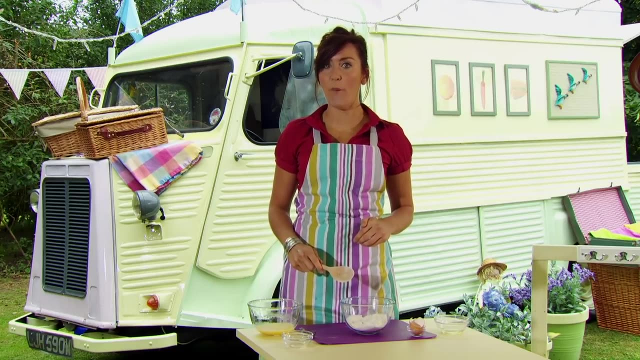 And don't forget to mix with us. Get your bowl and your wooden spoon and mix it up. Sit up, Brilliant. Now. what ingredient do you think we're going to need next for our sunny carrot cake? What's next? Let us see if you can guess what it could be. 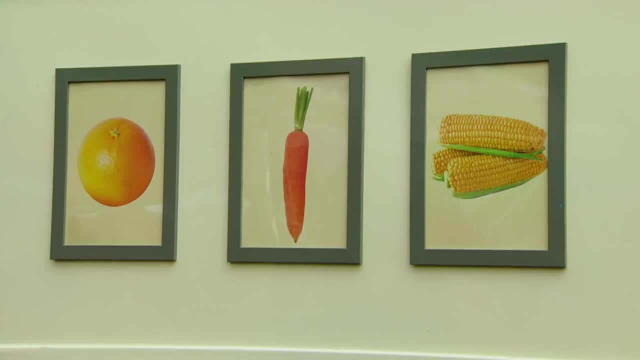 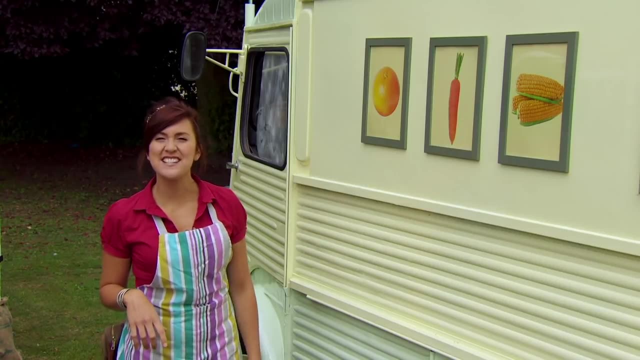 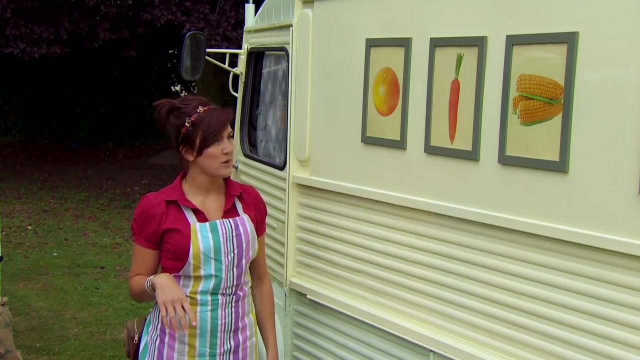 We've got an orange, a carrot and some sweetcorn. What would you choose for our sunny carrot cake? I know I'll give you some clues. There's special ingredients in the carrot cake that we're going to need. The special ingredient is orange. Well, sweetcorn is yellow, so we 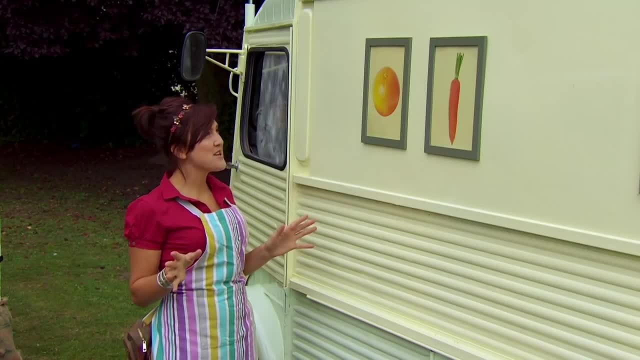 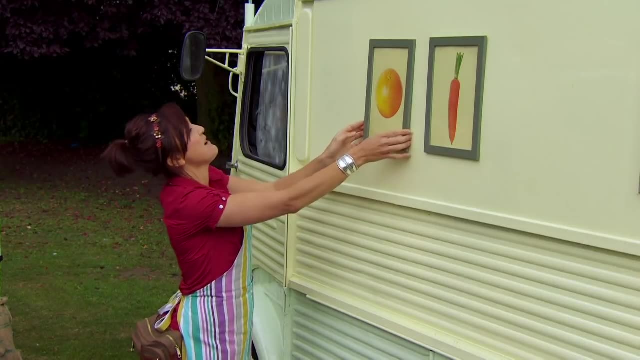 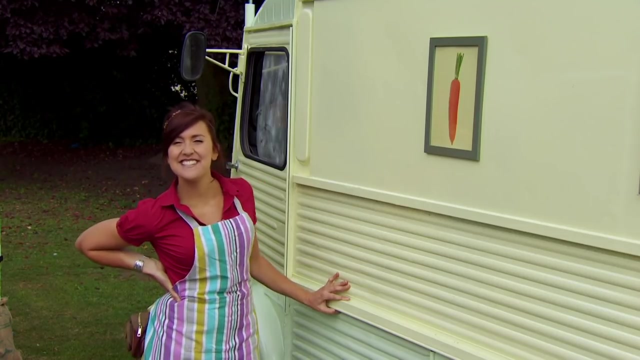 can take that one away. And here's another clue: The special ingredient is a vegetable. Well, oranges are a fruit, aren't they? So we can take that one away too, Which leaves us with a carrot. We're going to need carrots in our sunny carrot cake, And earlier I went. 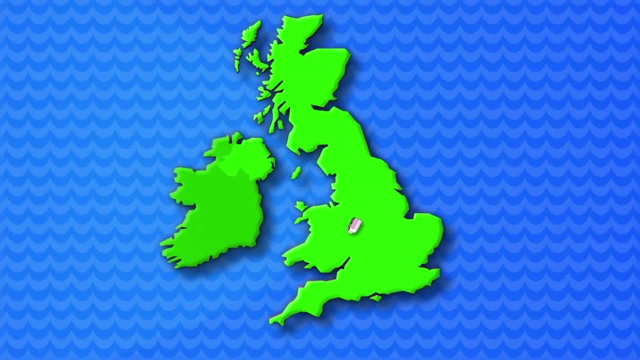 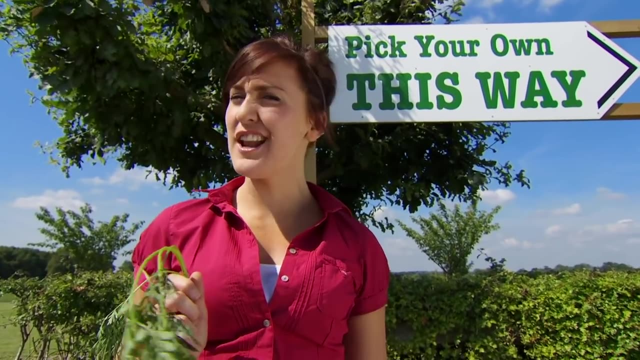 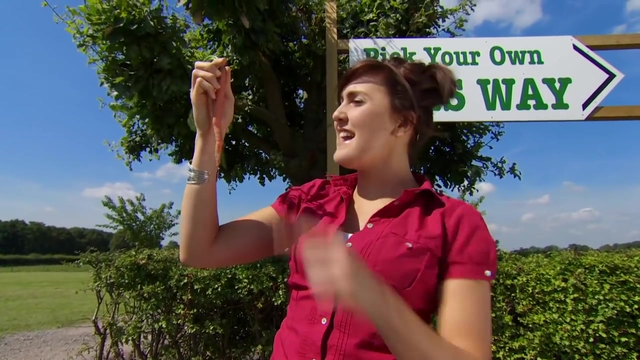 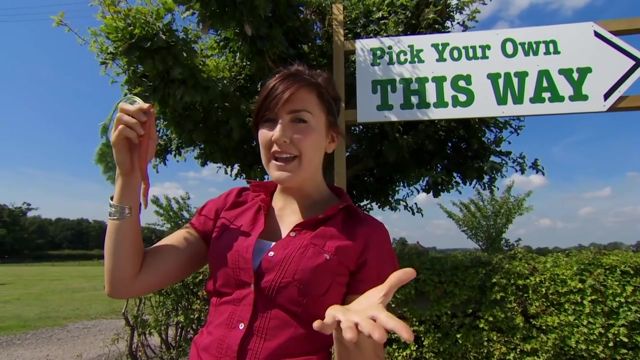 to find some. I've come to Esher in Surrey to look for some carrots, and I've come to a farm where you can pick your own. This is what we're looking for Now. this part of the carrot, which is the part that we eat, actually grows underneath the ground because it's the root, So we need. 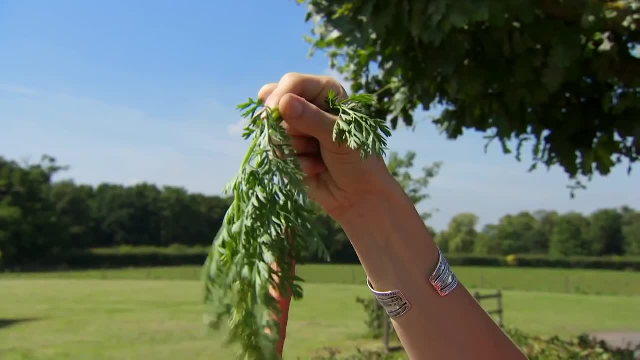 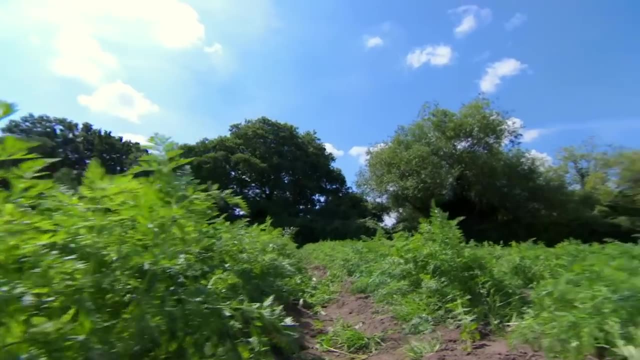 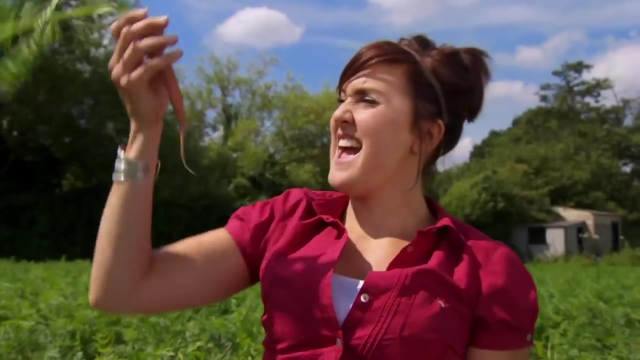 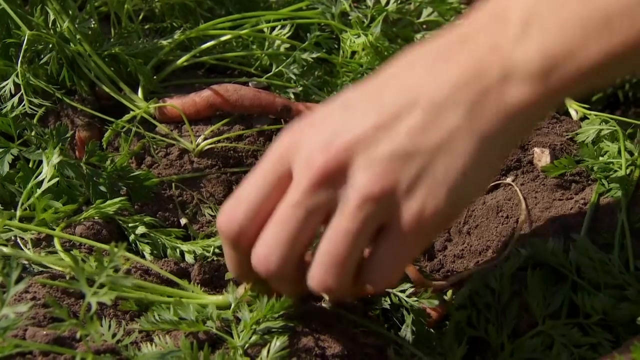 to look for the bushy green leaves which grow above the ground. So come on, let's go. Look at all these carrots I've found. There's hundreds of them. I've found a big carrot and I've found a teeny, weeny carrot. I've also found a curly, whirly carrot. Look at. 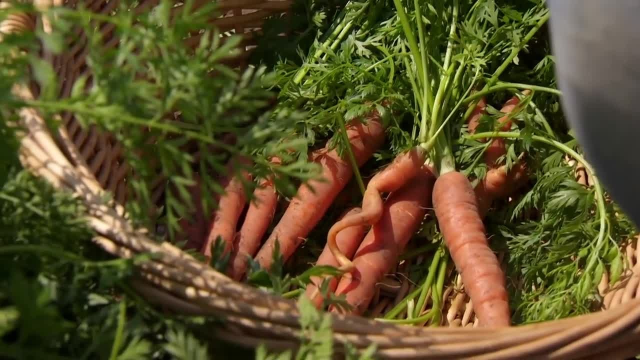 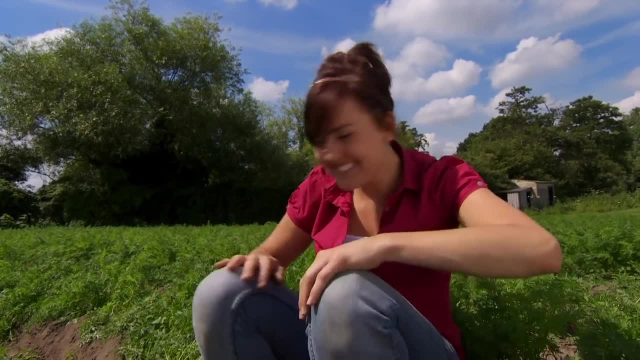 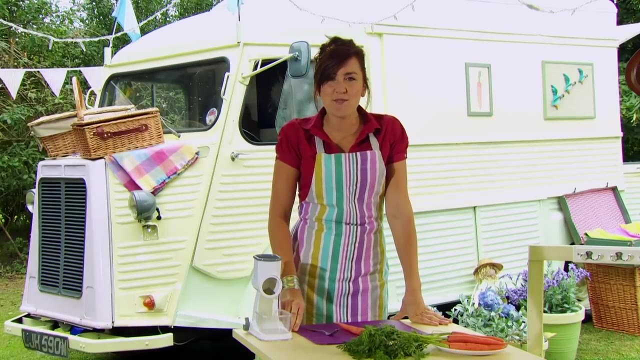 that It's brilliant. I'll definitely keep that one. Now, once I've given these a wash and taken the leaves off, they're going to be perfect for our sunny carrot cake. That was so much fun getting all those carrots out of the ground And you've got your carrot. 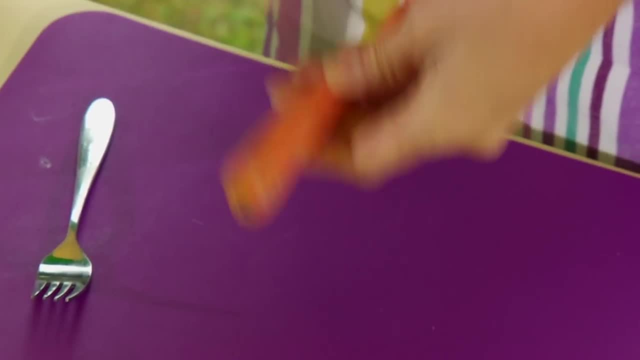 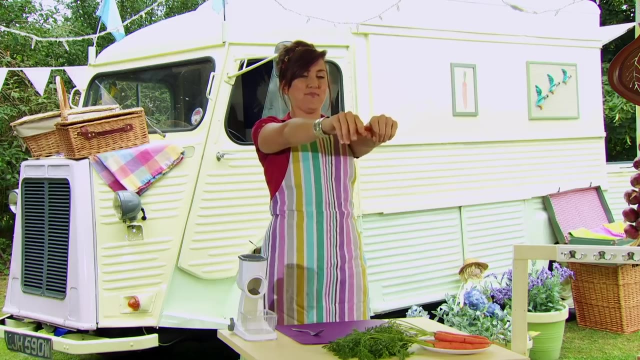 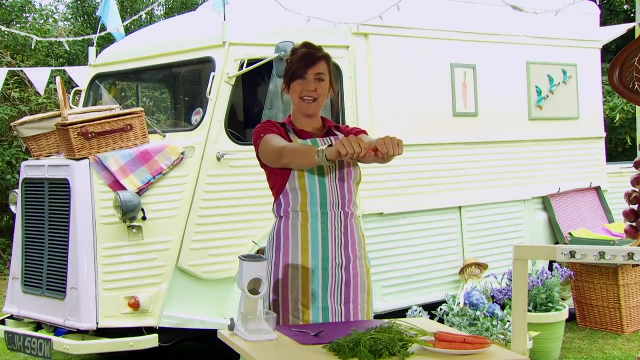 down here and he's had a hair cut already And we need to snap this carrot in two And to do that, we're going to hold it like a pair of bicycle handlebars like this And go for a quick ride Meow. So after three we're all going to snap our carrots, Ready One. 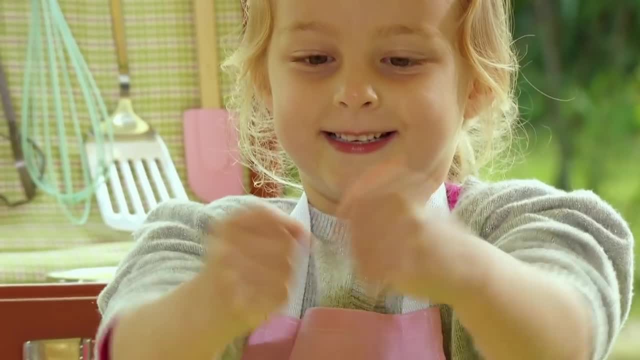 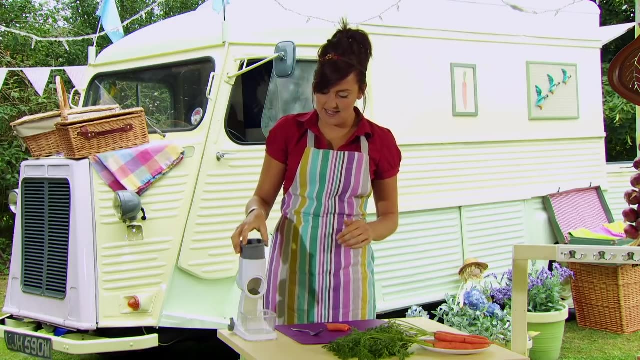 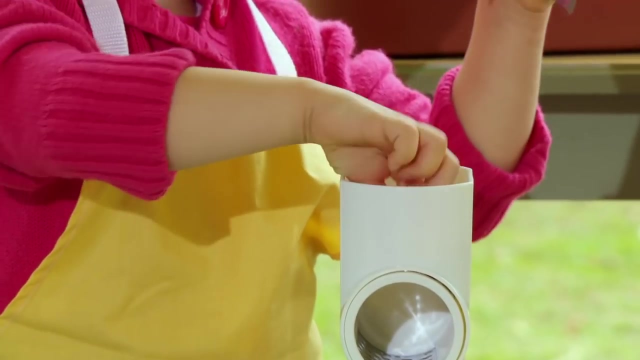 two, three, Snap. There we go. So we should have two pieces. And next we're going to grate our carrot, So we need to take the lid off our grater and one person puts their pieces of carrot into the top of the grater. Put the lid on top. You're going to hold the top down. 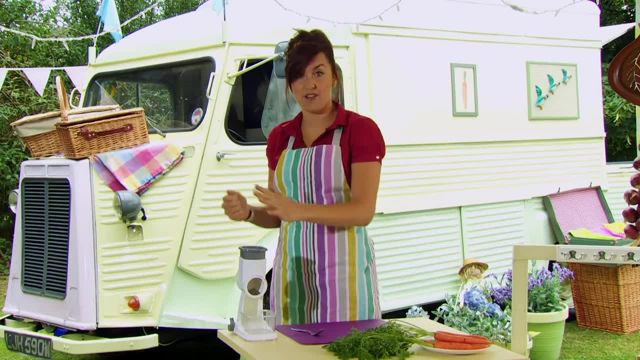 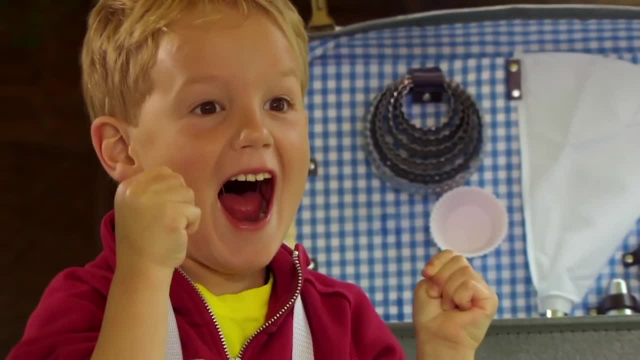 and then you're also going to turn the handle to grate it. But to do that you need to be very, very, very strong. Now, how strong are you, William, Very. And how about you, Caitlin, So strong? Can you show me your muscles too? 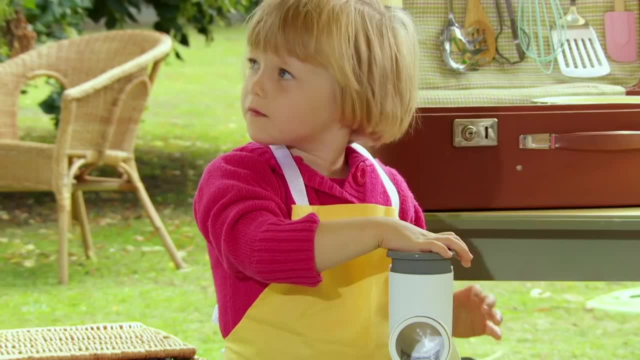 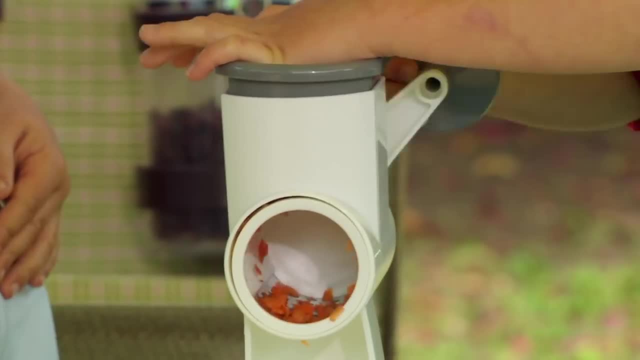 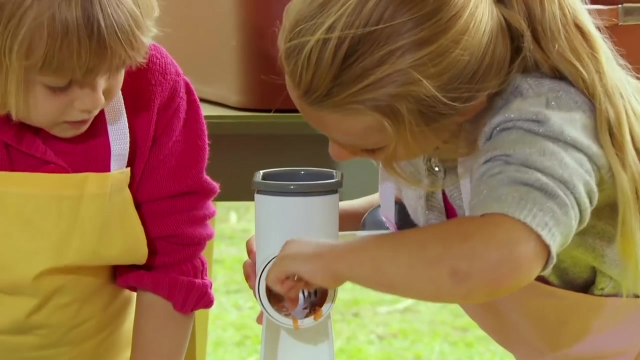 Grrrr, Oh gosh, you're very strong, So let's get grating. The round bit of the grater is quite sharp inside, so you need to use a fork to get the rest of the carrot out. Push really hard on the top, William. 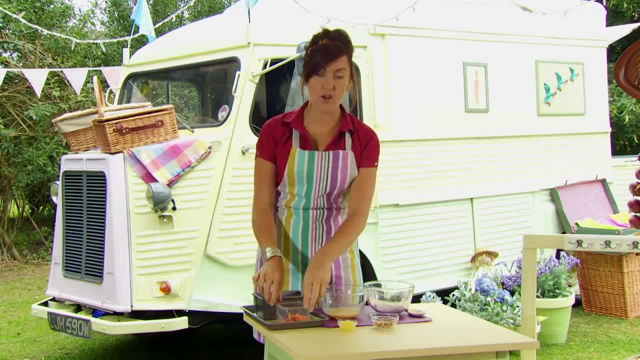 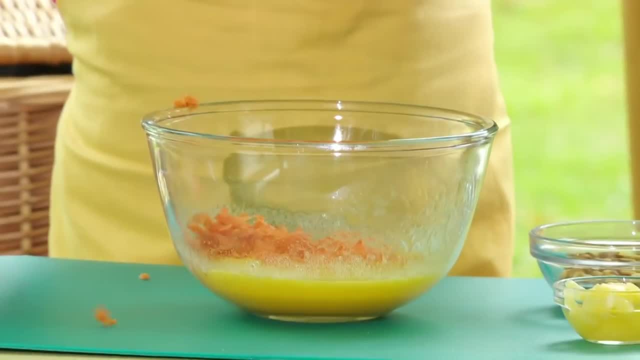 Grrrr, Grrrr, Grrrr. Let's add our grated carrot to our eggy mixture. There we go, Just pour it in Whoop. Next we're going to use some of these. Now, William, do you know what these are? 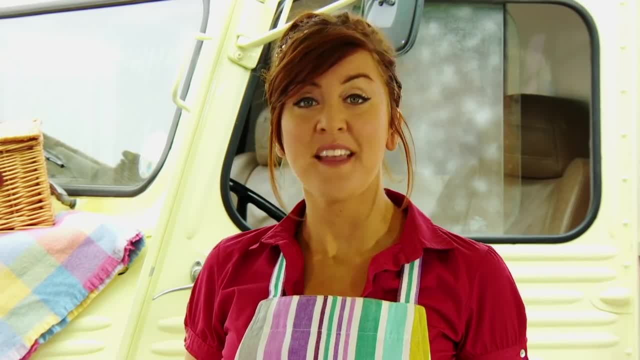 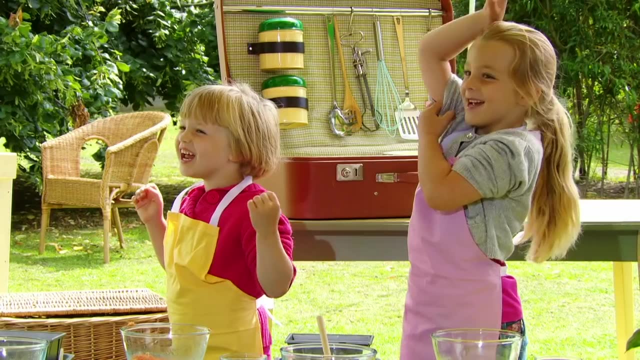 Nuts? That's right, They're walnuts, And if you can't eat nuts, you can just leave them out. And who wants to see the walnut face? Yay, I will show you, Betty, Who wants to do the walnut face. 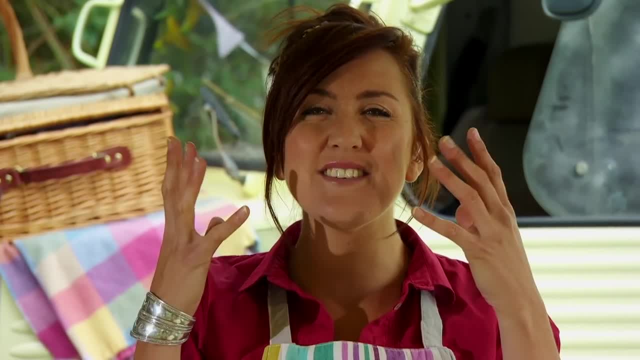 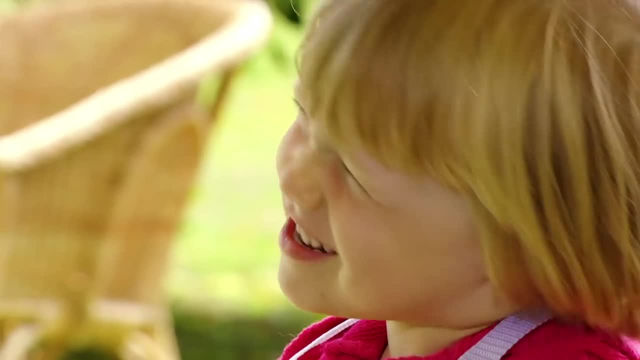 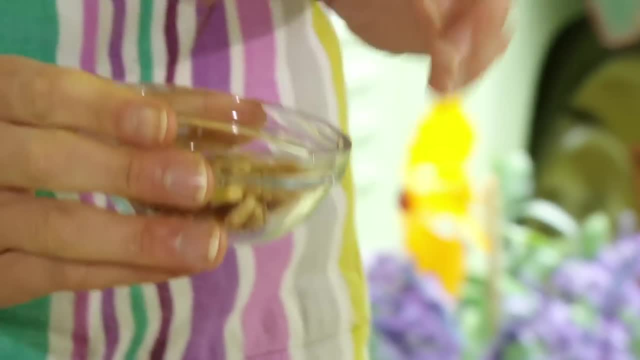 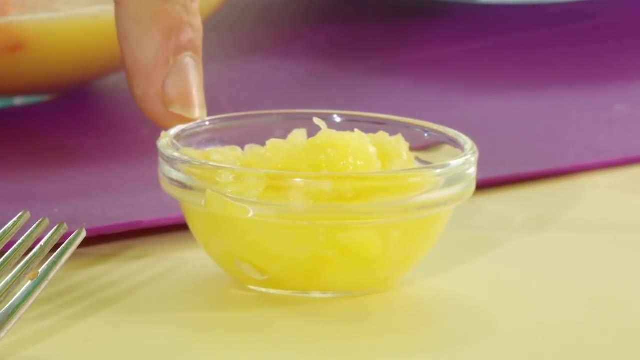 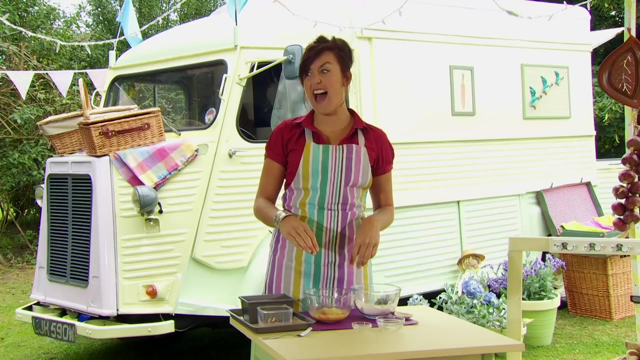 And then we're going to add some of this. Do you know what that is? Pineapple It is, and it's crushed pineapple. Let's pour that in. There we go. So let's press the fast button on our hand. Beep, beep, beep. 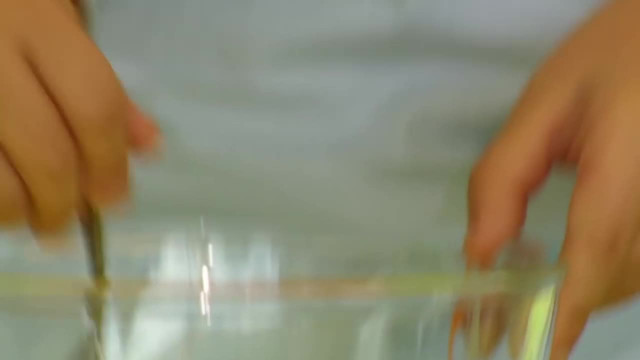 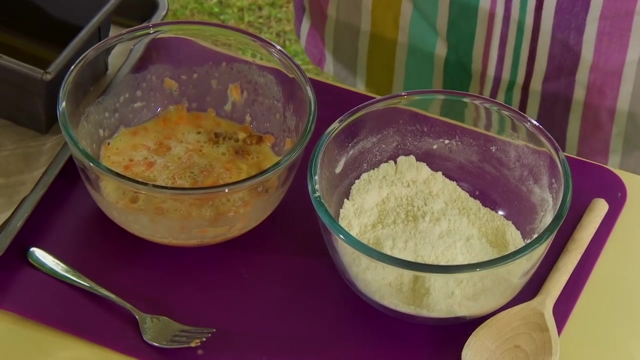 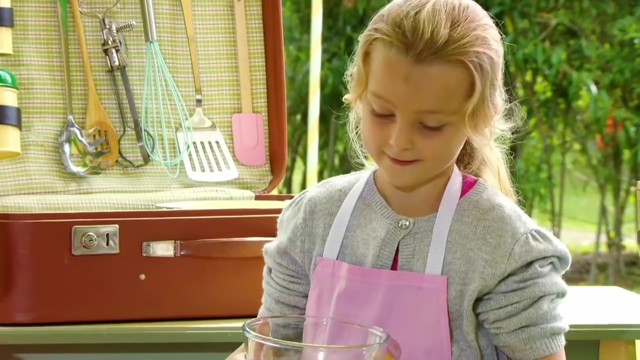 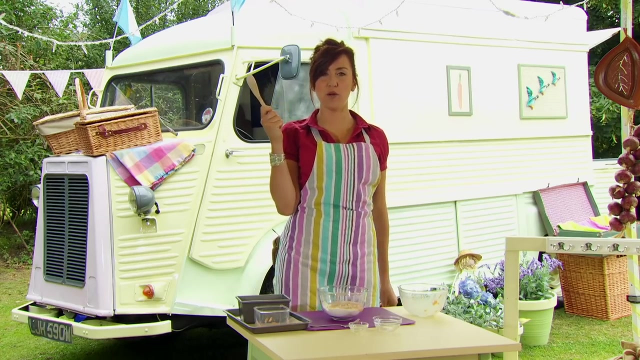 Let's go, Meow, Brilliant. Next, we're going to pour the wet bowl into the dry bowl And this is going to make a really big splash- One, two, three Splosh- And the next thing we need to do is take our wooden spoon and really give everything a. 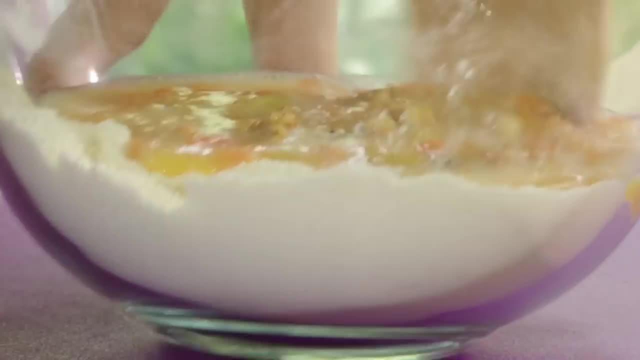 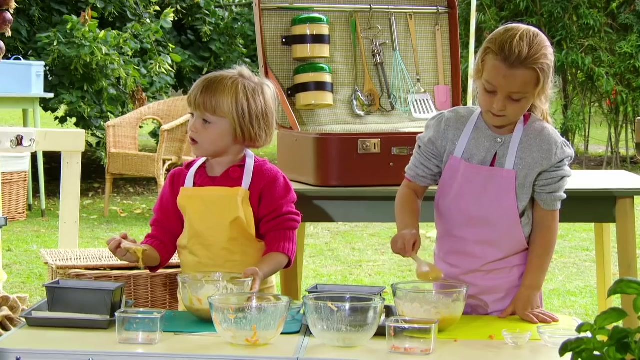 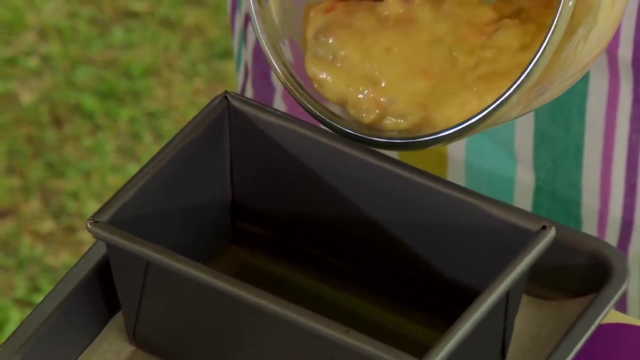 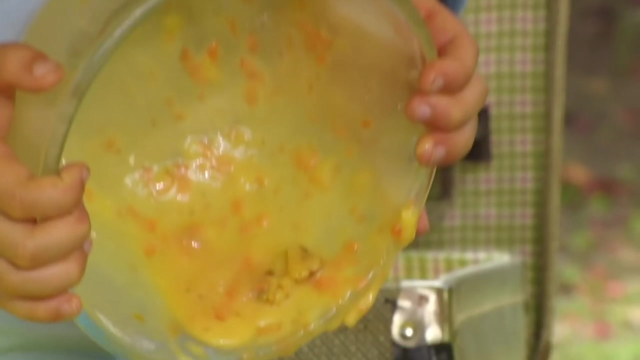 good, fast mix, And we need to keep mixing until all that flour magically disappears. Finally, we're going to pour our mixture into our loaf tin that I've already oiled for you using our wooden spoon. Okay, Splodge, splodge, splodge. Last little bit And that is it. 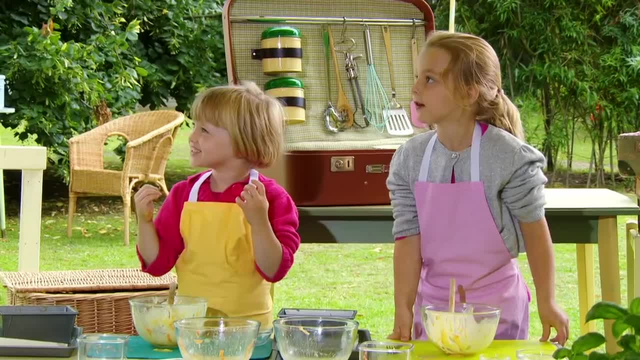 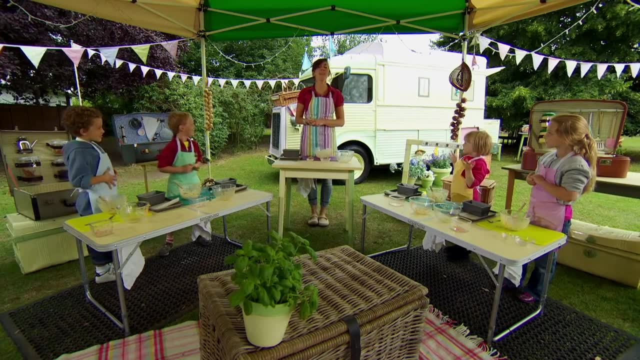 You've done it. You've done it: You've put all the ingredients together for your sunny carrot cake and you did it all by yourself, Brilliant. And now I'm going to put them all in the oven for you. Remember, ovens are hot. 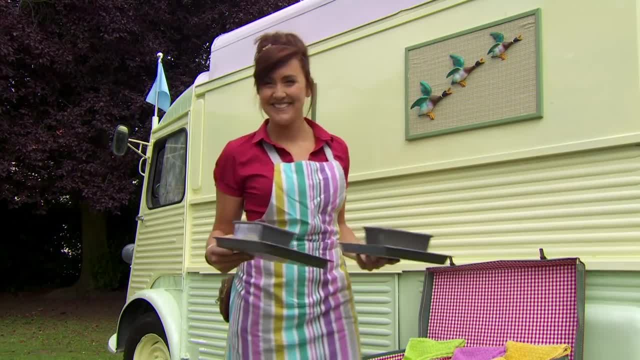 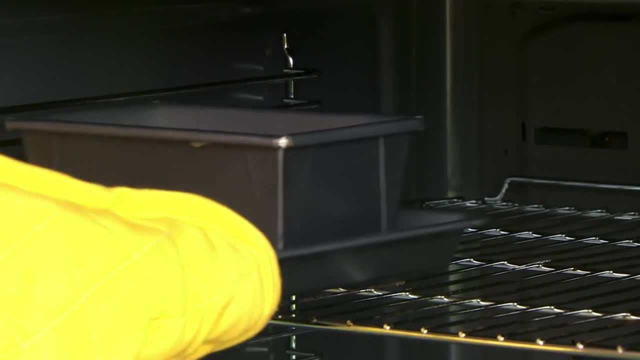 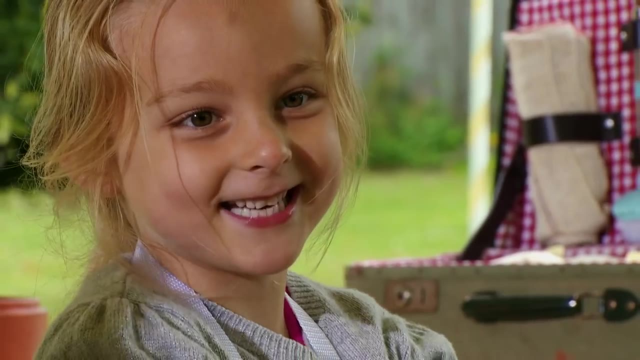 so don't go near Ask a grown up to help you here. Now. we've cooked with you and had lots of fun. Let's tidy up and think of all the things that we have done. There was cracking, whisking, mixing, grating. 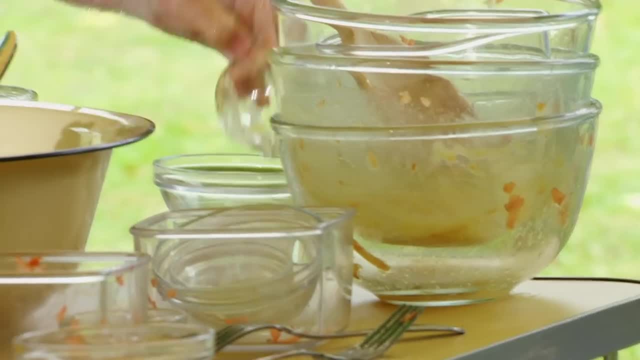 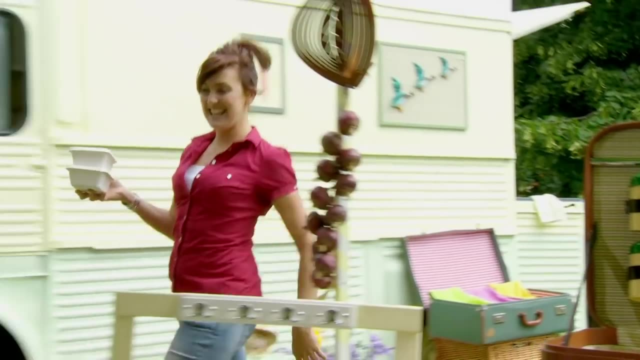 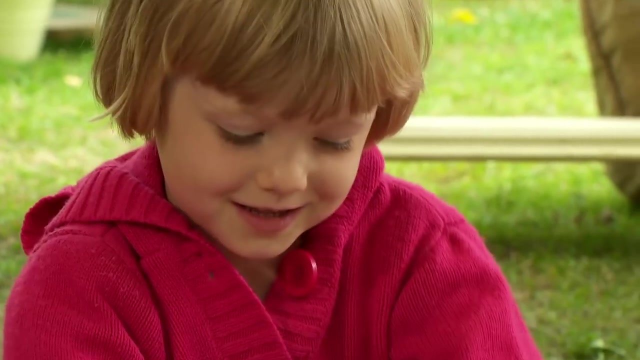 Now, clearing any mess and putting things away is always fun to do at the end of the day. And here they are, All cooked and now ready to eat. Okay, let's have a look at yours, Caitlin. Yummy, Ooh. What does it smell like? 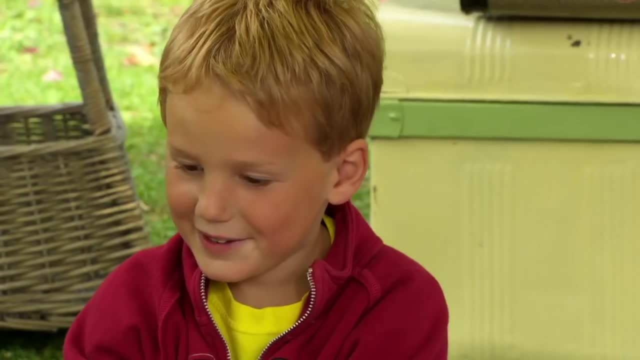 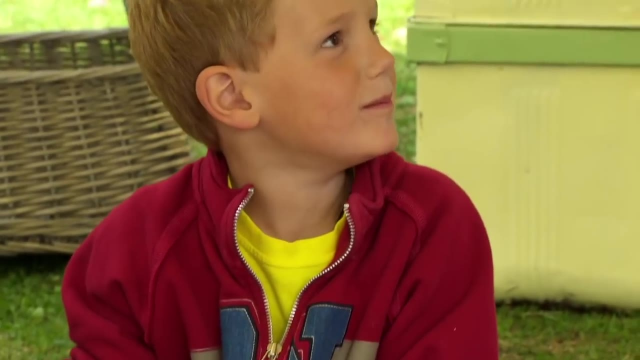 Yummy. Okay, William, let's have a look at yours. Ready, Open? Ooh, Wow, that looks fantastic. What does it smell? like? Um pineapple? Oh, can I have a smell? Oh yeah, I can really smell the pineapple in yours. Let's put the. 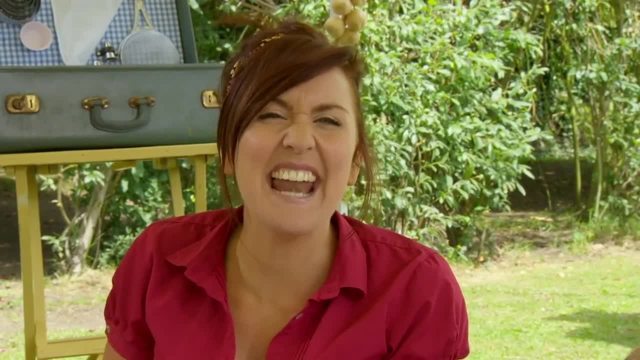 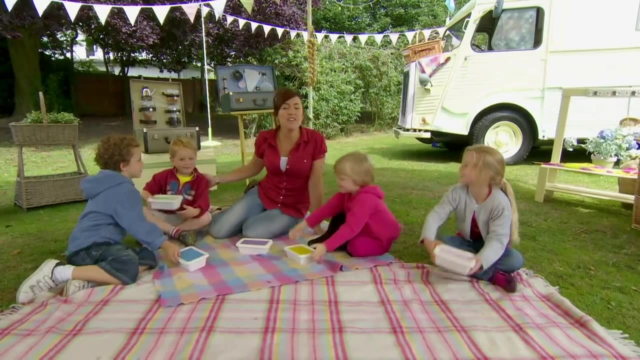 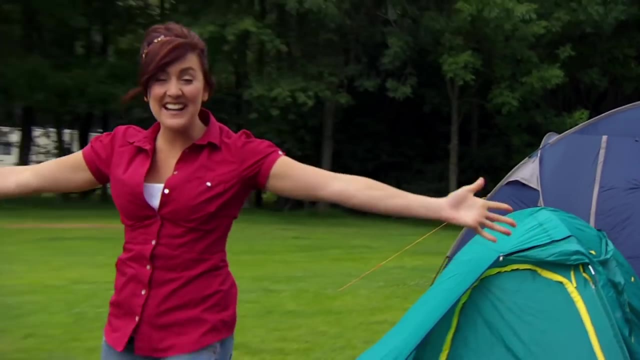 lids on top. We've travelled to you, we've cooked and had fun. Now let's have a party with everyone. Yay, Come on, you can come with us, Follow me. Well, here we are at the campsite and we are all ready for a delicious picnic, aren't? 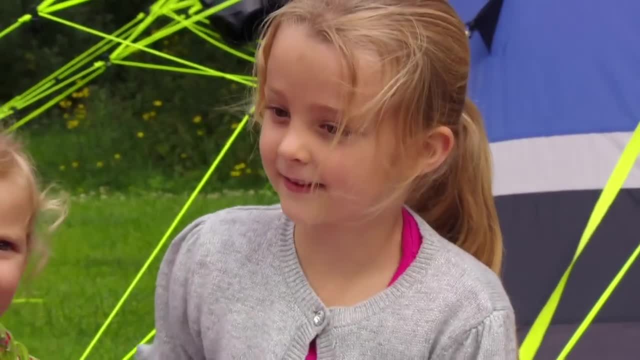 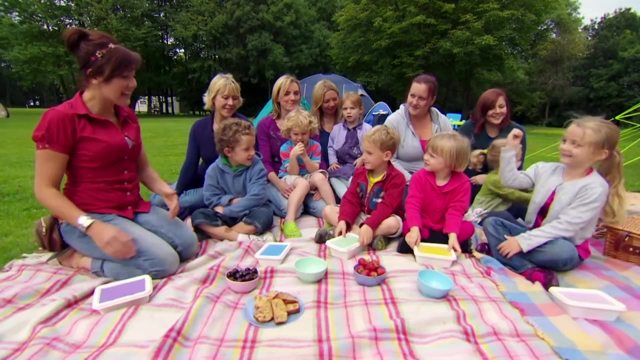 we everyone. Yes, Oh, I am so hungry for some sunny carrot cake. Mums and brothers and sisters, would you like some too? Yes, Brilliant, Okay, everyone, let's tuck in. We've got one slice for everybody. 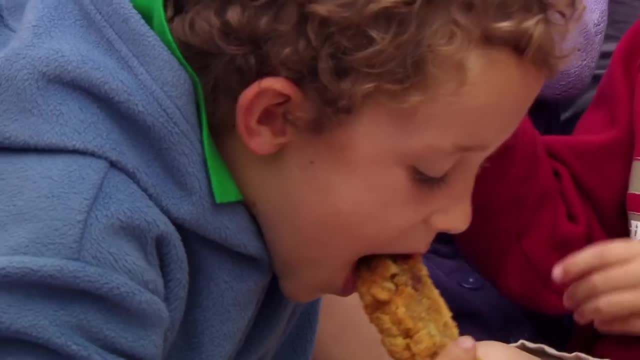 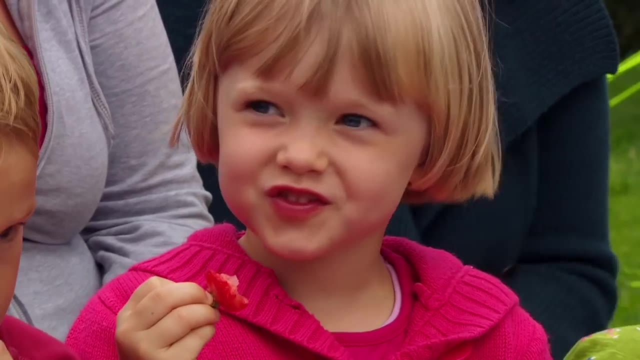 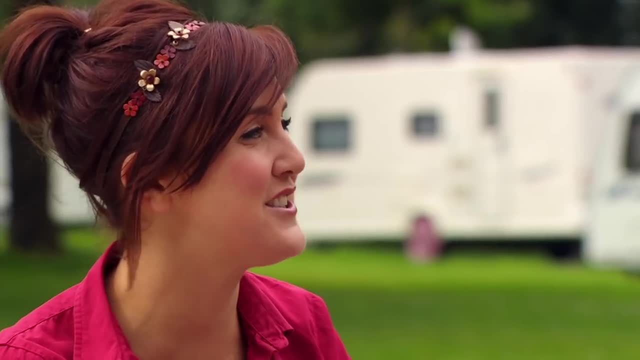 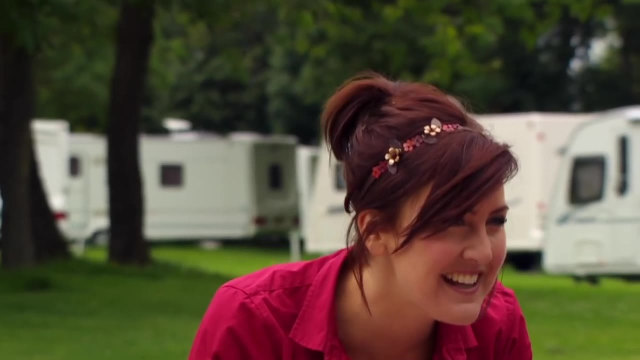 Chocolate cake as well. Yeah, What would you like Olivia to cook for you? Definitely more carrot cake, More carrot cake. We've got to make more carrot cake, Yeah. So what can you do? everybody, I can cook, I can cook. 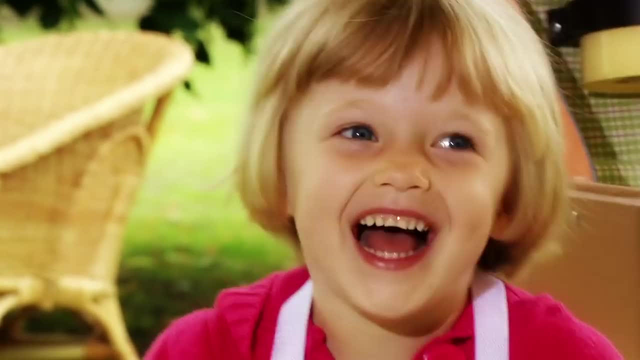 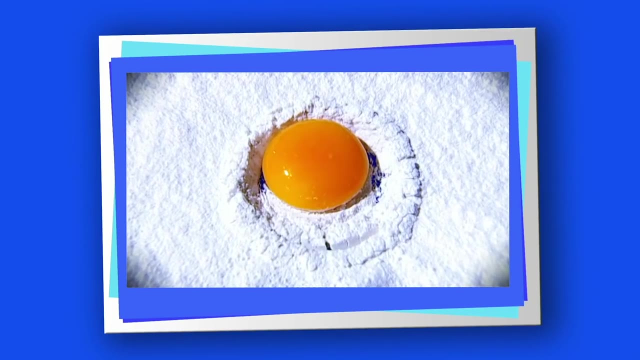 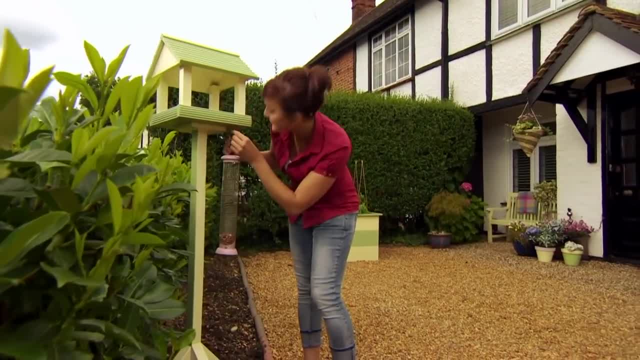 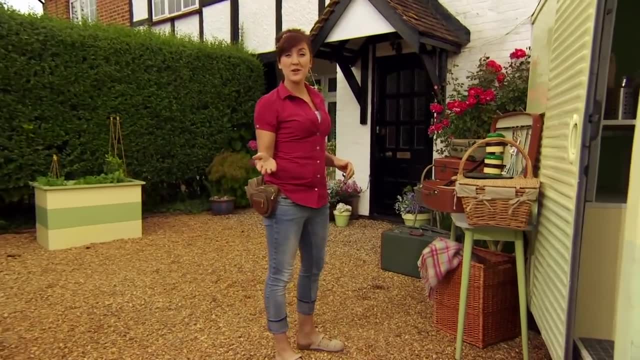 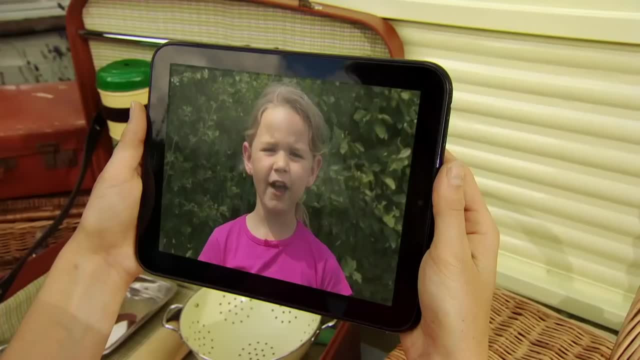 I can cook With you. Oh great, I'm so glad you came. I've been getting everything ready to go on an outing and I hope that you'll come too and meet some new friends. Ah, Here we are. Hello, Kati. 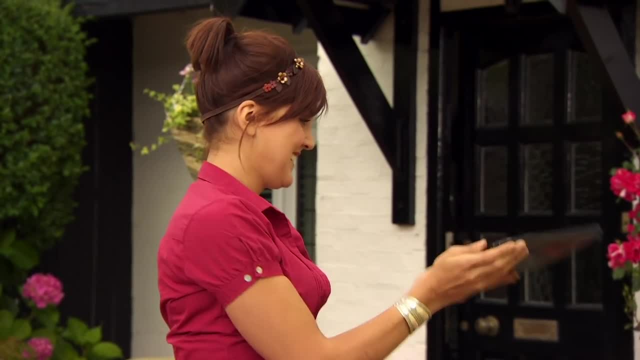 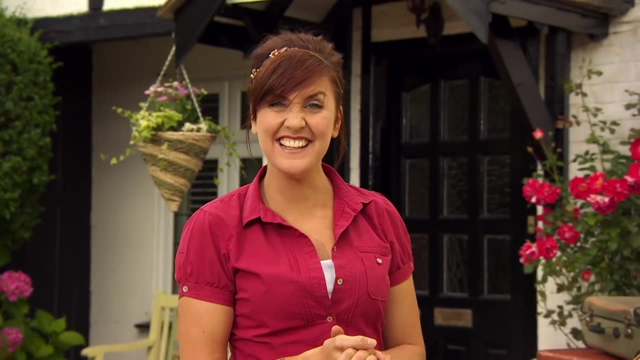 My family love going on boat trips and I like fish. Definitely can Amber, Brilliant, And you can cook with me too. Oh, I wonder if I'll get to go out on the boat. That's exciting, Right, let's get everything packed up and get on our way. 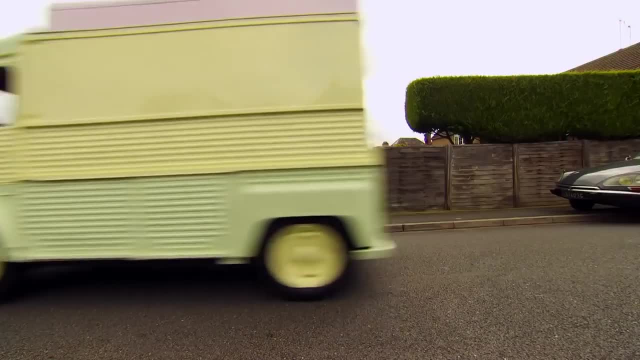 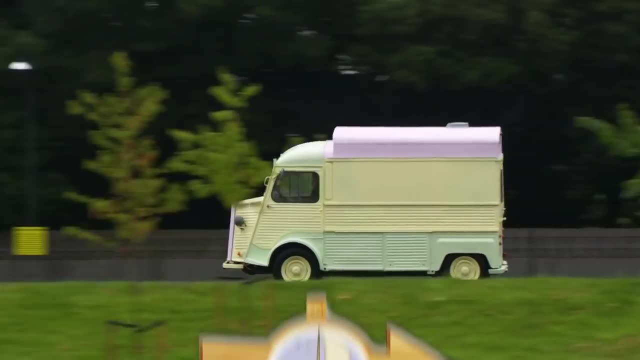 Off on a journey and I'm coming to you. It's going to be busy and there's lots to do. Get ready to help, join in and have fun. Let's cook a feast for everyone. Well, here we are at the harbour where I've been invited by Amber. 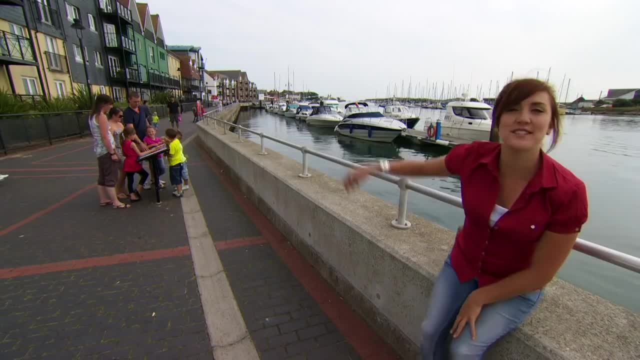 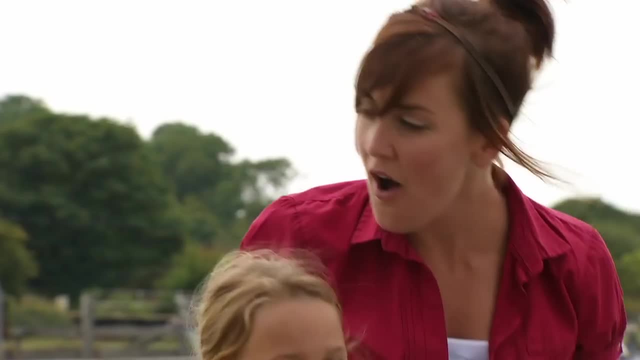 But I don't know where she is. Oh, she's over there with her friends. Hi, Amber, Hi, Katie, Amber, are these all of your friends? Yes, And what's your name? Ryan, Amy? And what's your name, Kyle? 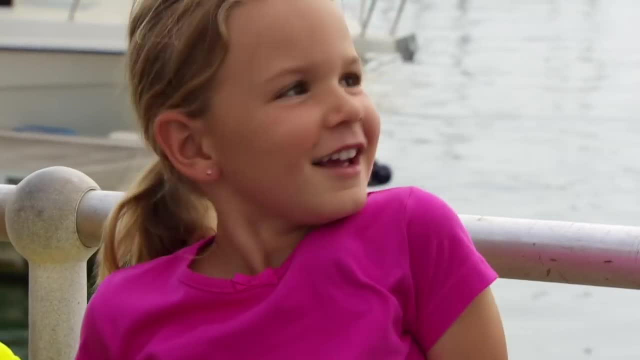 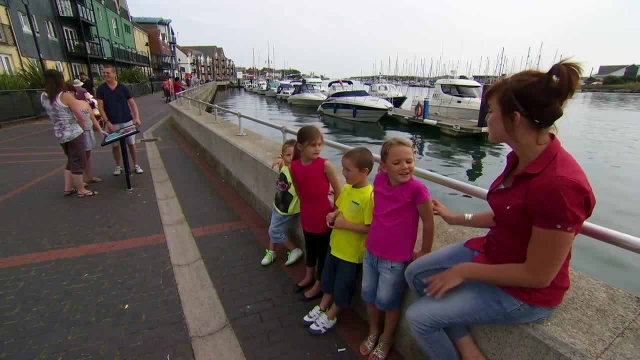 So, Amber, do you want to go for a picnic? Yes, please, And after that, would you like to go on my dad's boat? I would love to go out on your dad's boat, And I've got a really delicious recipe that we can cook for the picnic. 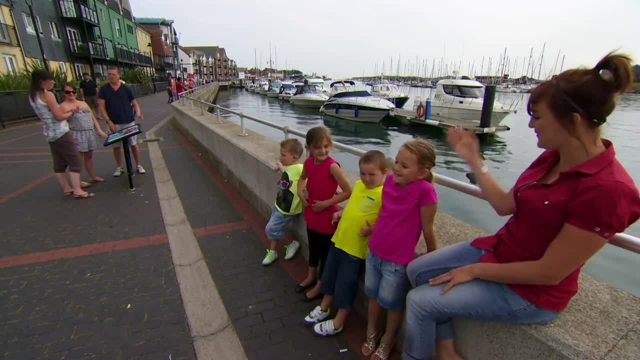 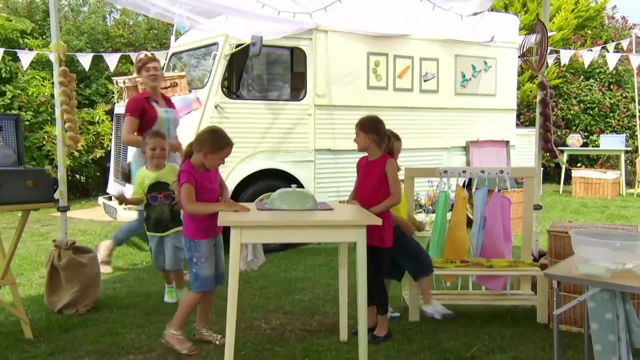 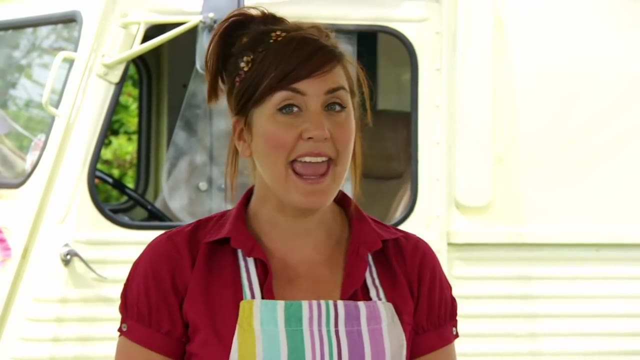 Do you want to cook it everyone? Yes, Fantastic, Follow me. I'll show you Welcome to my outdoor kitchen. Would you like to know what we're going to cook today? Yes, Today's recipe is seaside bites. How tasty do they look. 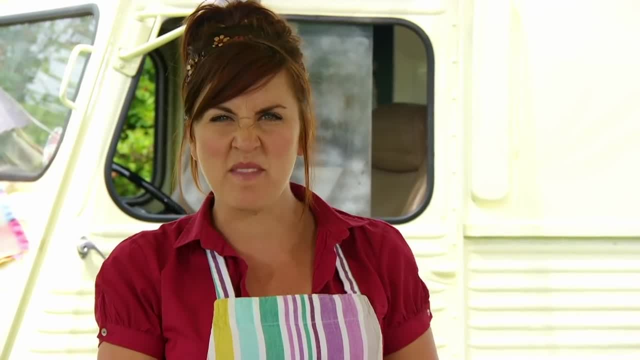 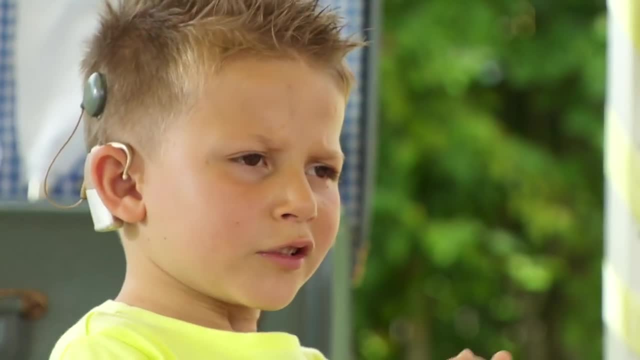 Now, before we get started on the cooking, we've got to do something really, really important. Do you know what it is? Wash our hands. We've got to wash our hands, of course. Come on, everyone, let's get going. 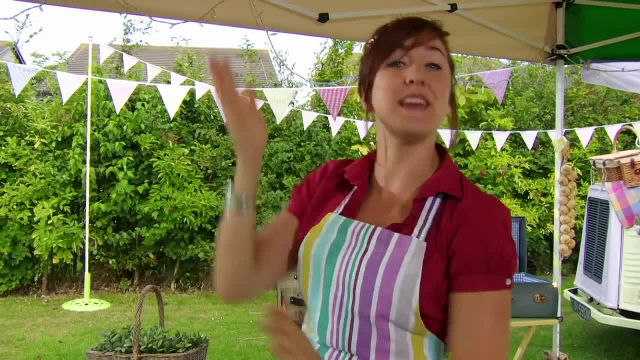 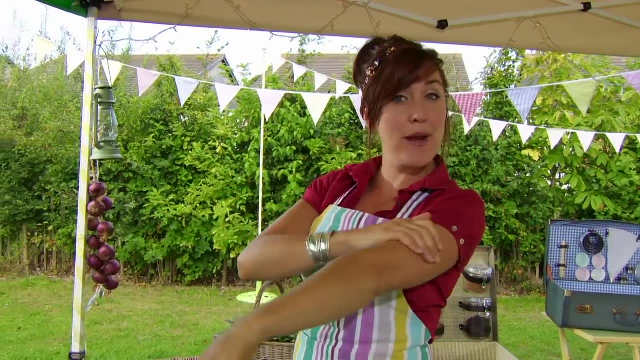 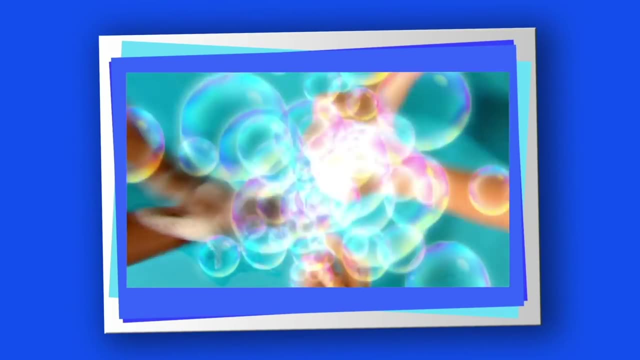 Roll up your sleeves, Give your hands a wash With slippy dippy soap, Splish, splash, splosh. Have you done? your hands Washed and dried? Sleeves rolled up, Apron tied- What can you do? I can cook, Right. well, let's get started on our seaside bites. 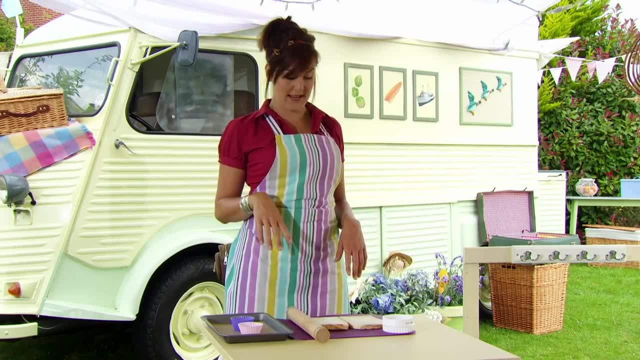 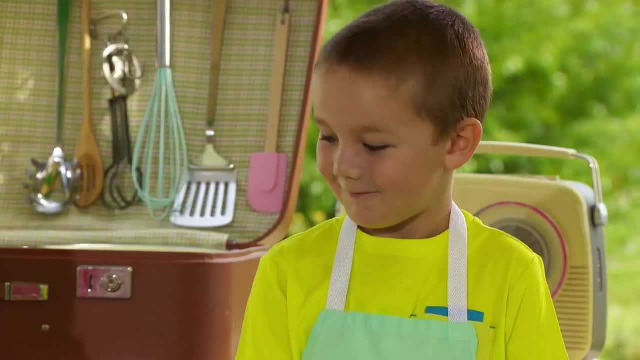 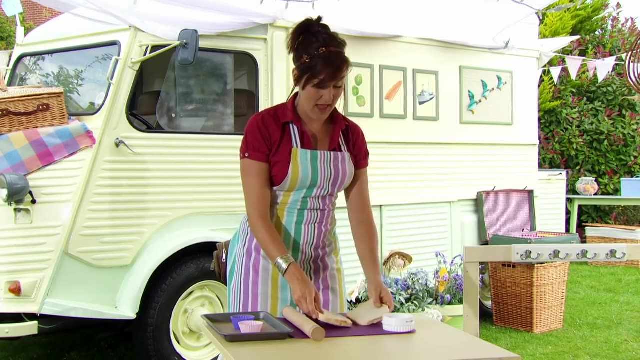 The first thing we need is two slices of bread. Oh, look, watch, If I do this, They look like elephant ears. OK, we're going to use these two slices of bread and we're going to roll them to make them really flat, like this: 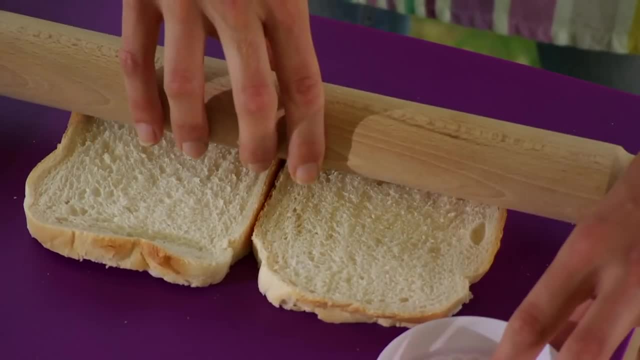 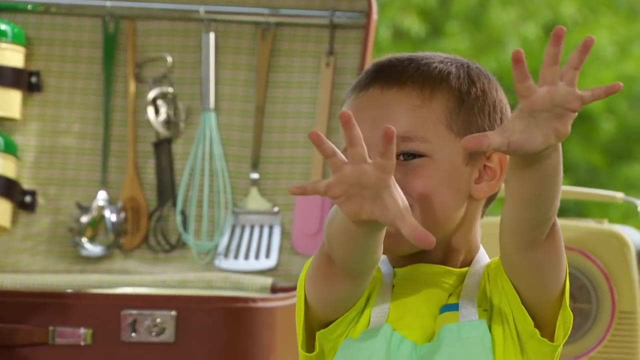 OK, so let's get our rolling pin and put it on top of our bread. Stretch your hands out in front of you like this, and make your fingers really, really wide. And these are your duck feet fingers. Now, keep them really wide. 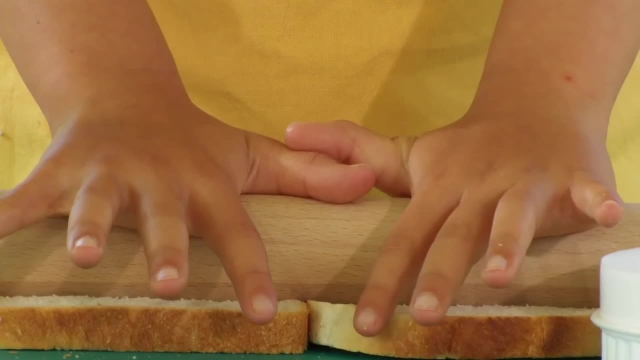 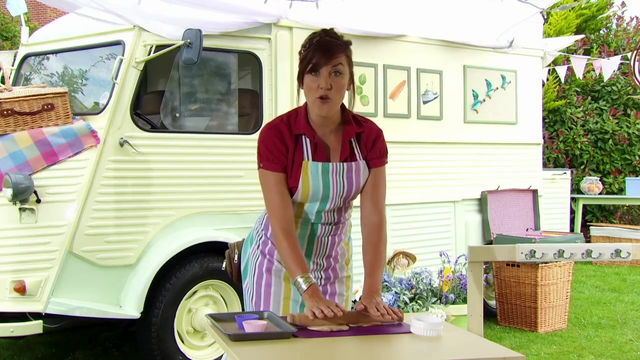 We're going to put them on our rolling pin And then we need to roll the bread to make it really flat. Why don't you do some rolling with us as well at home? You can get your duck feet, fingers and go: Squish squash, squish squash. 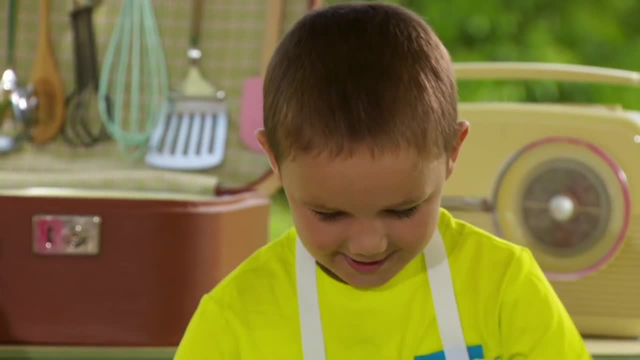 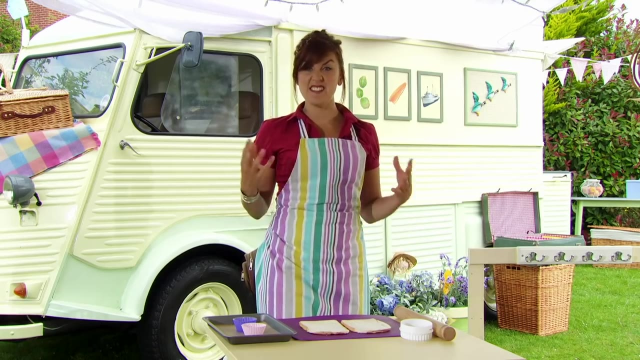 Squish, squish, Squish squash, squish squash. That's good, Ryan, Brilliant. And then we need to make two bread circles, And we're going to do that using a pastry cutter, but we're going to use it to cut the bread. 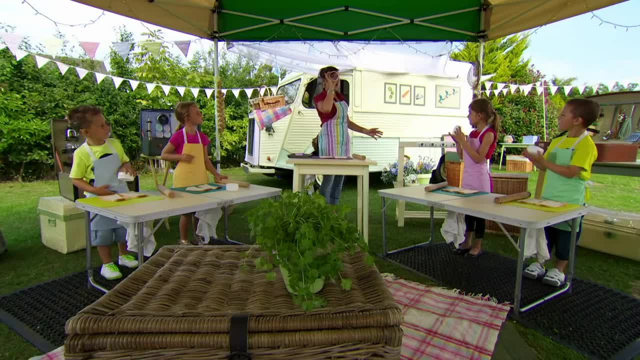 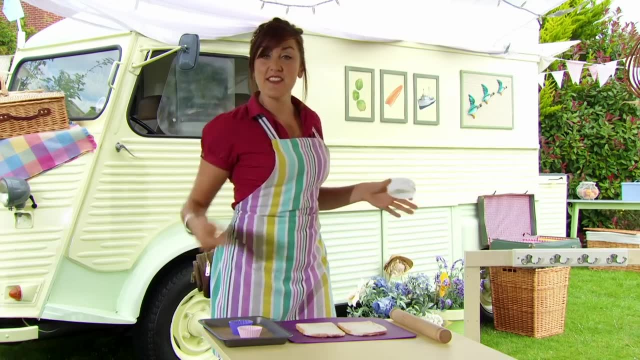 It looks a little bit like a seaside telescope. Ha-ha, What can you see through your telescope, Ryan, Me, Me. Oh, I can see you too. Can you see anything through your seaside telescope? OK, let's use our pastry cutter to make a circle. 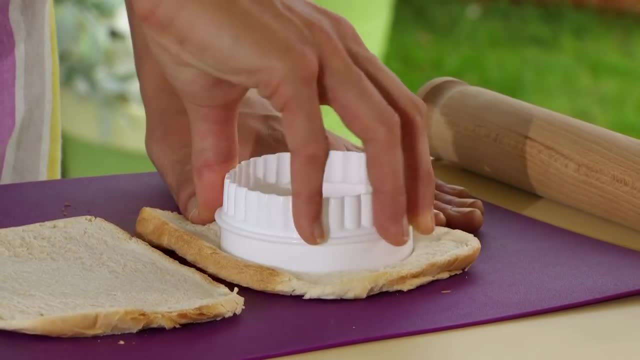 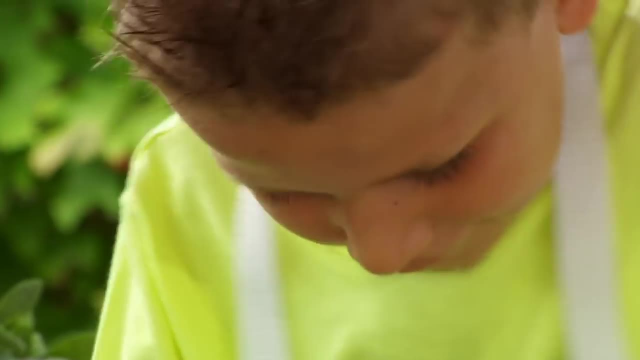 So let's put one here, And we're going to give it a little wiggle and a little twist. Good, wiggling, Wiggle, wiggle, wiggle- Who can wiggle while they do it? And let's do one and the other slice of bread too. 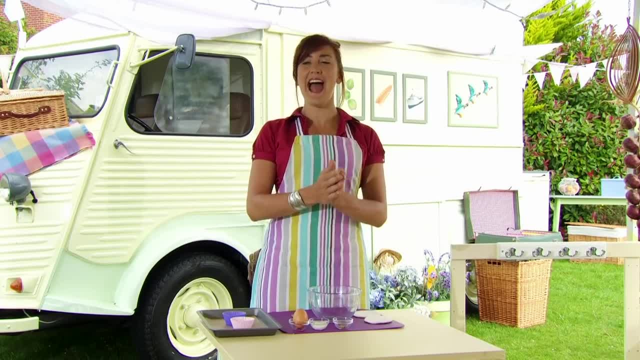 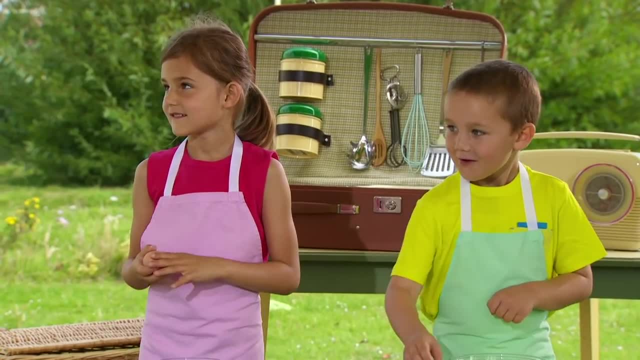 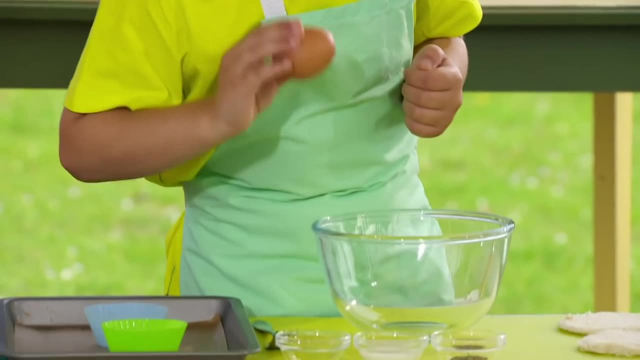 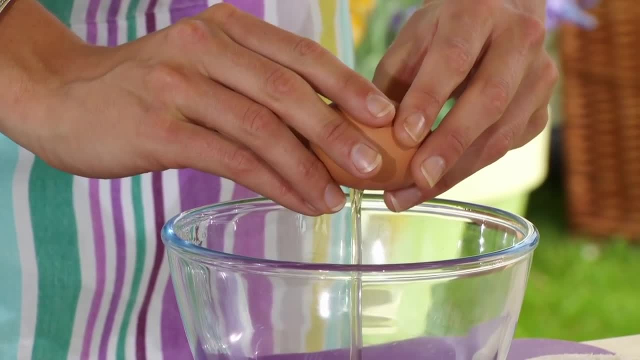 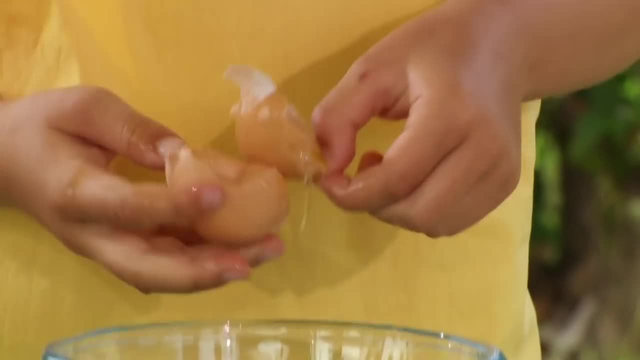 And then we use our thumbs and open it up There. Oh no, That's OK, Just take that bit out. OK, to the egg we're going to add some milk, which is in this little bowl here. Let's splash it in. 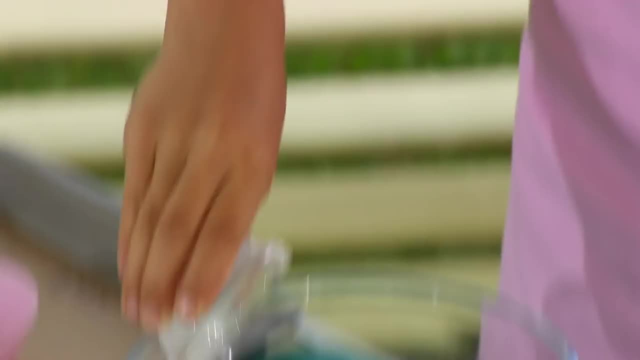 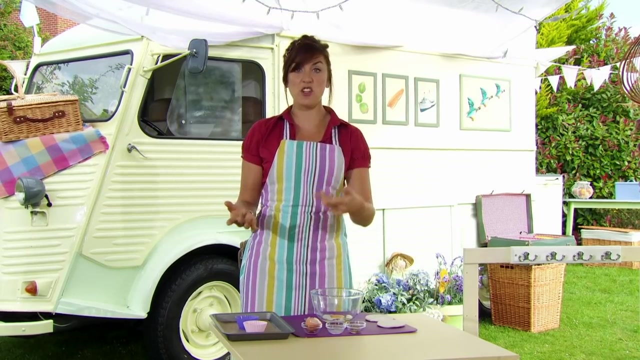 Ready: One, two, three Splash. Now we need to get our pinchy parrot out because we need to take a pinch of black pepper. Now I'll show you how to get your pinchy parrot out. Put your thumb like this: 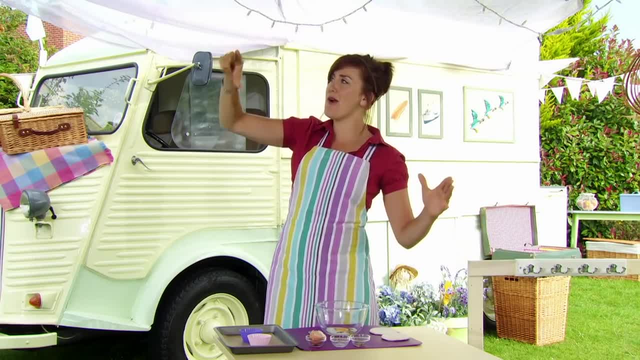 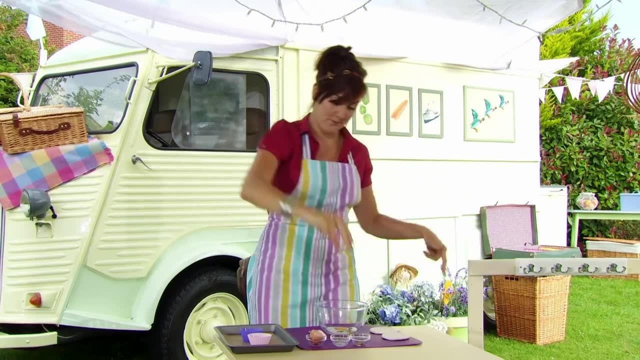 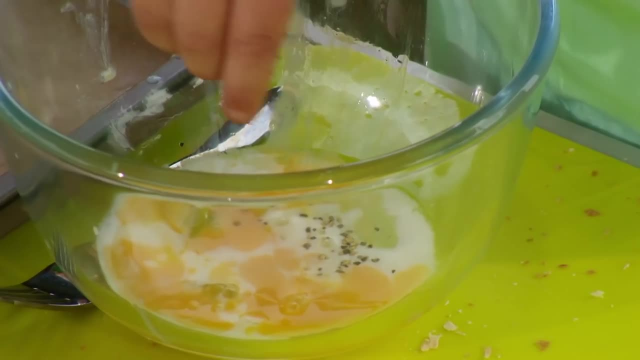 and then you put your fingers like that and you go, And this is your pinchy parrot. He needs to take a pinch of black pepper And sprinkle it into the bowl. OK, now we've added our pepper. we need to mix everything in this bowl. 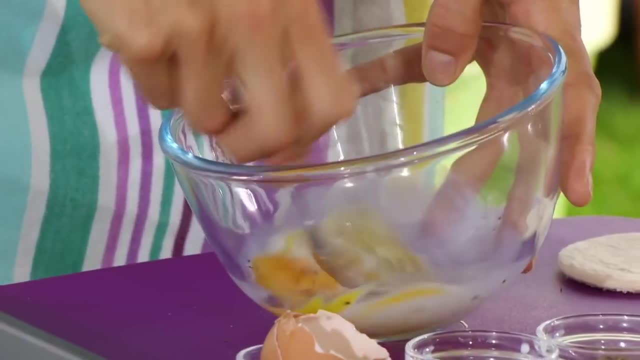 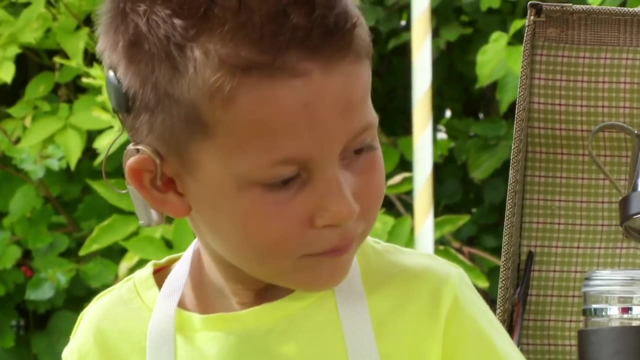 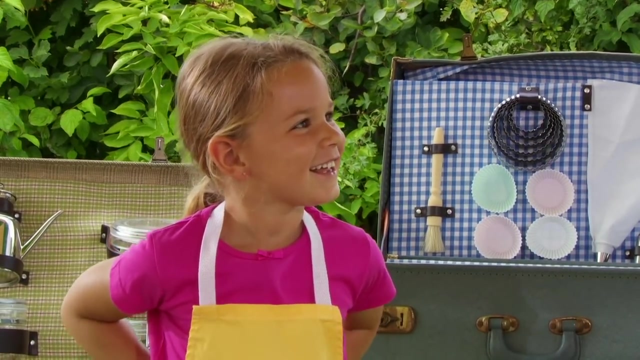 using our thumbs, Using our fork, And stop everyone. Fantastic, You can put your fork down now because it is time To get messy. You've got it. Everyone say: let's get messy. Let's get messy, We're going to take our bready circles. 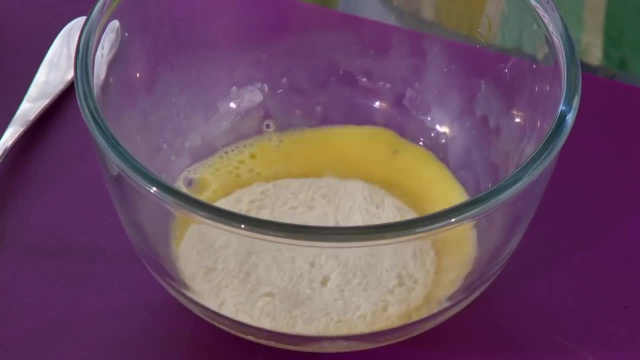 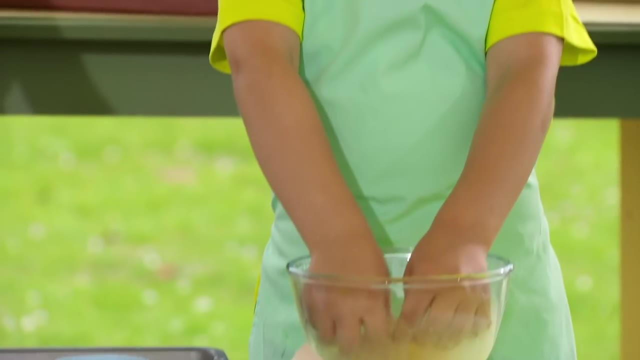 and we're going to soak them in the eggy mixture. Ready, One, two and put your hands in. Ah, look at that. Oh, it feels funny, doesn't it Ryan? Now, once they've soaked up most of the eggy mixture, 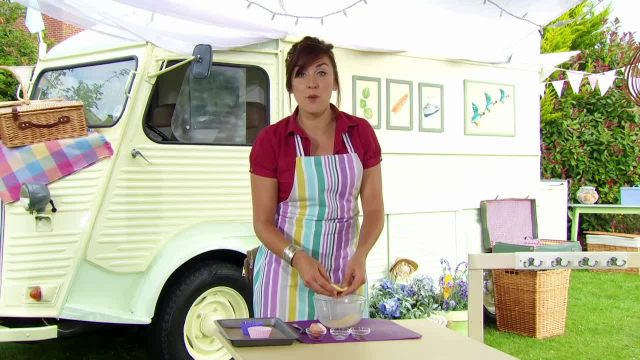 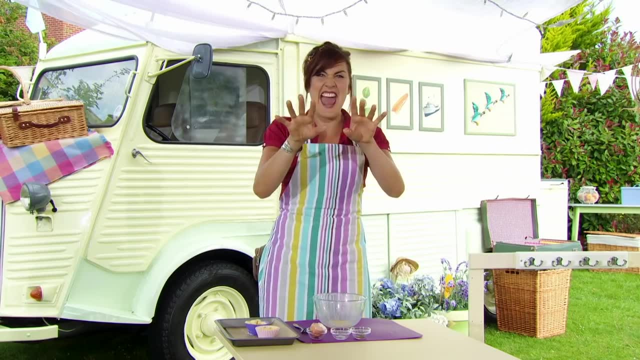 you need to take out your eggy bread circles and put them in your muffin cases over here. It's like a little bed for all the ingredients that we're going to put in later on. Oh, look at these eggy fingers. Shall we give our hands a wipe, everyone. 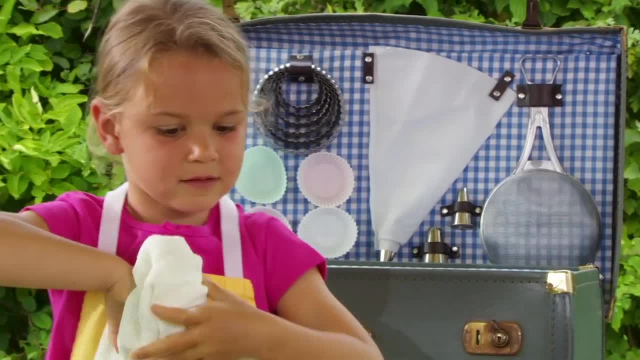 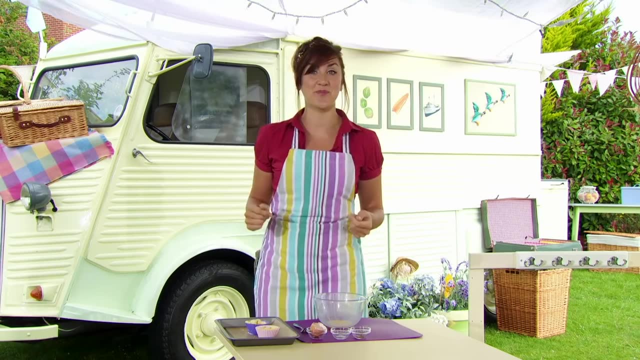 Yeah, I think that's a good idea. Now, what ingredient do you think we're going to need next in our seaside bites? Well, what's next? Let us see if you can guess what it could be. What would you choose for our seaside bites? 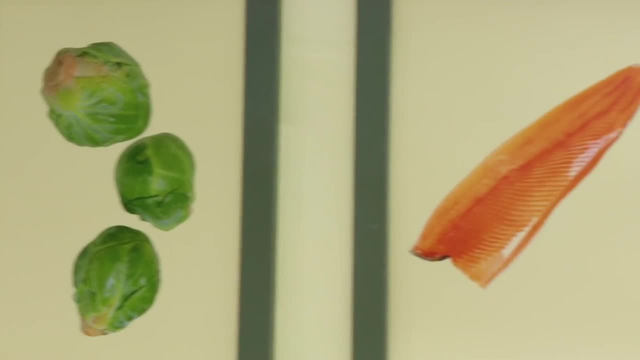 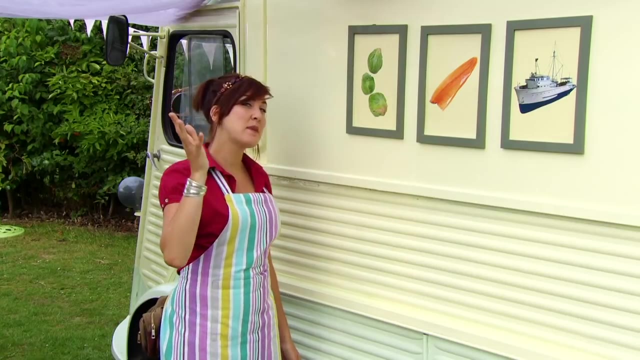 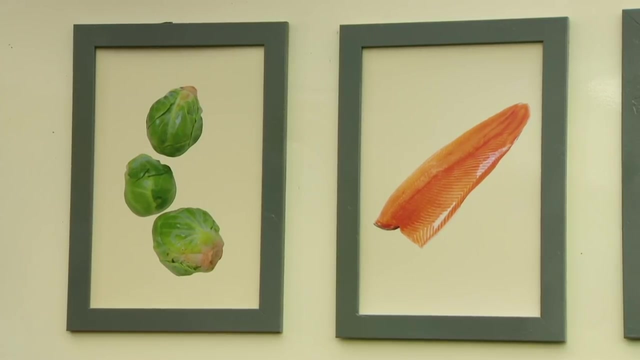 Well, we've got some Brussels sprouts, trout and a boat. Hmm, I know I'll give you some clues and you can guess what it might be. Our special ingredient is found in rivers or the sea. You won't find Brussels sprouts in rivers. 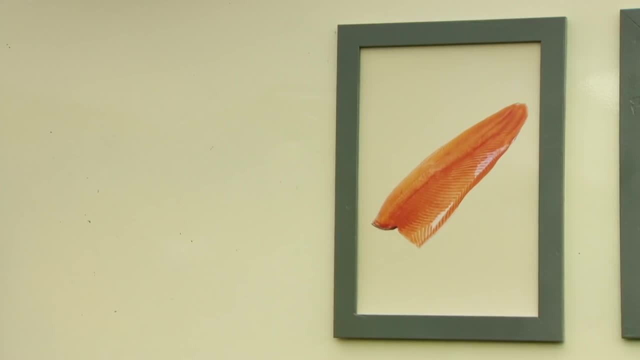 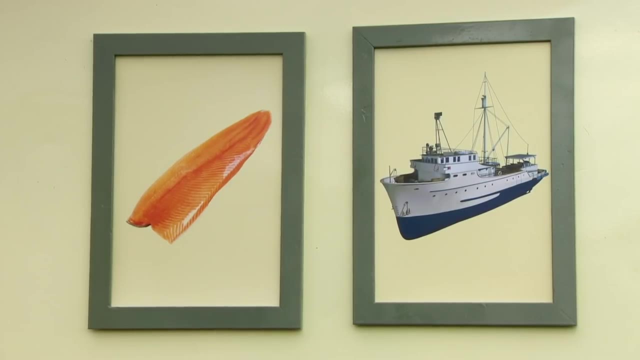 or the sea, will you? So we can take that one away. OK, here's another clue. The special ingredient is found in rivers or the sea, and it's a type of fish. Well, you can find boats in rivers and in the sea. 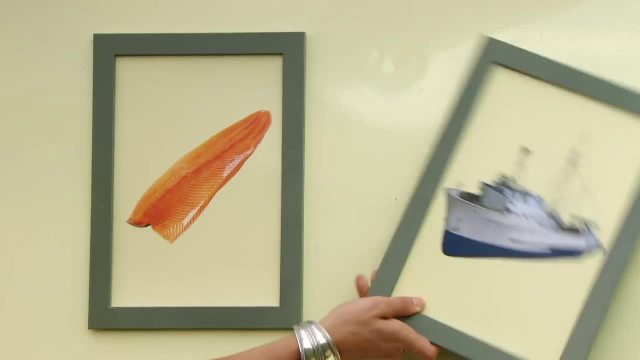 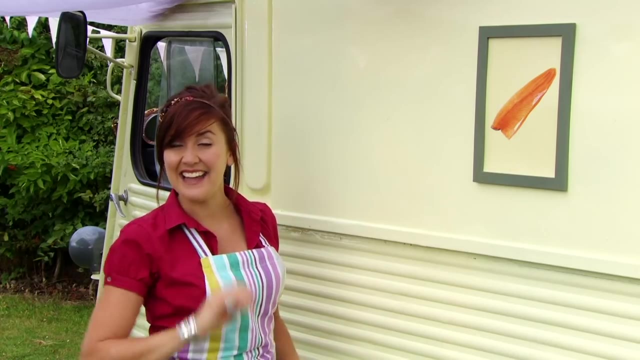 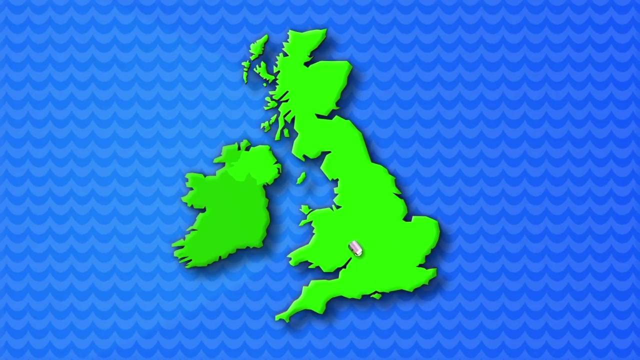 but it's definitely not a type of fish, so we can take that one away too, I think, Which leaves us with trout. We're going to need some trout in our seaside bites, and I went to find some MUSIC PLAYS. I've come to Guildford in Surrey to find some fish. 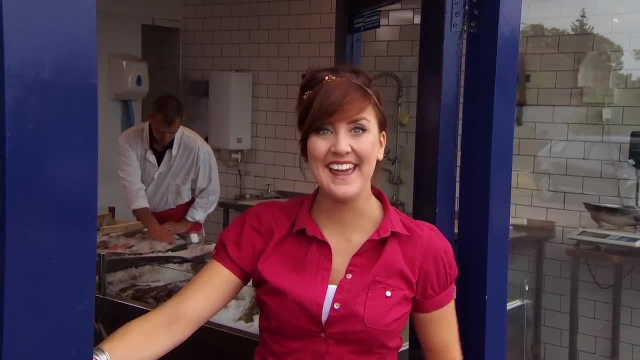 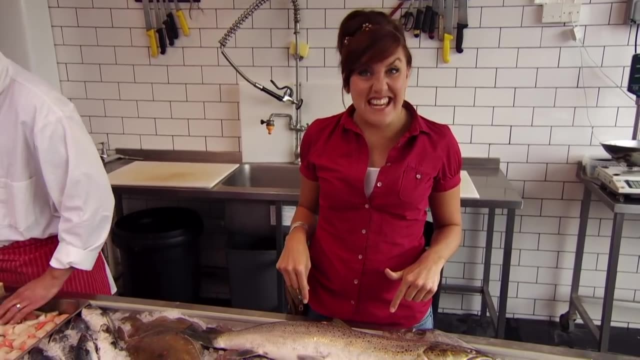 and I think I'm definitely going to find some in here. We could use lots of different types of fish for our seaside bites, but we're going to use sea trout and this is what a sea trout fillet looks like And look, it's a really nice orangey-pinky colour. 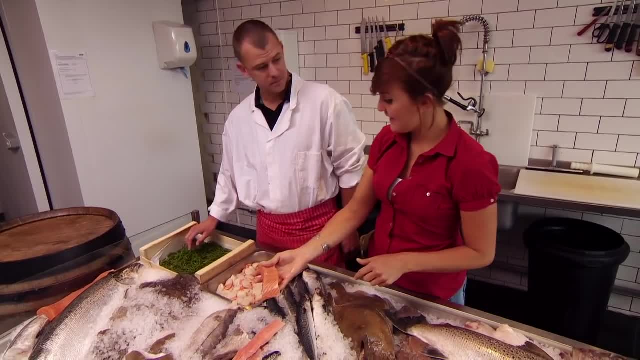 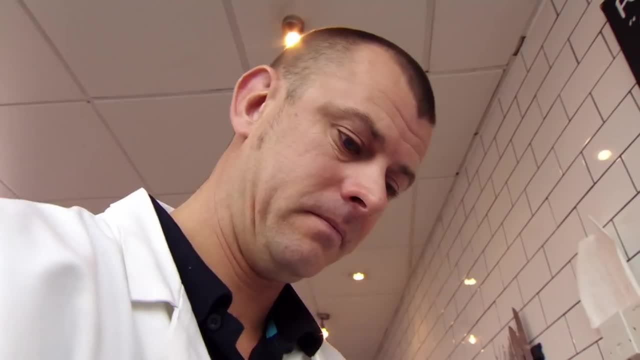 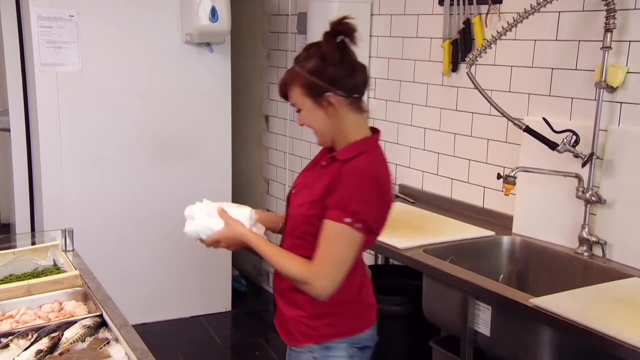 All I need to do now is get this fillet wrapped up. Please, can I have this wrapped up, Duncan? Of course, There you go, Katie. Thanks, Duncan. Can't wait to use this in our seaside bites. That was really interesting, wasn't it. 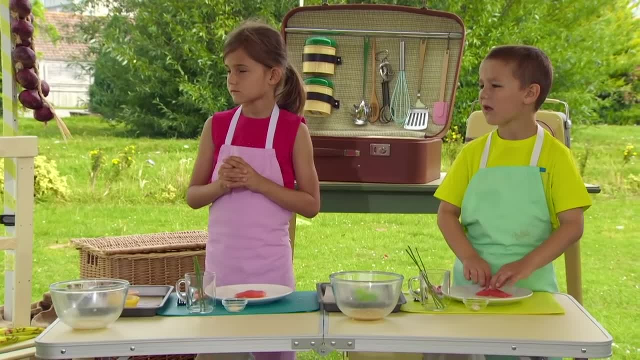 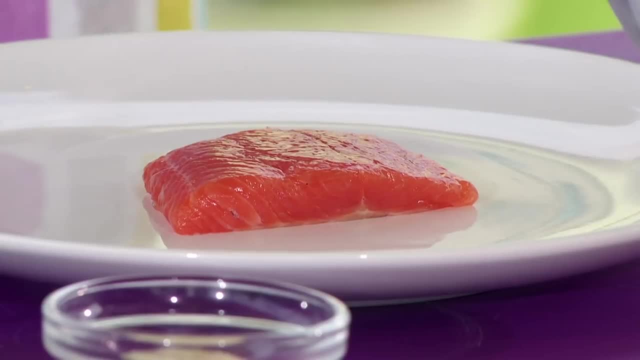 Well, I've got our trout here now and we're going to use it in our recipe. Now it's really important everyone, when you're cooking with fish, to make sure that there are no bones in it. So I've already checked the trout for you. 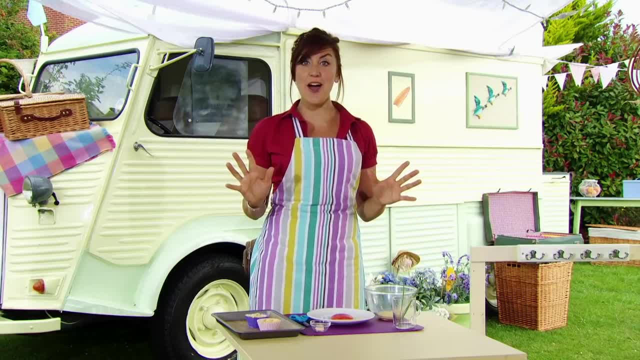 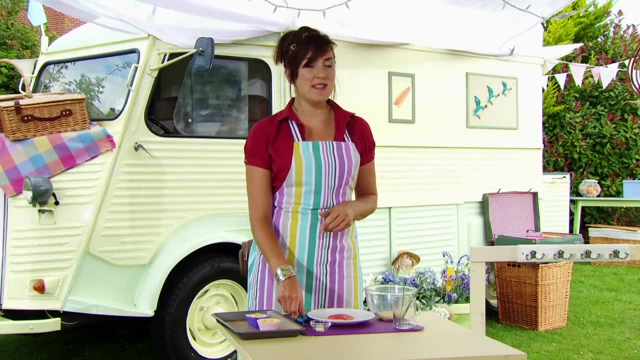 to make sure that there are no bones. So we're ready to go. So the first thing we need to do with our trout is snip it up, and to do that we're going to use some scissors. But remember, be safe with scissors. 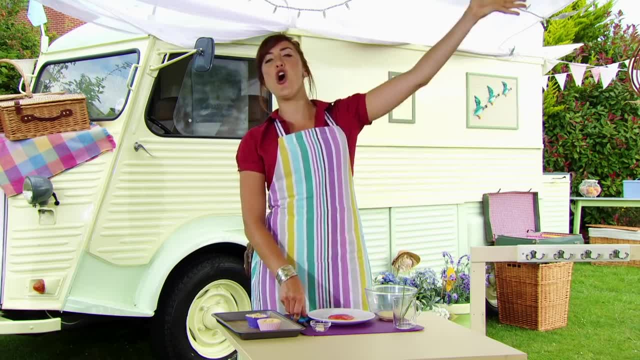 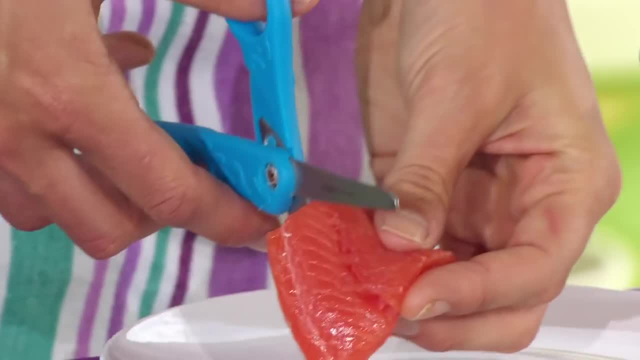 Everybody knows that you point them down towards your Toes. Toes, You've got it OK, so take your trout and then use your scissors to snip it up, and we want to snip them into bite-sized pieces about this big. 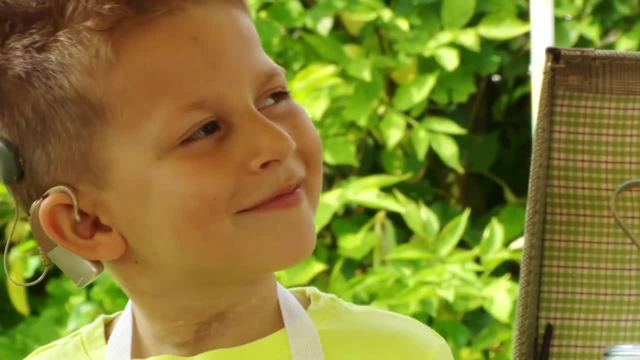 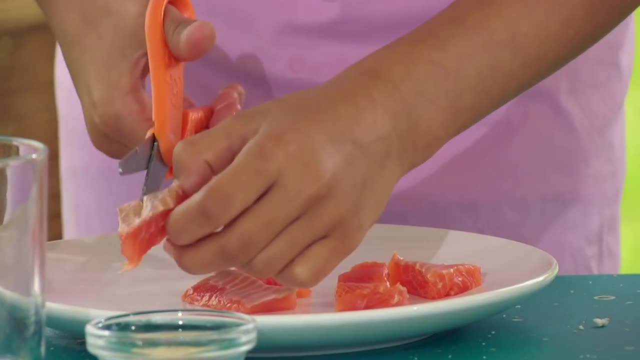 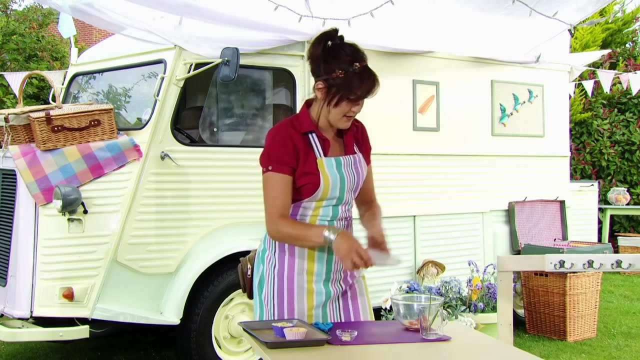 Ah, That's it. OK, let's get snipping. everybody See. And when you've snipped your fish, you can just put it into your bowl with the eggy mixture that's been left over. OK, let's put our plates over here. 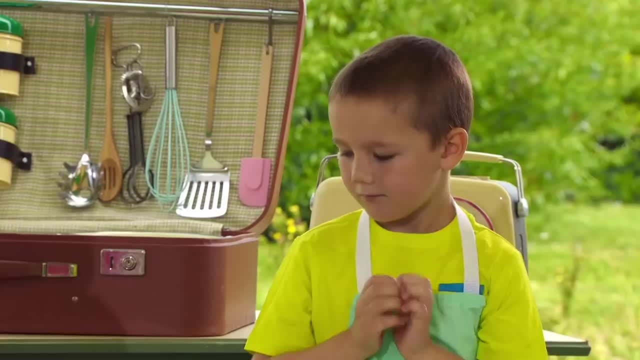 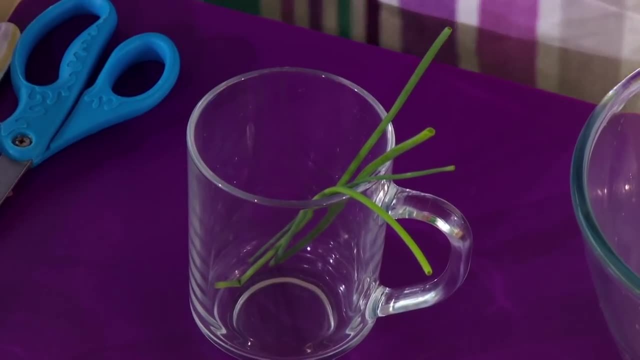 because we don't need those any more, And we'll give our hands a quick wipe as well, because we've been touching fish. The next thing we're going to use are these, And they are herb called Chives, And they come from the family of onions. 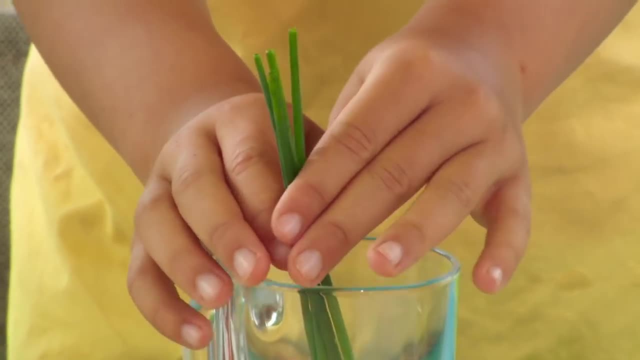 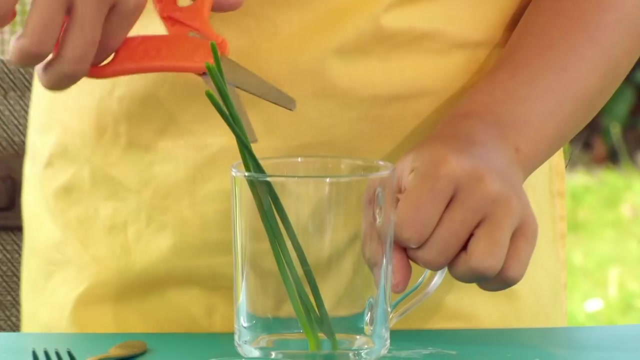 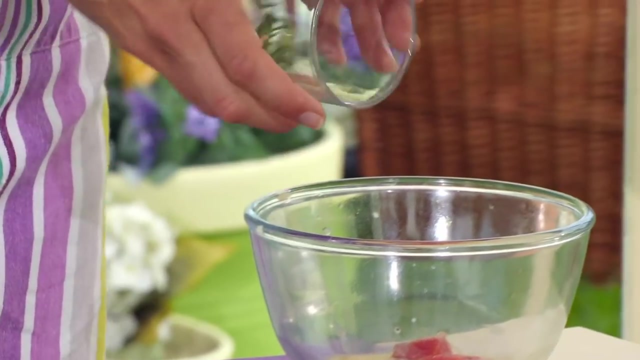 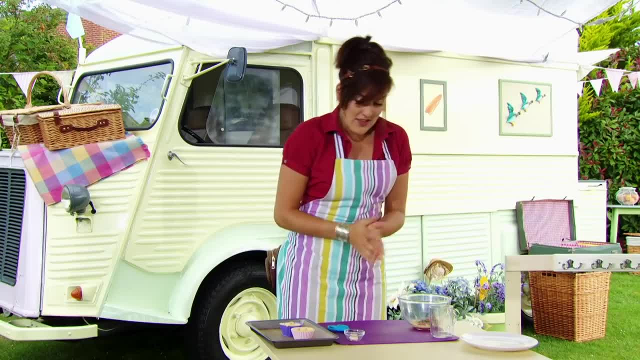 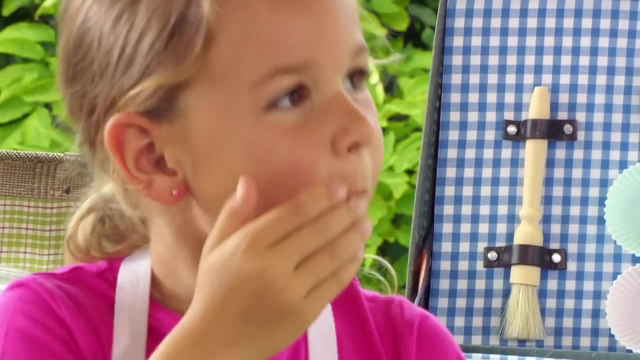 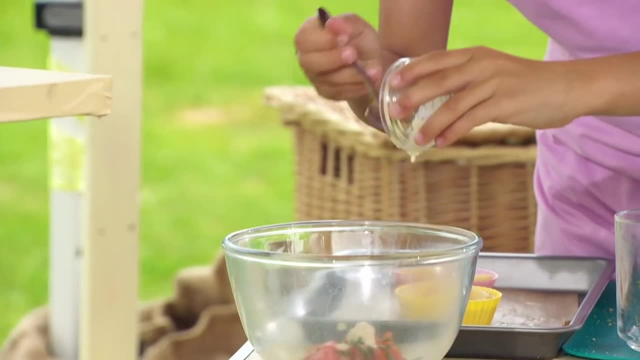 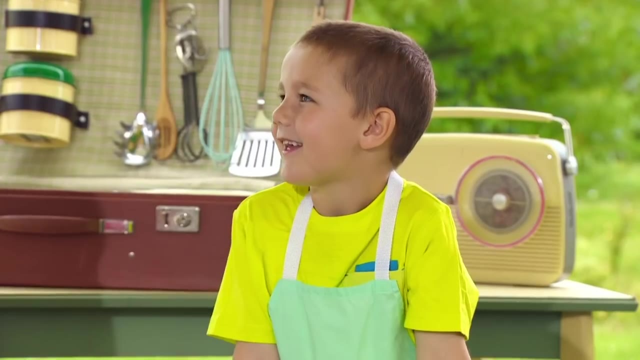 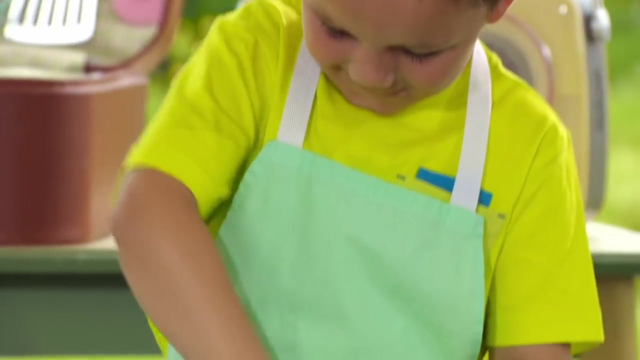 So let's just tap that out There we go, Out you go, And when you've got your horseradish in your bowl, we're going to give it a big Mix. OK, off you go. Yeah, Don't forget, we need you to join in with us as well. 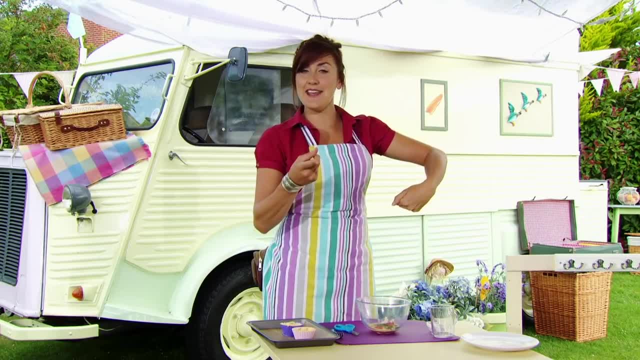 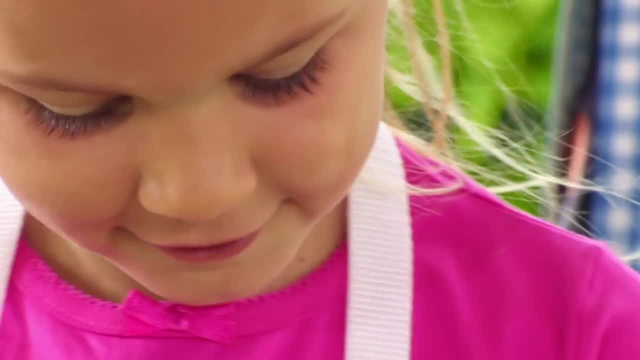 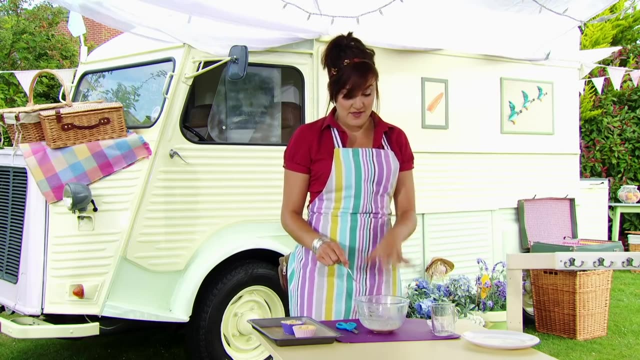 Get your bowl. Get your bowl like this, And then get your fork like this and go mix, mix, mix. It looks very yummy. I think it's going to taste even more yummy, Amber, Great. And the last thing we need to do is put this mixture. 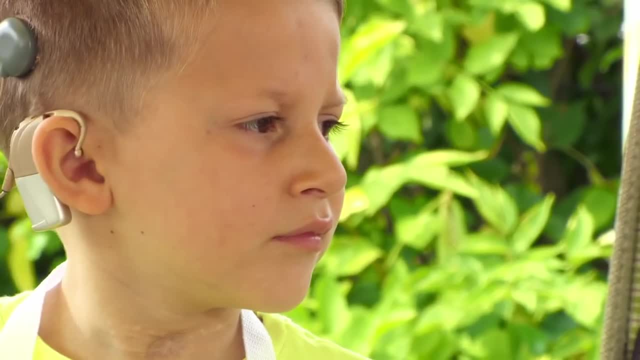 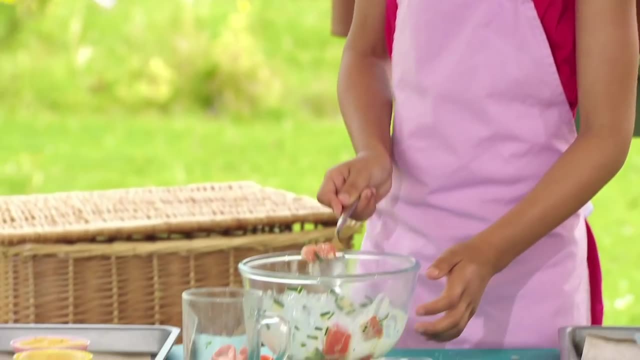 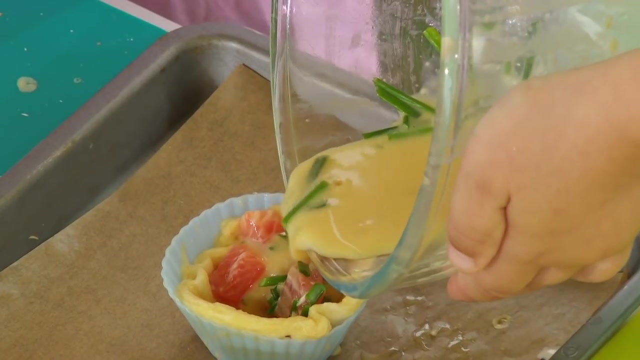 into our muffin cases with our eggy bread. So let's use our fork to scoop out the fish- I'm going to put a little bit in here- And then all we need to do is pour the rest of this mixture into the muffin cases. 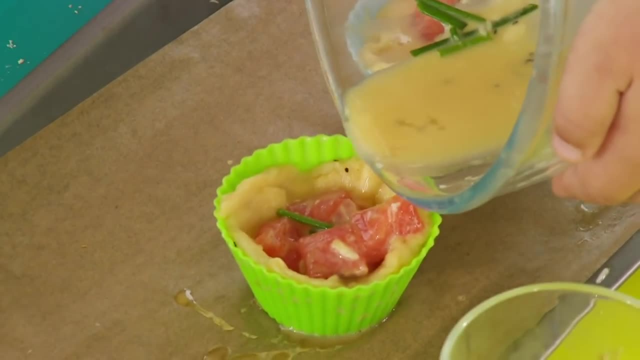 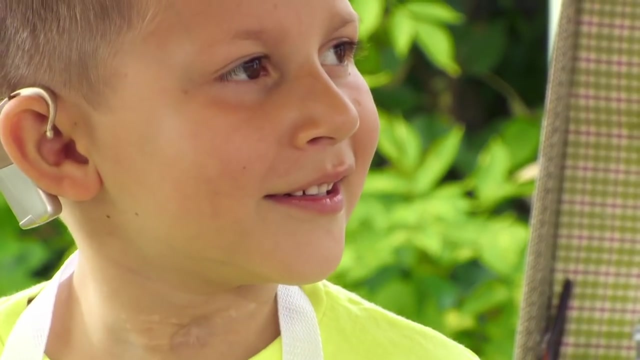 That's it, Ryan. Good job, What a great chef. And that is it. You made it. You put all the ingredients together for your seaside bites and you did it all by yourself. Well done, And now I need to put them in the oven. 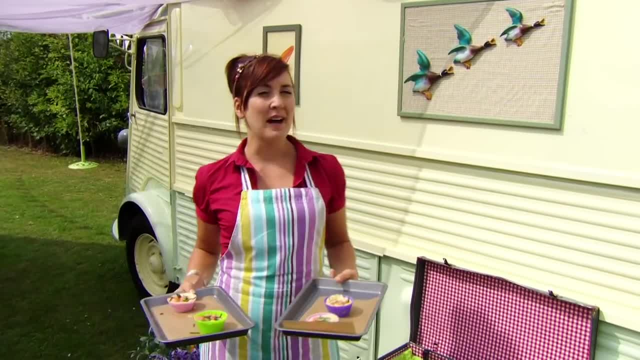 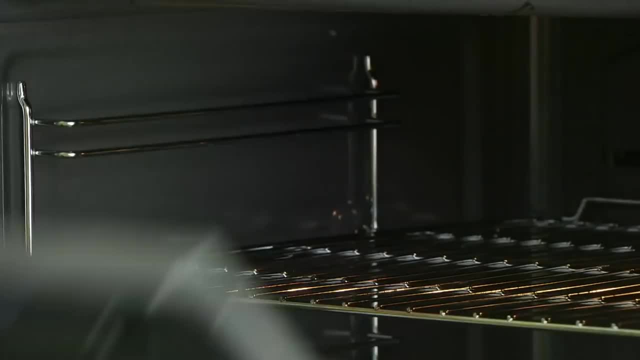 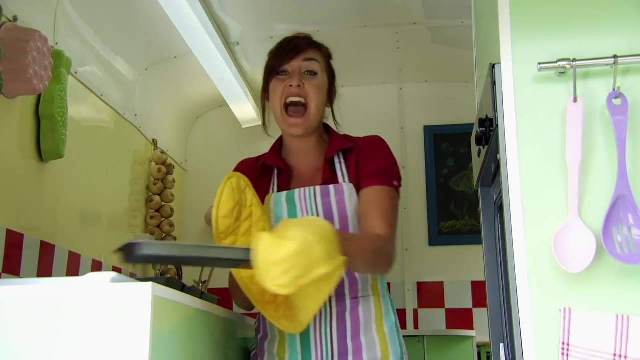 But remember, ovens are hot, so don't go near. Ask a grown-up to help you here. Now we've cooked with you and had lots of fun. Let's tidy up and think of all the things that we have done. There was. 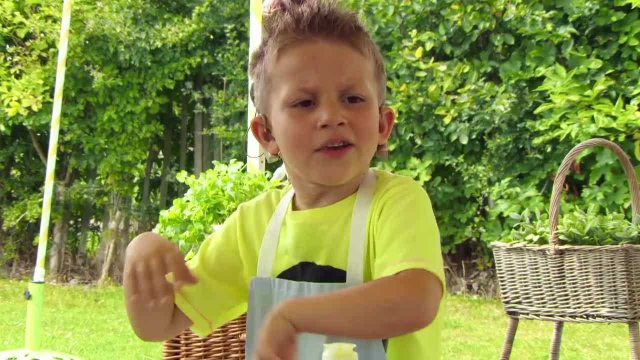 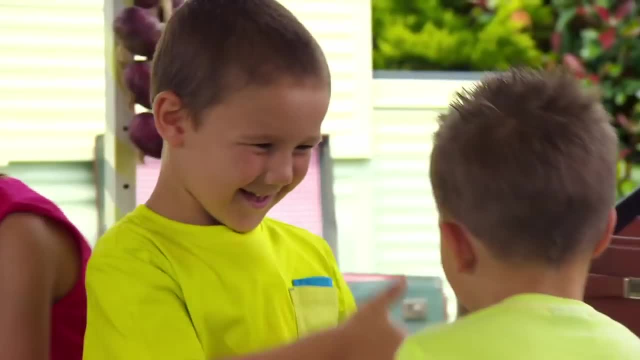 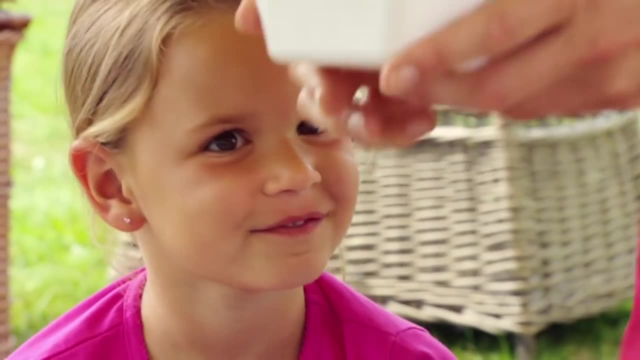 Cracking Nothing, Pouring, Mixing And clearing any mess and putting things away is always fun to do at the end of the day. And here they are- everyone your very own seaside bites, And they're all cooked. Let's have a look at yours, Ryan. 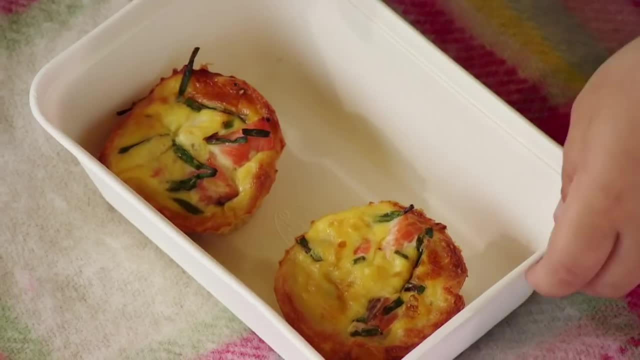 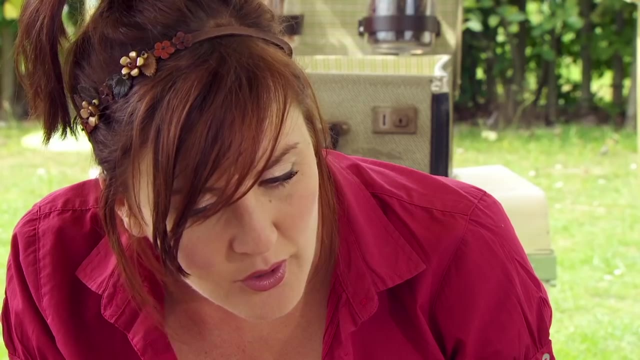 Wow, Hey Ryan, how have they changed in the oven? It's mostly at the top. What the fish? It's all poking out at the top, isn't it Say hello, Hello, Hello, Hello. Okay, Amber, let's have a look at yours. 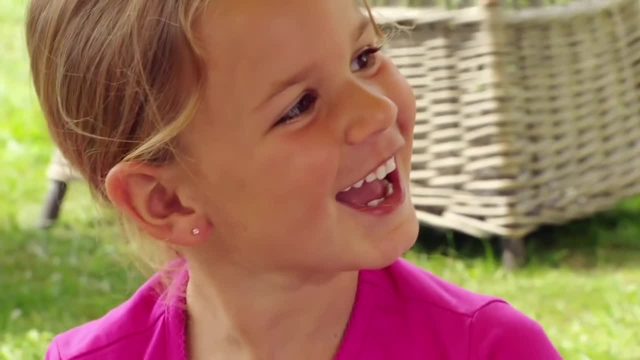 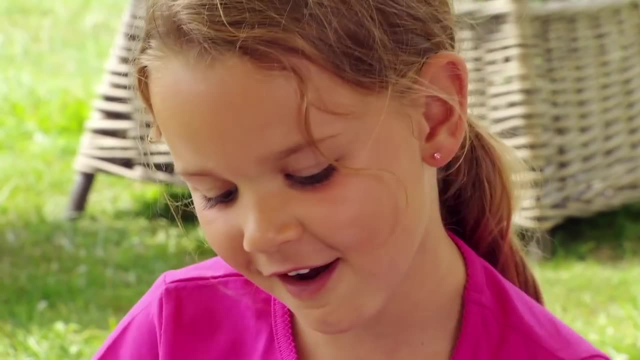 Hey, look at that, It's all cooked. It's all cooked. Hey, that looks fantastic. Are you pleased? And what has changed about your seaside? bites Different colour and it's got higher. Okay, let's put the lids on top and we'll save these for later on. 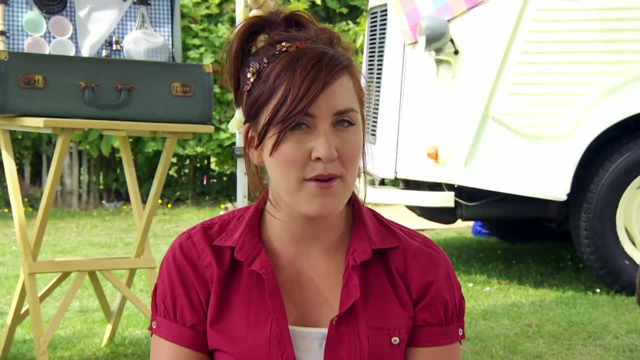 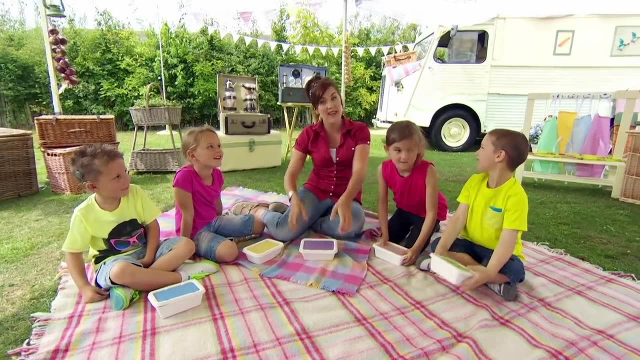 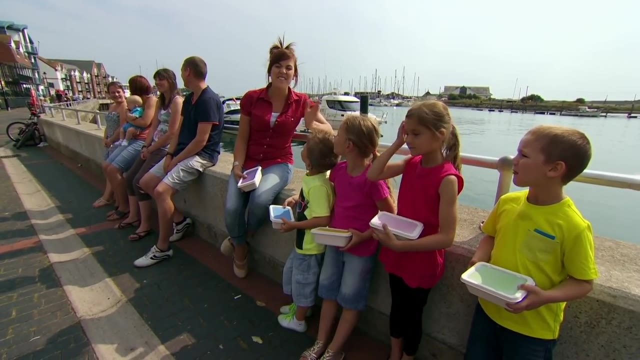 We've travelled to you, we've cooked and had fun. Now let's have a party with everyone. Yeah, Come on, you can come with us, Follow me. Well, we're at the harbour and we've got our food to share with everybody. 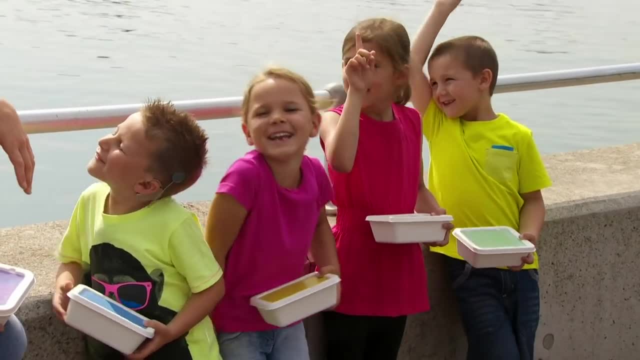 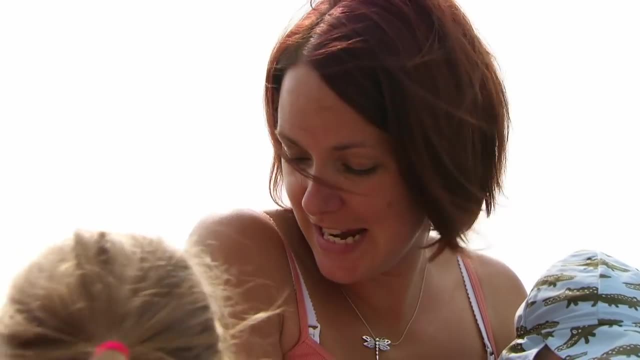 Hey, who's hungry? Me Me. Come on, let's share it with everyone. I made these myself. Would you like one? Oh, yes, please, Mmm, that's nice, Mmm, That's nice, That's nice. 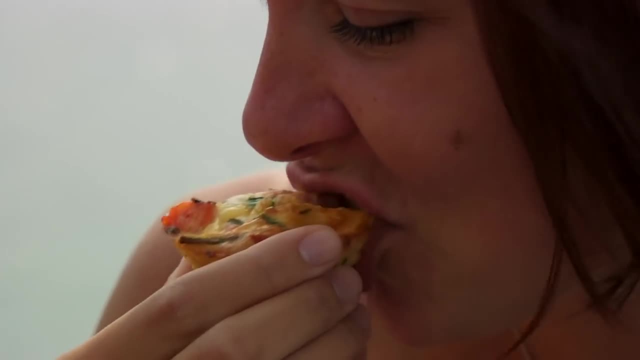 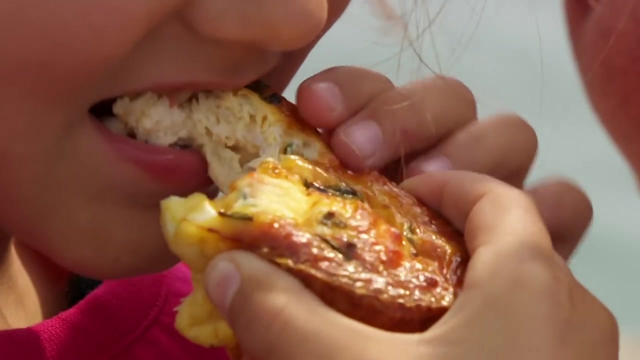 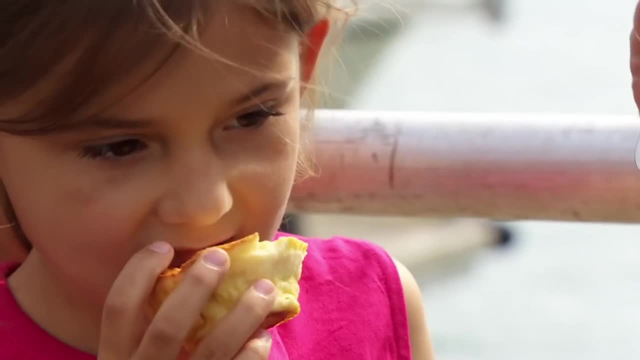 Yummy, Yummy. Can you taste the chives in it? Mmm, me too, Mmm, They are lovely. So what did you enjoy the most? I like eating, You like eating it. Oh, it's very yummy, isn't it?